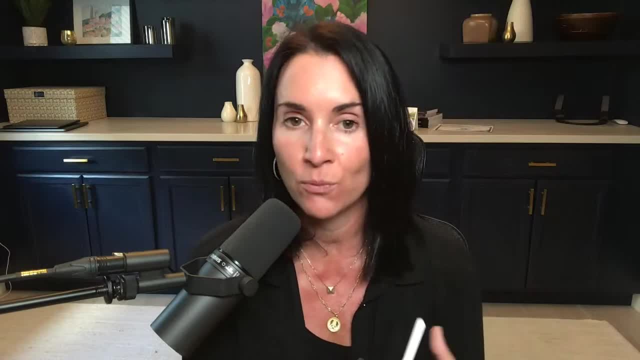 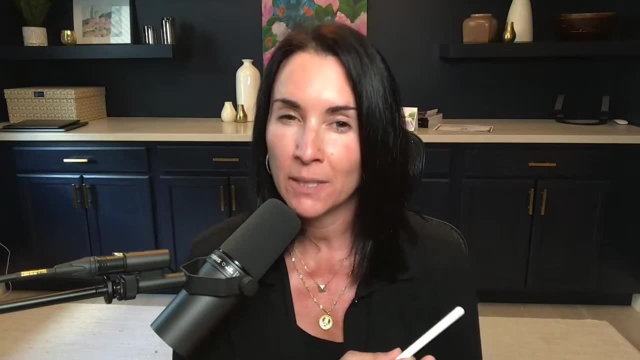 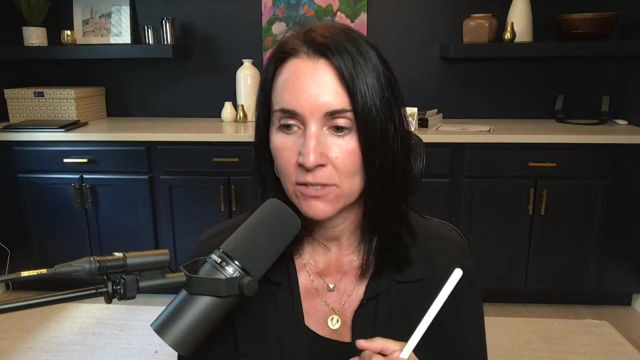 thing, no worries, When I am done, it will be available for replay And if you sign up through the form that you did, you will get a follow-up email in about an hour after the webinar is over and you will get all the information and all of that. So, if something happens, 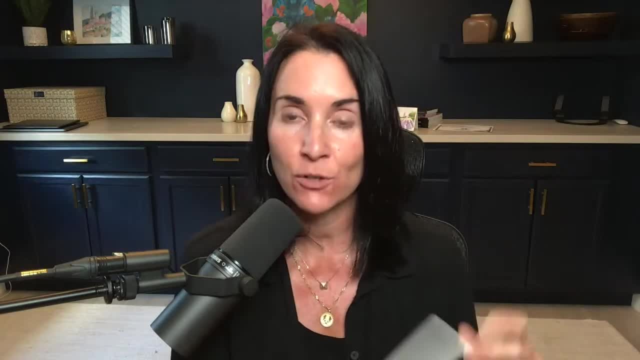 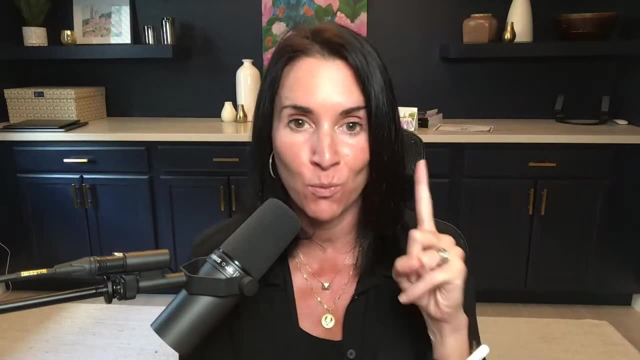 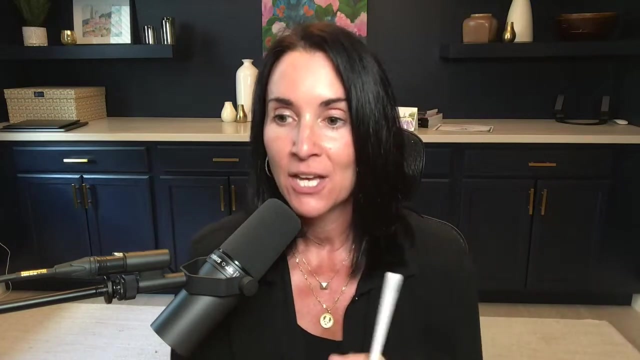 don't worry about it, No big deal. You will be able to get this Now if you're watching live on Facebook or YouTube. I can't respond to you yet because I've got like 40 things going on here And you know I'm a one-woman show currently, So I have to prioritize. Okay, So I'm so glad. 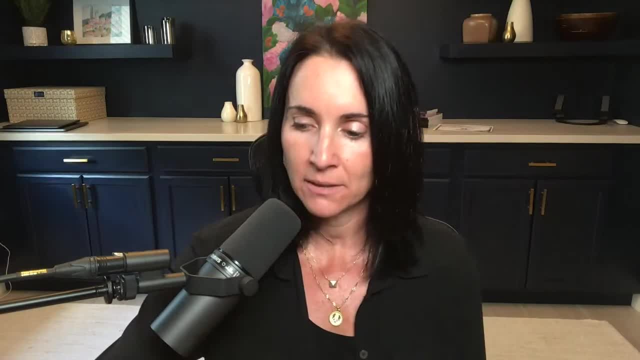 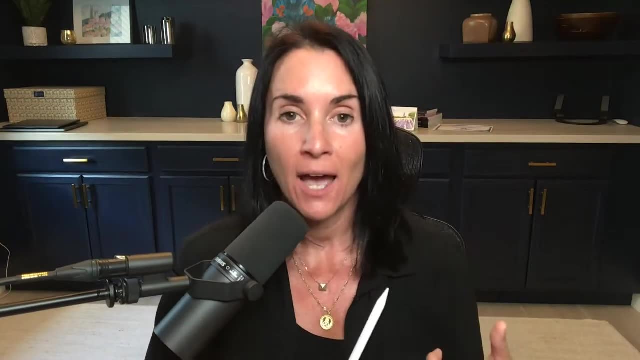 all of you are in the chat. I think my mic is a little loud. Let's turn that down a little bit. There we go. Sounds a little bit better there, And okay, Think about the chat. When I'm listening, it's hard for me to kind of chat and present. So what I'll do is I'll stop after each. 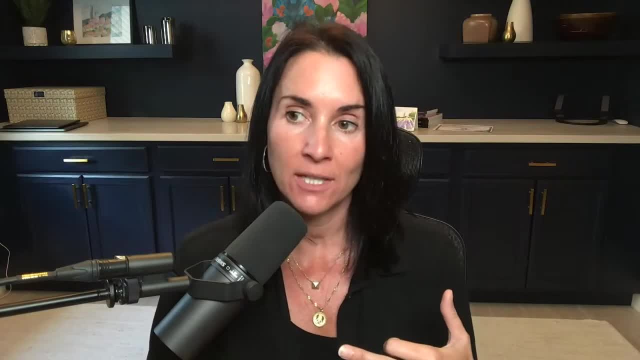 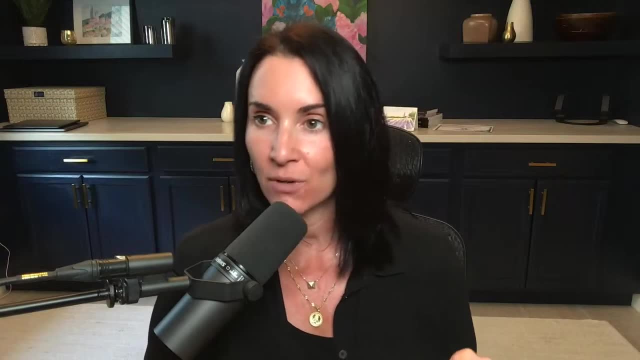 section and take questions and you can put it in the chat if you're in the live webinar and I will do my best to get to everyone. We do have a lot of people in the webinar: over 800 people signed up and we have right now about 65 live, So that's a lot of people talking and I will do my best to. 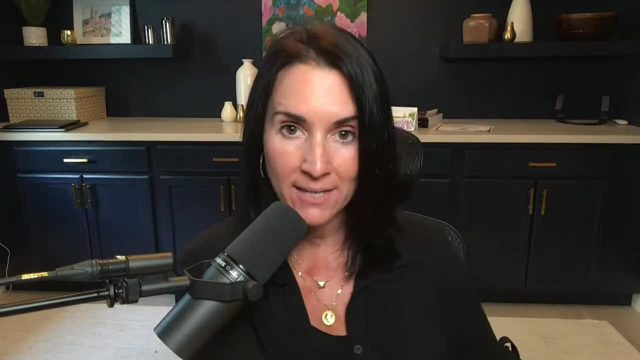 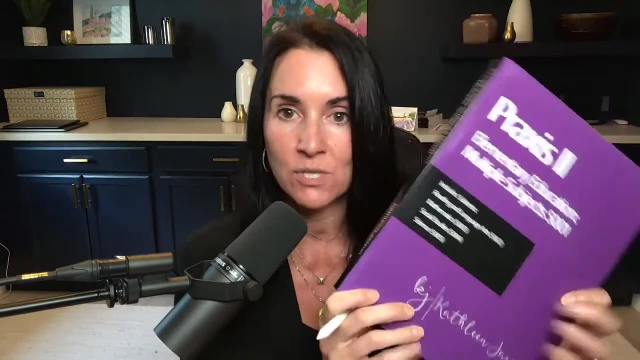 get to all the questions. All right Now, really quickly. this webinar is for the Praxis 5001.. That's the Elementary Education Multiple Subjects Test. I have a book for this and I will be using problems from this book If you downloaded. 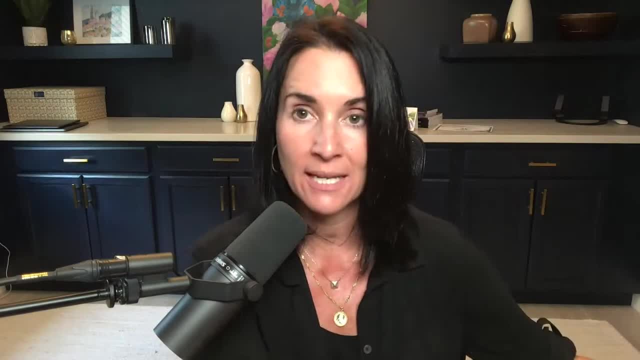 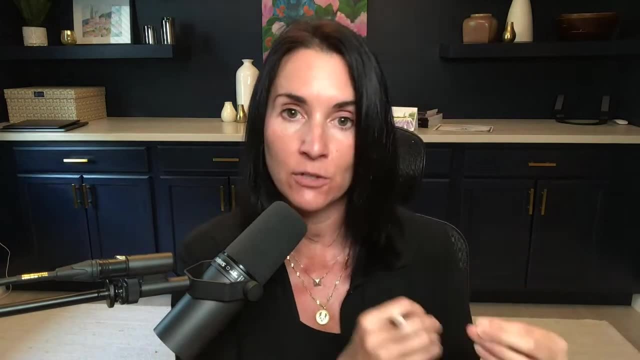 the study guide you have the exact questions I'm going to be using in this webinar, So don't worry if you're like where's the presentation, your book, the study guide. the little free study guide that you downloaded with this is that I just blew it up So it looked a little bit better for 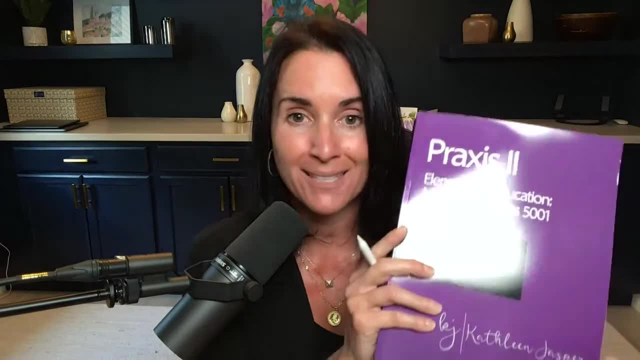 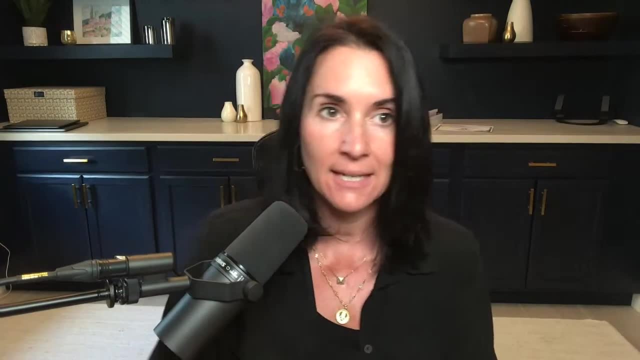 the viewing public. Okay, So this is the purple book. Now, keep in mind, this is 500 pages, Okay, And today we're going to just do a snippet of that, All right, So if you're interested in getting the book really quick and we'll get into the webinar, 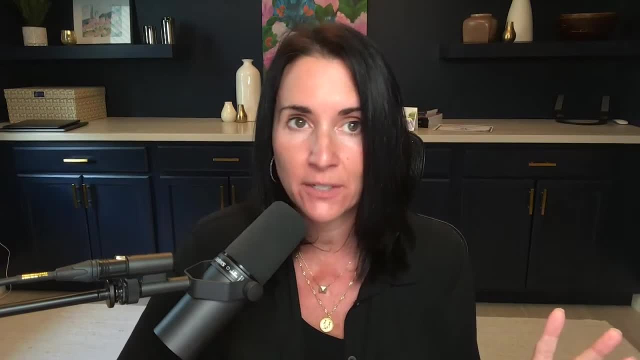 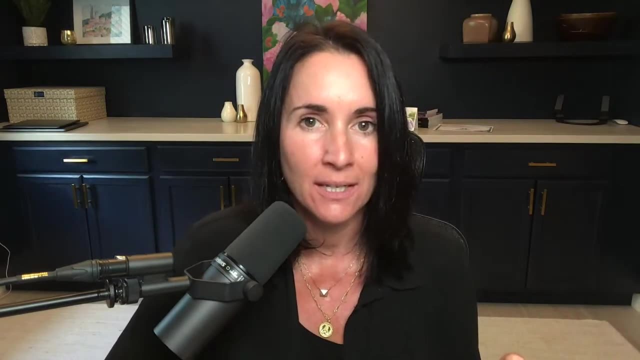 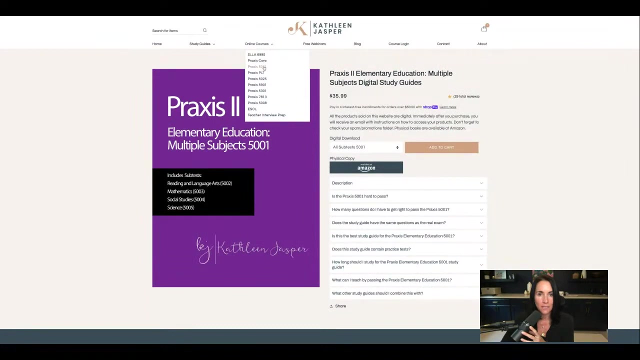 you can get it on my website here. There's also a button here to get it on Amazon and you can. oh, I need to share screen. Please hold Sharing screen. Here we go, Okay, So you can see that this is where you get the book. You can also get the online course here. The online course comes. 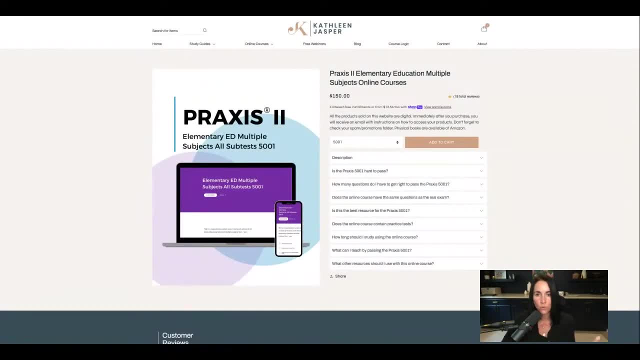 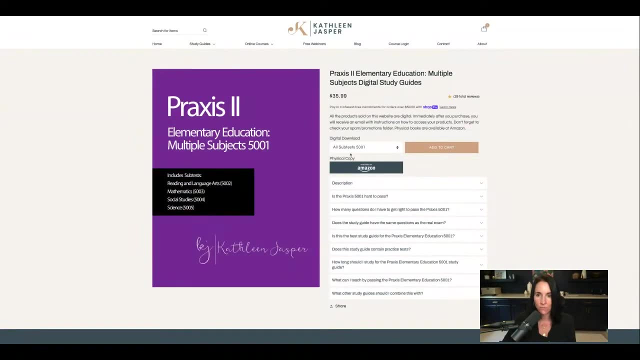 with the book and you can buy individual sections. So if you pass one or more sections and you don't have one, you can buy individual sections. You can do that also in the study guide. So if you only need the math or you only need the reading and language arts, you can do that here. The physical 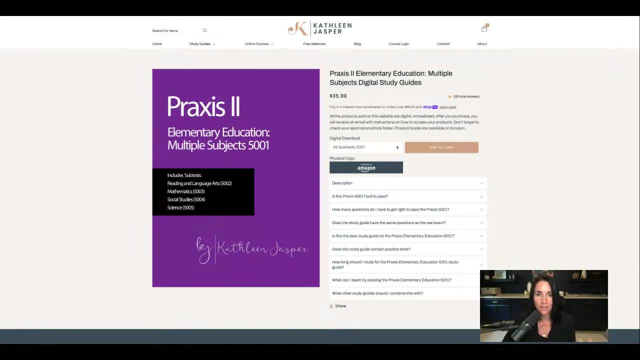 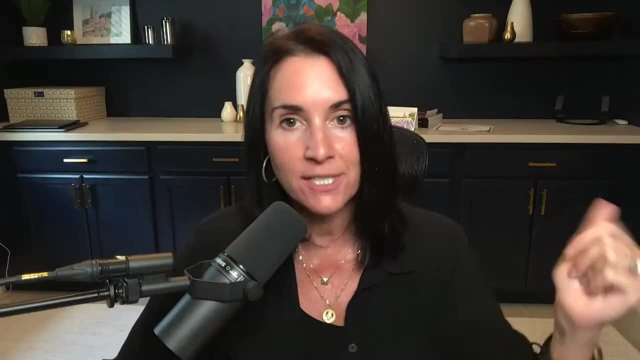 study guide. you just click this little Amazon button. It'll take you here and you can see we have over 600 five-star ratings for this book, So it definitely works. But if you're, um, if you are trying to save money and you just want to do the free stuff, totally the free stuff works. I have. 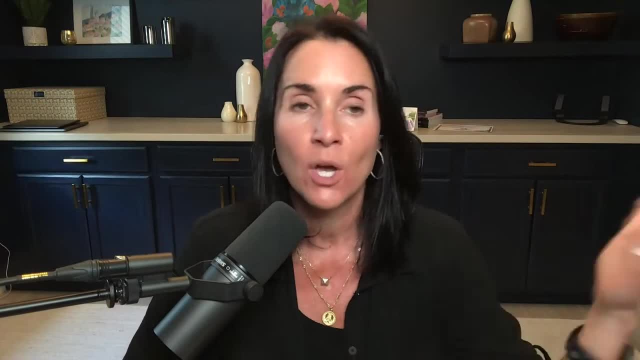 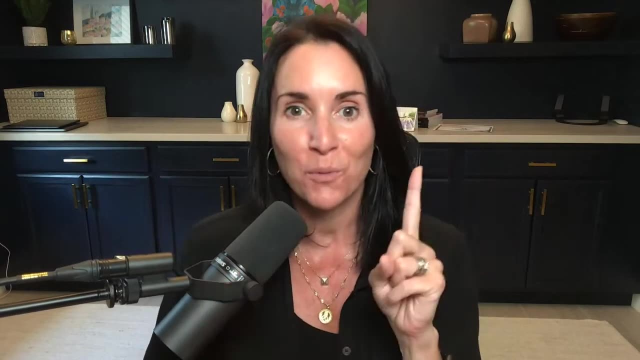 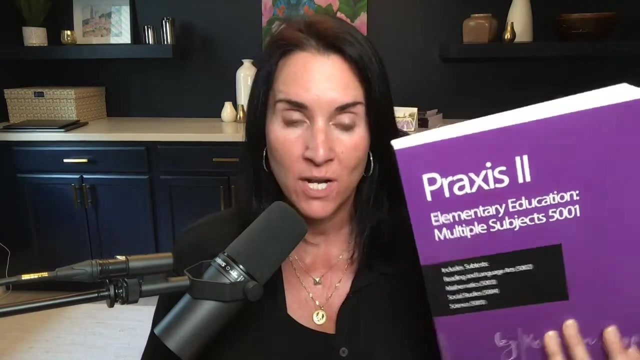 a YouTube channel with all kinds of stuff in it that will help you as well. So we have lots of books. You can pass your exams Okay. So no worries, I want to jump right into it now. Oh, one more thing. If you're taking the 5 9 0 1 test, that is the exact same test as the 5 0 0 1,. 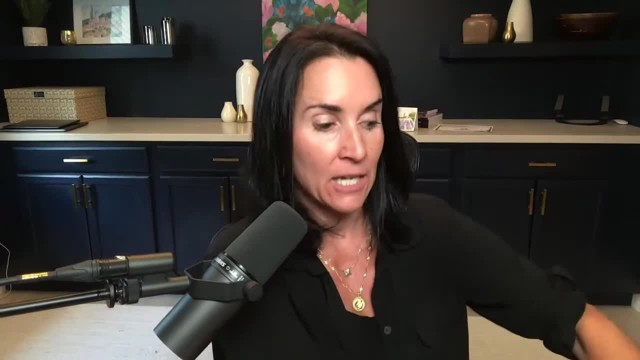 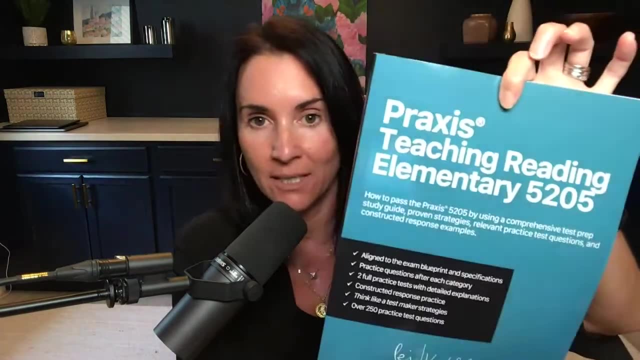 but it just doesn't have the English language arts and reading And you guys have to take, instead of the language arts and reading in the in the test, you have to take a separate reading exam And I have a book for that. So, anyway, I have books for a lot of things And I 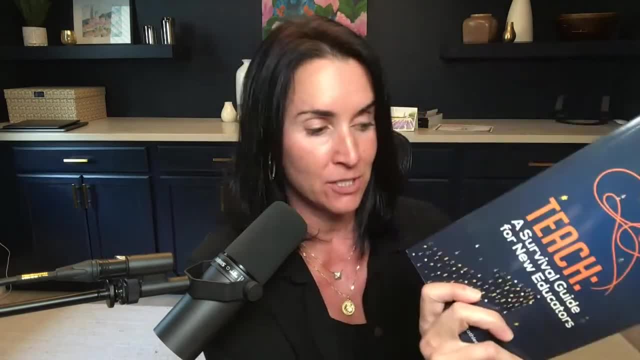 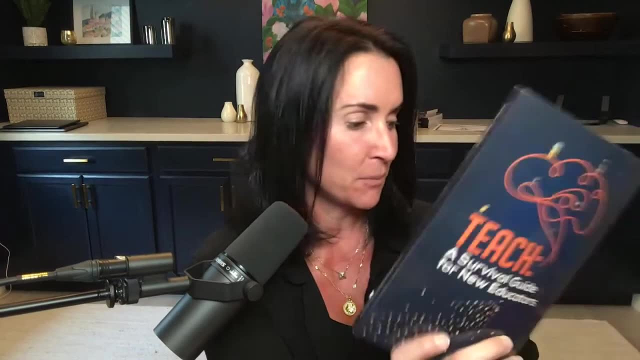 teach how to teach. I just published it. I published it in the middle of the year. Some of you may not be ready for it until August, but I do have this book teach- a survival guide for new educators. A lot of people like it and I'm really proud of it. So if you get on Amazon, 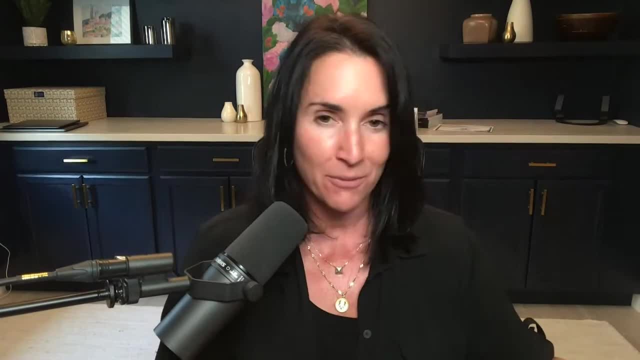 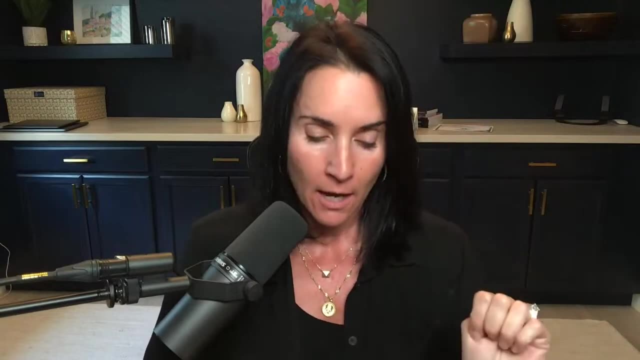 go ahead and check that out. It comes on Kindle as well. All right, enough about my products, Let's get in. So we're talking 5 0 0 1 today. big test for subtests, Um you. 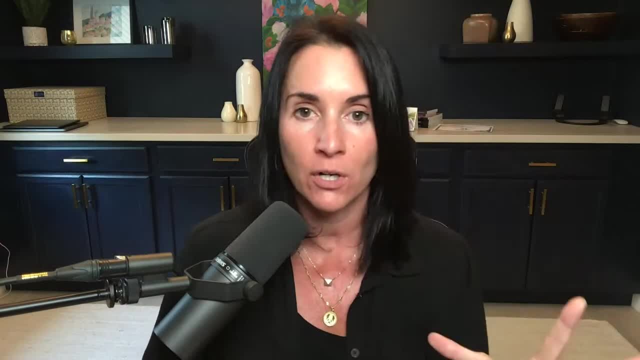 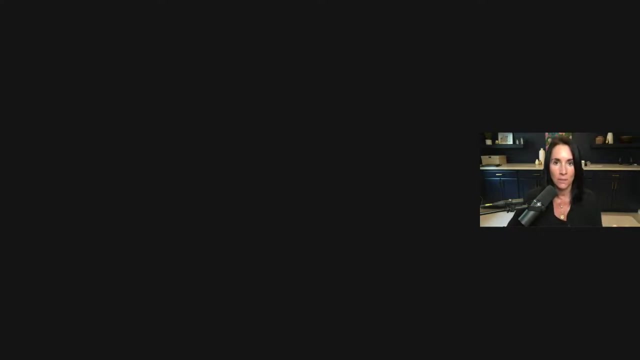 it is scored separately. I'm going to go through an overarching idea of the test recommendations and then I'm going to get into some practice problems. Okay, So let me just go here really quick and I'm going to share my screen. All right, let's go here And I'm just 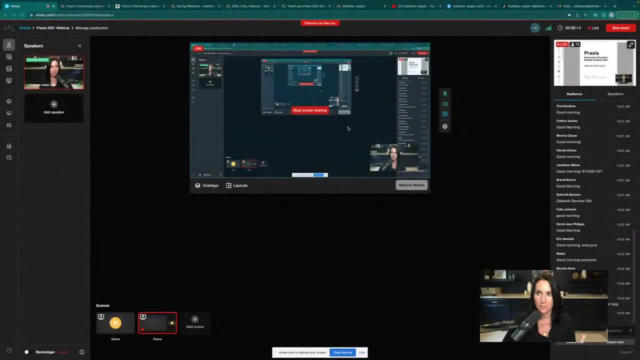 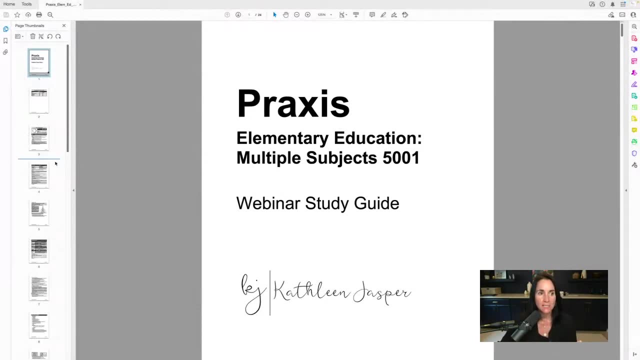 gonna talk really quickly. Can you guys see? Yeah, you can. Okay, You can see this. So this is the study guide you got when you signed up for the webinar. It's got tons of information in it. This is just a snippet of the big study. 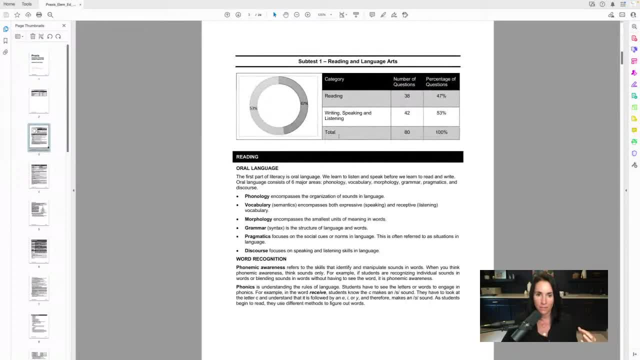 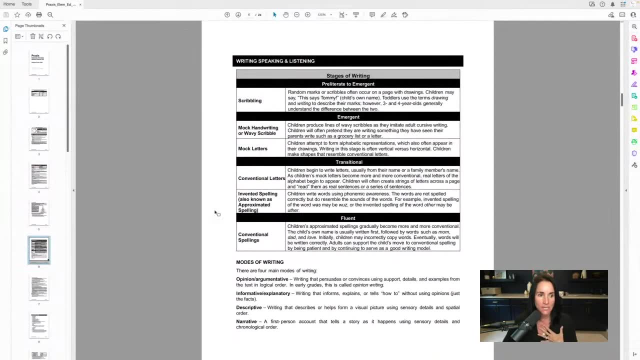 Guide, but you can see that I have broken up the blueprints here and under the reading section. I have a lot of information here because the reading section, in my opinion, is one of the hardest sections. Some of you may agree with that or whatever. but and then past that, 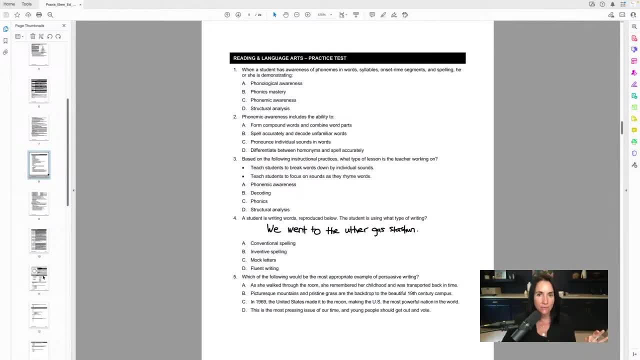 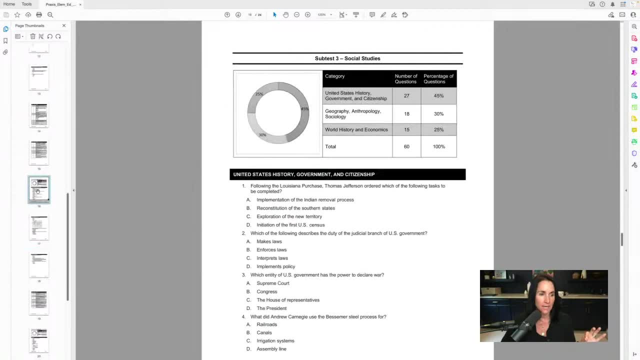 I have practice problems for each individual section. Then I have the blueprint for the math. Then I have practice problems, you know, for the math. Then I have the blueprint for the social studies, Then I have some practice problems for the social studies And then I have the blueprint. 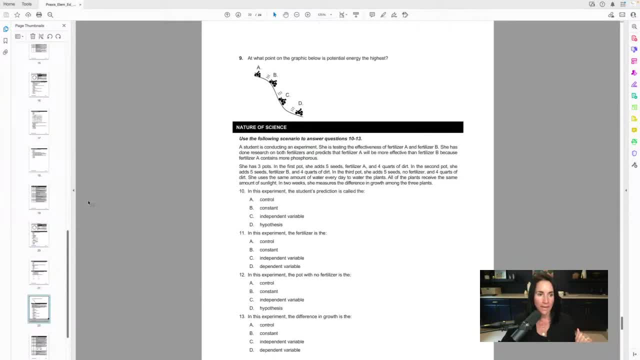 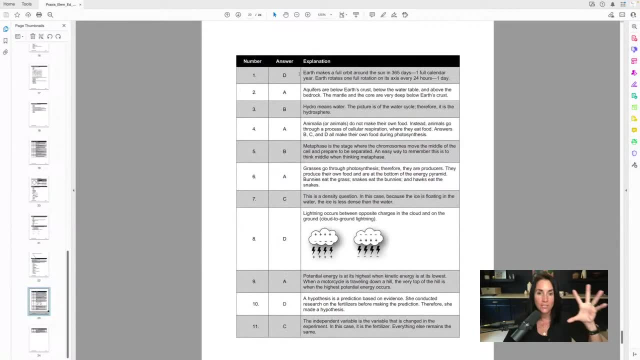 for the science section And then again practice problems for that. Now understand too that these answer explanations are very important, And that goes with the book as well. Don't skip the answer explanations. There's a lot of good information here. They're almost like their own chapter, So 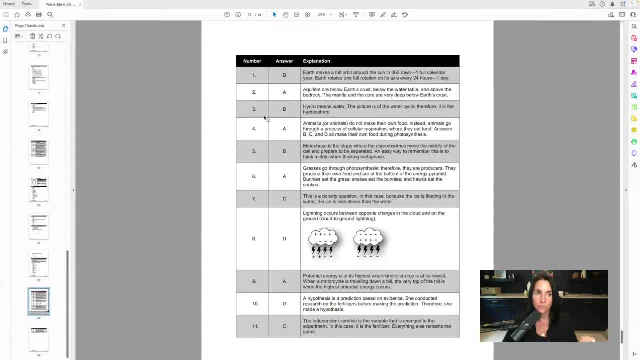 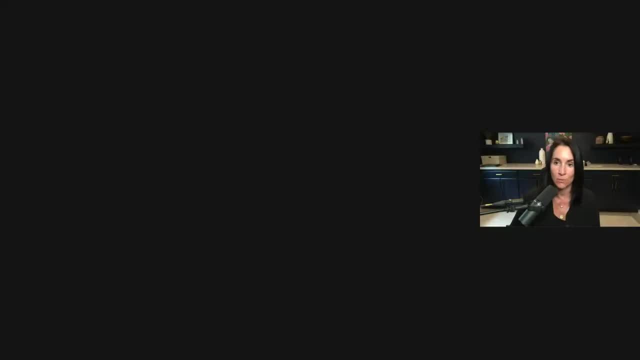 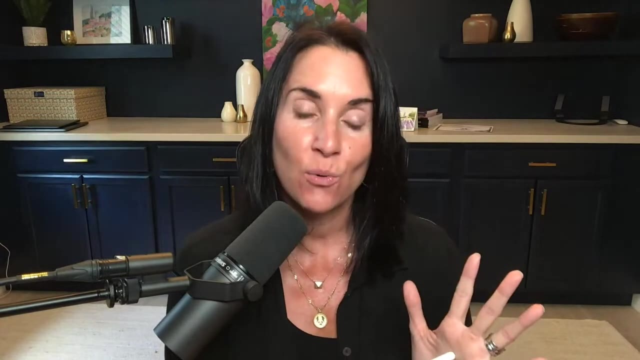 if you're in the free study guide or paid study guide, definitely read those answer explanations, All right, So that's going to be really, really important. And let me just tell you one more thing, One more tip of advice for you here. So a lot of people want to just do practice tests over and 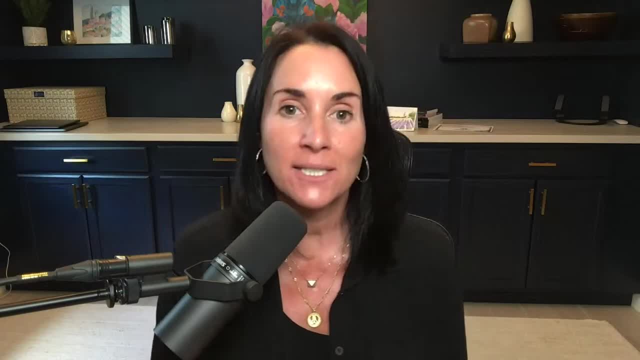 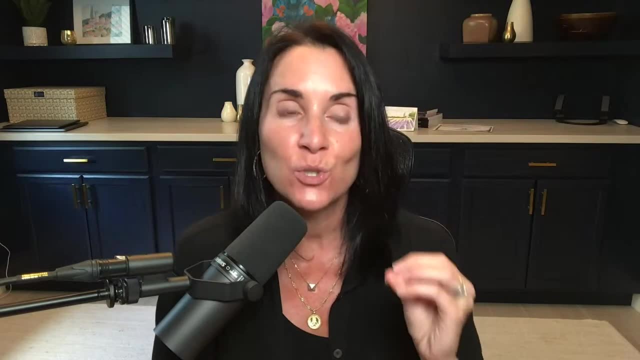 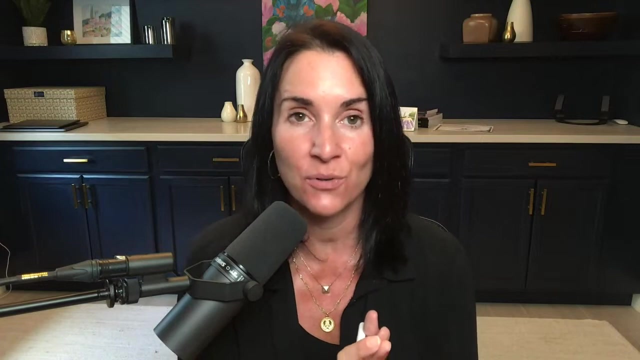 over and over again to get this information, And practice tests are a really good tool to assess your skills, But this test is huge and has tons of information, And so you really have to understand the concepts. So I'm begging you- I keep doing videos on this. Please stop doing practice tests. 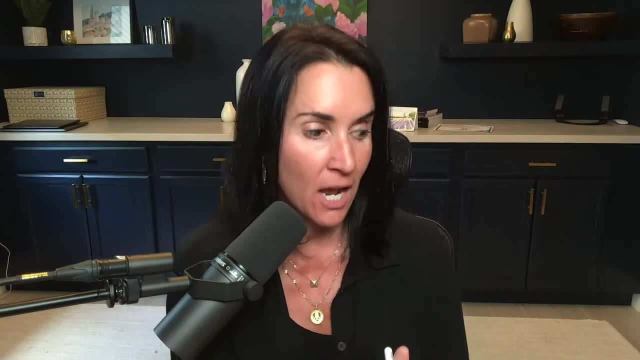 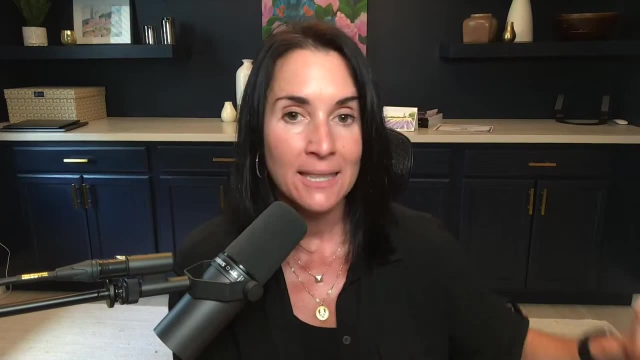 over and over again, expecting to pass the test. If you're having a hard time, you have to understand the information. That's why I have online courses, YouTube videos that explain these concepts. Okay, This book: look how big it is. All right, It's full of information that's important for you to. 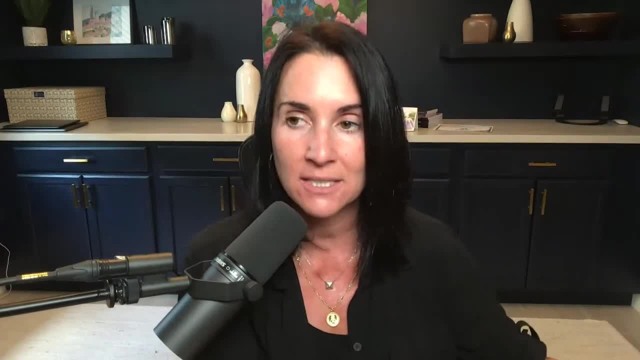 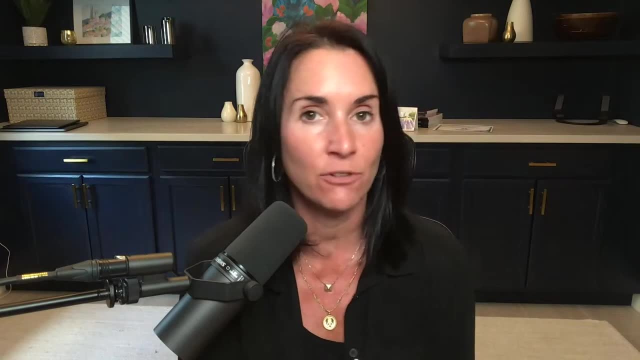 know The practice tests are awesome. I know everybody likes to do a practice test to see where they are, But you don't know what questions you're going to get on test day, So relying solely on practice tests for you to understand this information is not going to work. So really got. 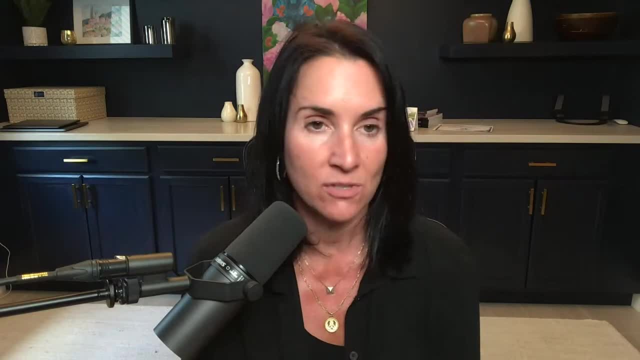 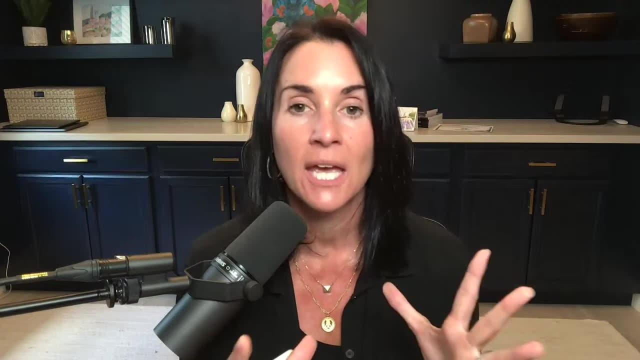 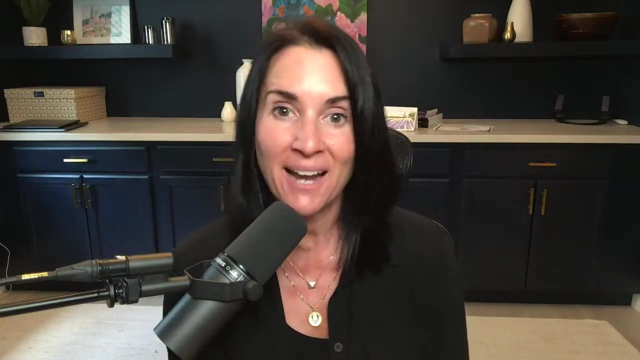 to dig in. You got to understand the fundamentals of reading, the fundamentals of math, important science and social studies concepts, And really get to know those content categories and test specifications in order to pass this exam. Okay, So, just like your students, if your students didn't pass a test, you wouldn't say take another. 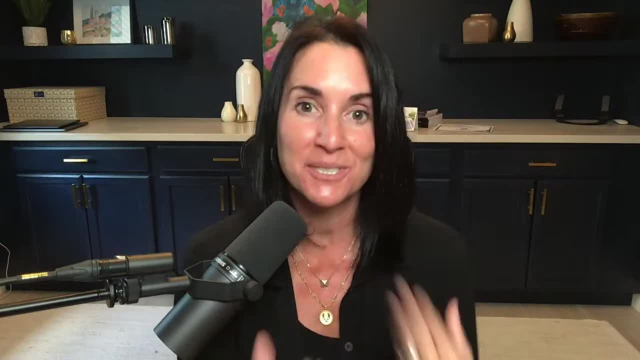 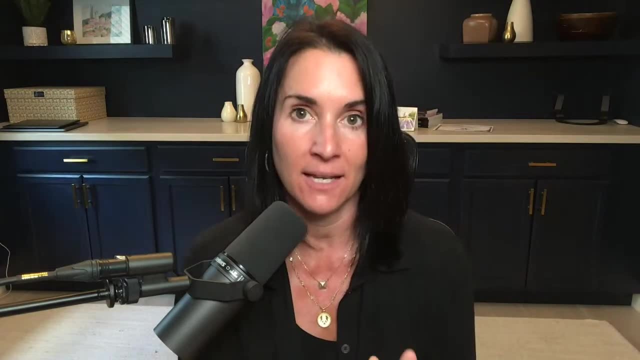 practice test. take another practice test. take another practice test. You would stop and work on the skills that the students were missing. So do that for yourself as well, because this is a big test and it can be difficult. Now the other thing is if you pass one or more sections of this. 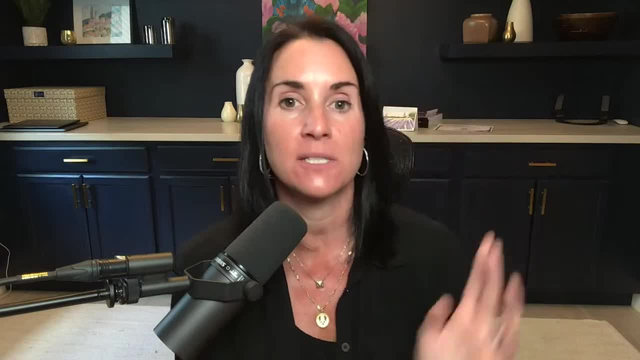 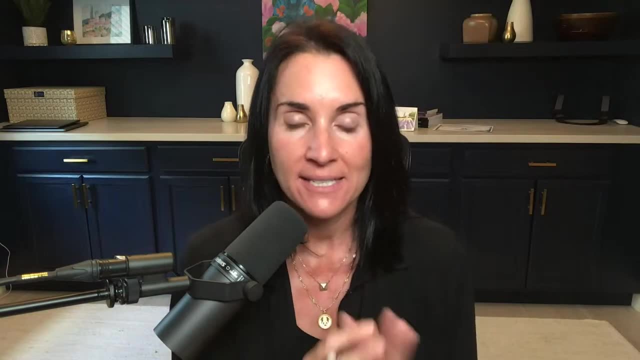 test. that's a victory and you should celebrate. Some people get upset because they don't pass all four at once. It's a huge exam. If you pass any of them, that is fantastic. And remember: you can take this test as many times as you need to. I know it's expensive, It's not. 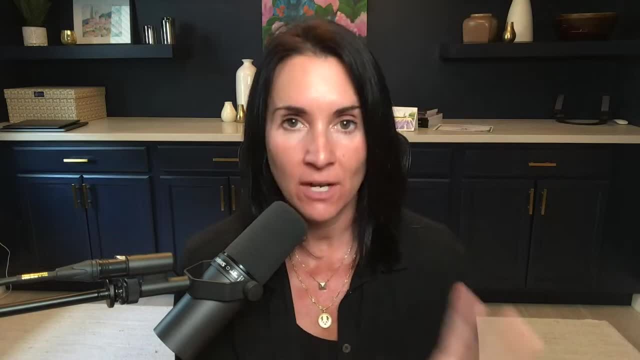 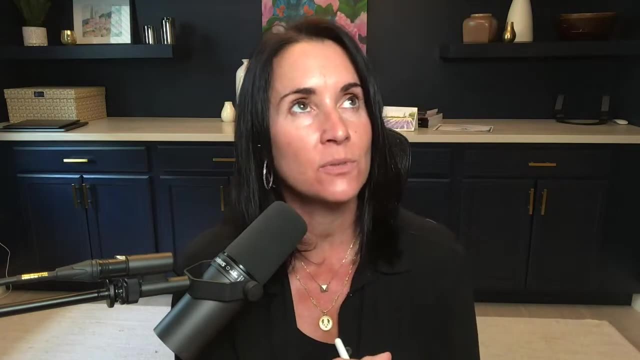 ideal, but just take the pressure off yourself a little bit and understand that it's okay. So just understand that. And then the next thing: what else was I going to tell you? It'll probably come to me in the middle of the presentation. All right, Let me run over to the chat. really, 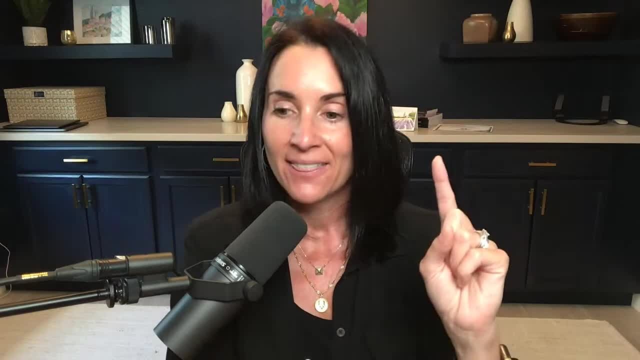 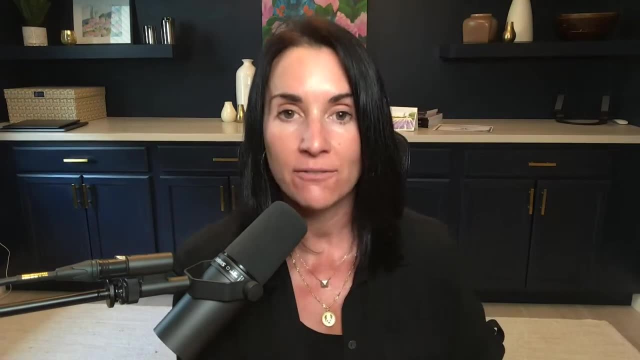 quickly, And I see a question here about the 7.812.. The Praxis: 7.812,. this is comparable because the 7.812 is the English language arts And these two tests are very similar: 7.812 and the 5.002.. 5.002 is a section of this book. 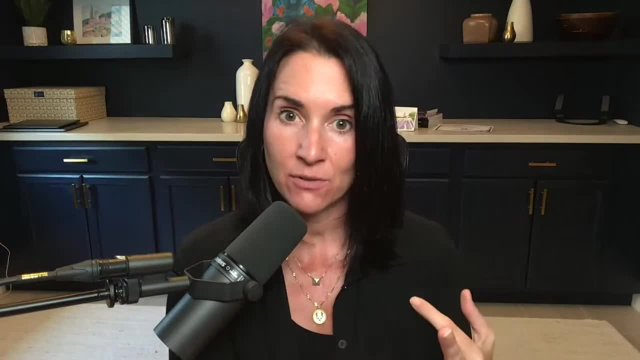 or of the test. I am working on a 5.006,, a 7.811, and a 5.017 book. They're the other elementary ed exams. They're a little different than the 5.001, but if you're. 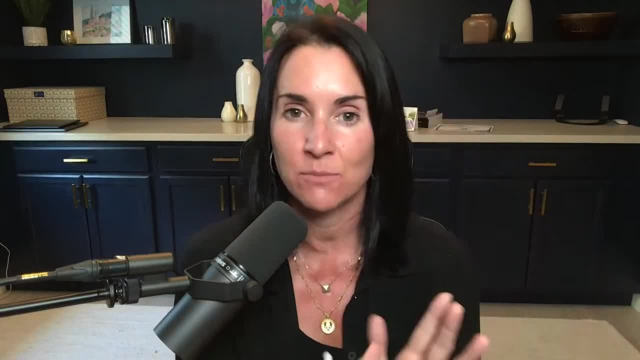 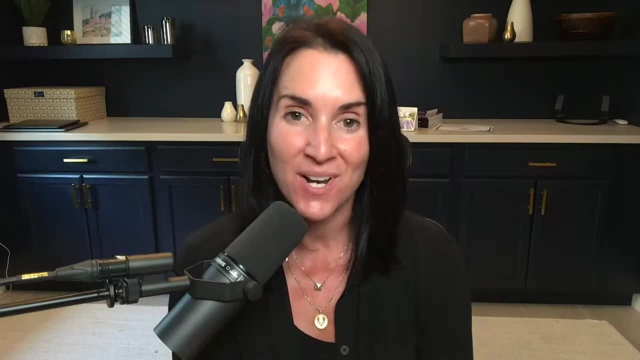 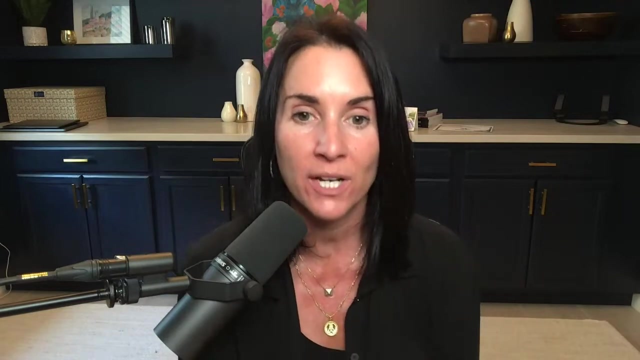 into English language arts. this is going to help you. The math on those exams are different than the one on this exam. Okay, So we're talking specifically about the 5.001.. The 5.901 is the same exact test And the other content area for teaching for elementary. I'm working on it. I've 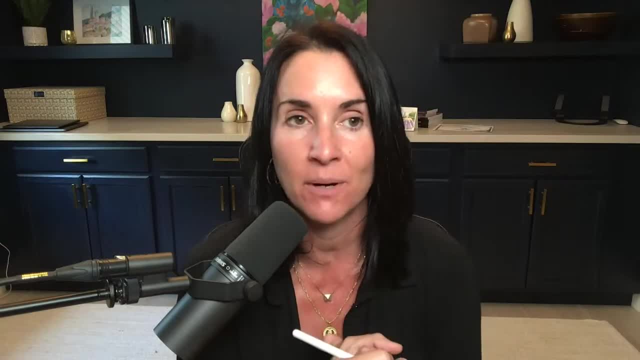 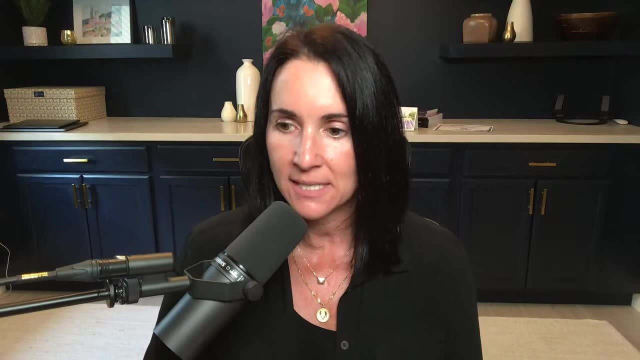 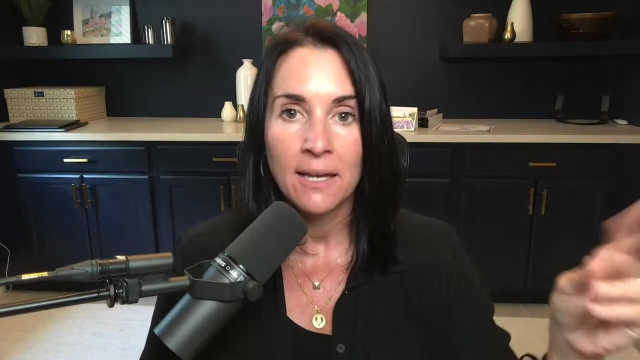 got some. it's in edits. I'm trying to pump it out as fast as I can, but I want to make sure everything is good with that. Okay, All right, A couple more questions. If you pass one out of them, you passed Yes. Okay, So these tests are scored separately. So if you pass, like the ELA, 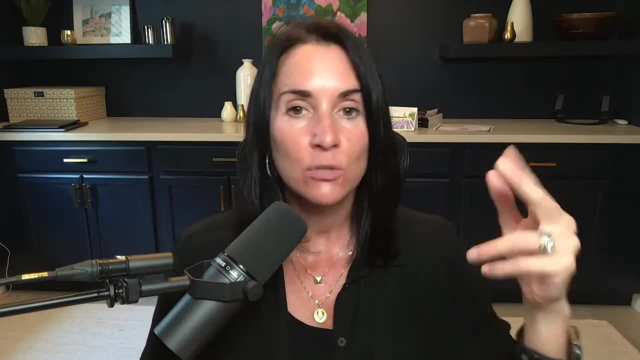 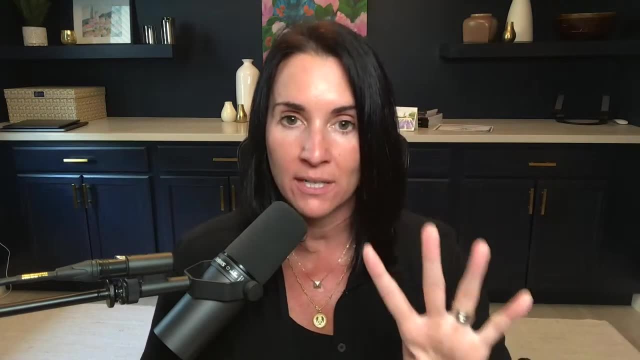 but you didn't pass math, social or science. you just take the math, social studies and science. You do not have to retake anything. They're scored separately. So it's one big test but four individual subtests. Do you have a book for the 190 foundations of reading? I do not have a book. 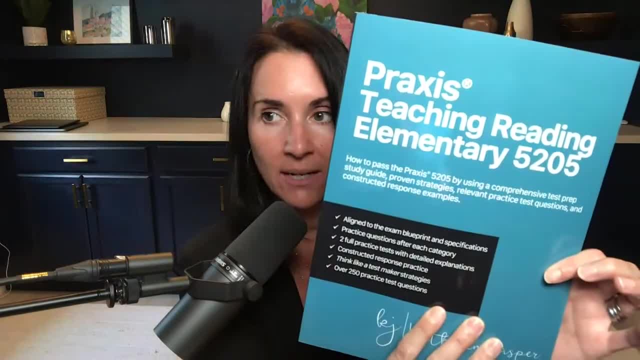 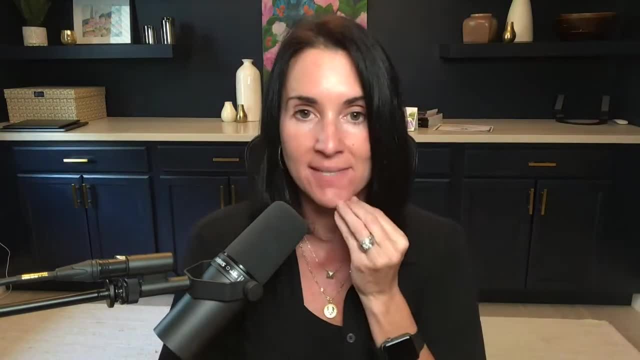 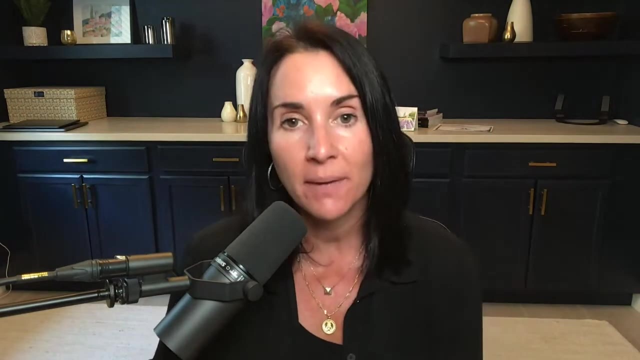 for the foundations of reading, but this teaching reading. lots of people use it to pass the 190.. Very similar. The tests are very, very similar. They assess the same things. Okay, Should we take the test all at once or in sections? I recommend the first time you take it. 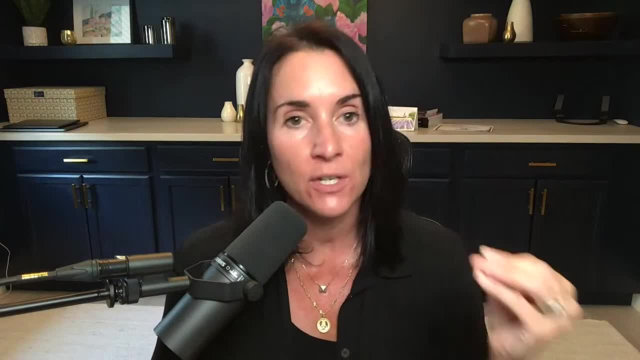 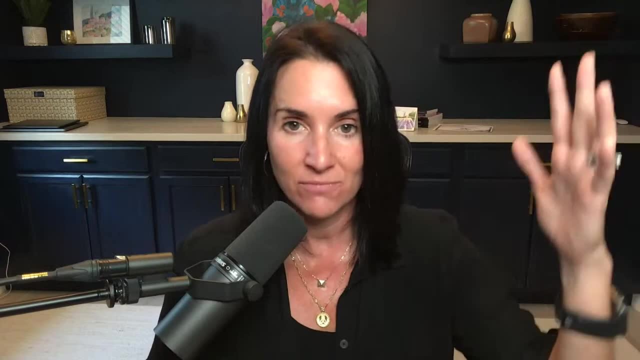 take it all at once, All right. If it's too overwhelming for you, then you can sign up for individual ones. The reason why I say take it all at once: because you might get two. You might get one, So just go for it And then, if you're not successful, you can take them individually. 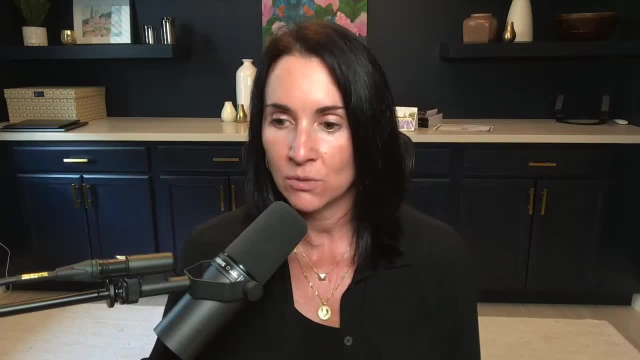 All right, All right, So so you need to wait 30 days to retake? Yes, you have to. it's 29 days, but you have to wait a month. Okay, Can this help the 5-0-0-7: humanities, language arts and social studies? Yes, So this? 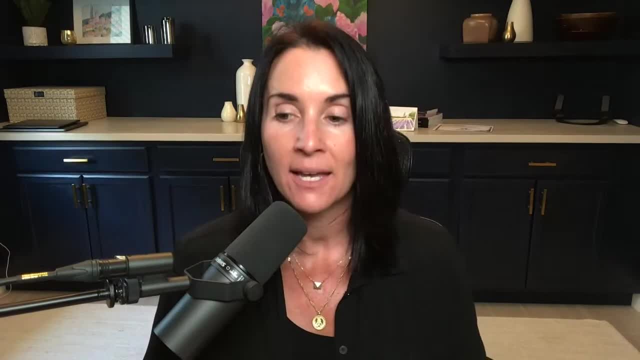 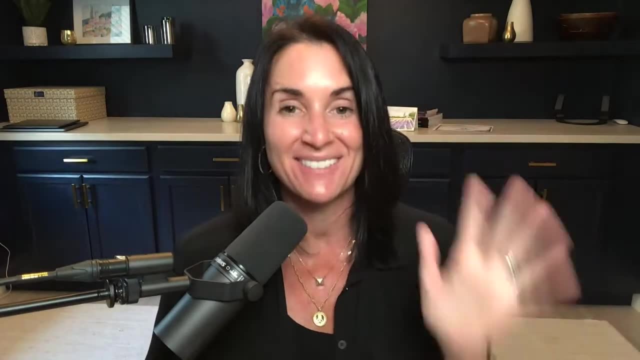 this particular section is going to be good for the 5-0-0-7.. Yes, But again, I have a specific program coming out very soon for the 5-0-0-6, which includes the 5-0-0-7 and the 5-0-0-8.. So I 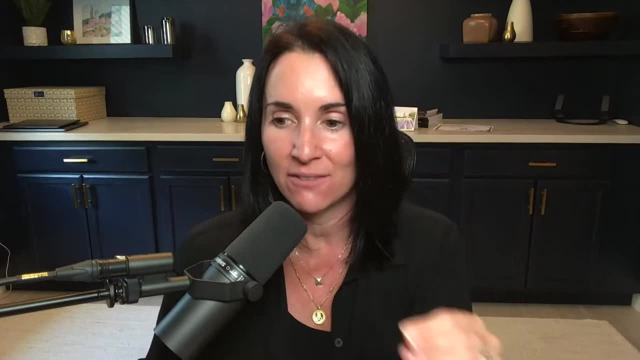 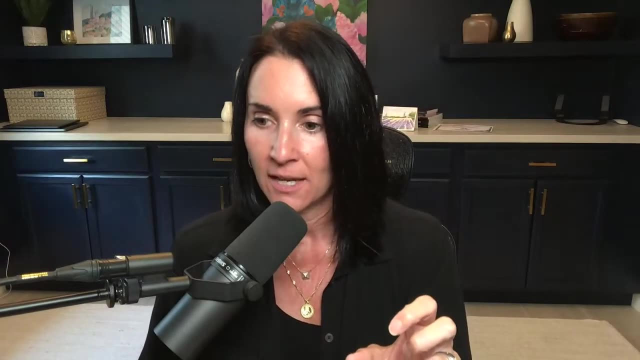 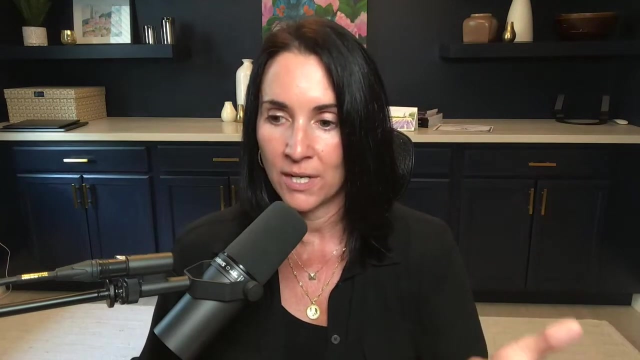 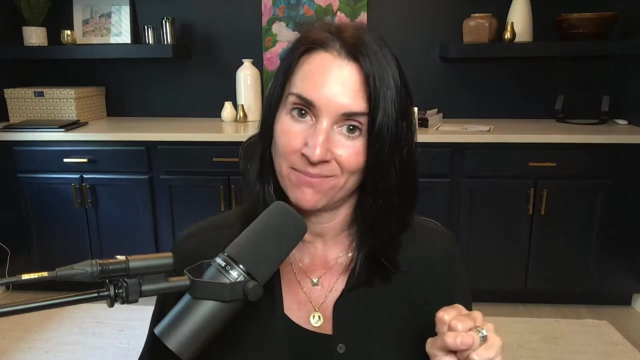 there's so many numbers, there's so many tests, but let's just focus today on the 5001, you will get a lot of information that will help you with the. some people are asking about the EC6.. Yes, The Praxis- 5901.. Yes, The FTCE K6.. We don't do FTCE. I have to be very, very clear. 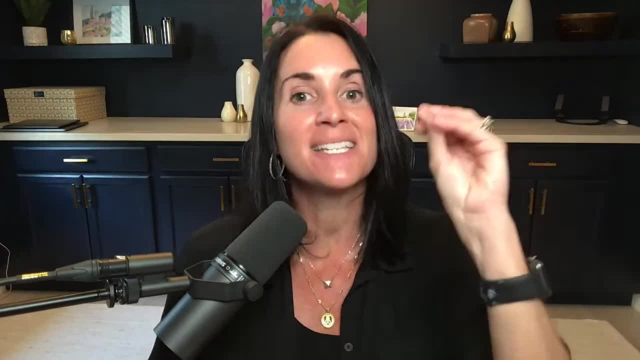 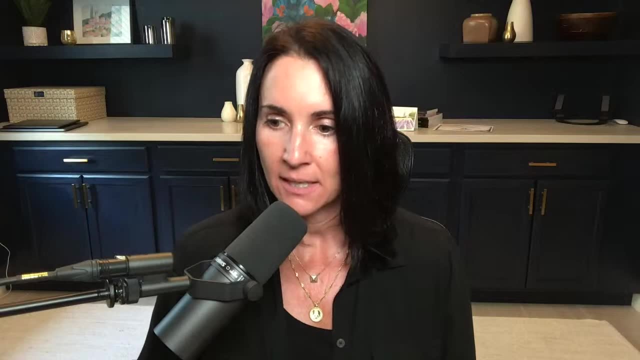 about that. This is for the Praxis. They are both elementary tests, but this is for the Praxis exam. Okay, Somebody said I was only studying using practice tests, and this is affirmation already that I'm not studying right. Do you think 240 tutoring is efficient enough to pass the Praxis? 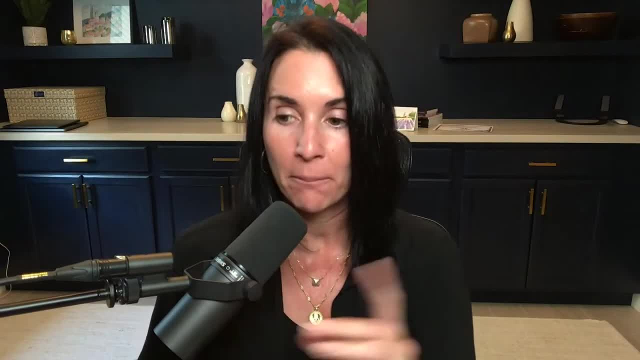 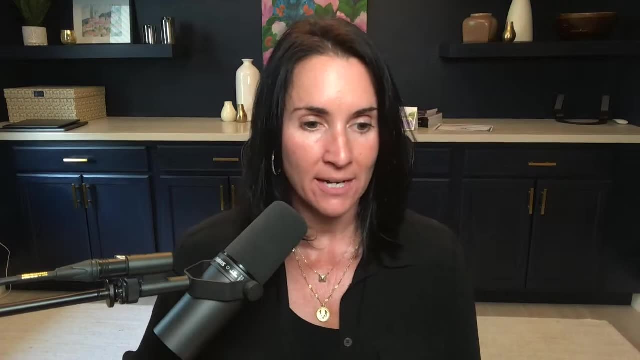 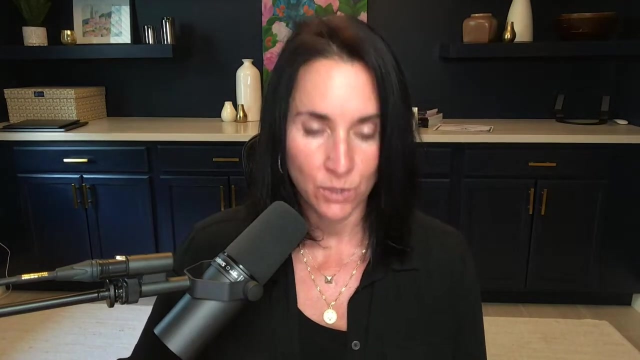 Well, 240 tutoring is my competitor, and they do have great stuff, but practice tests alone are not going to do it. Okay, All right. So let me go to the next part here, and we are going to let me share screen, entire screen, and we should. you guys should see Praxis. 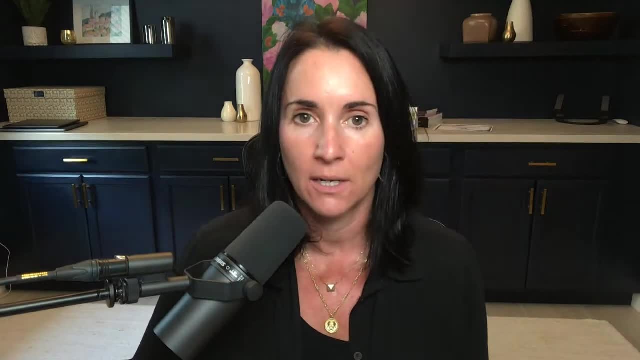 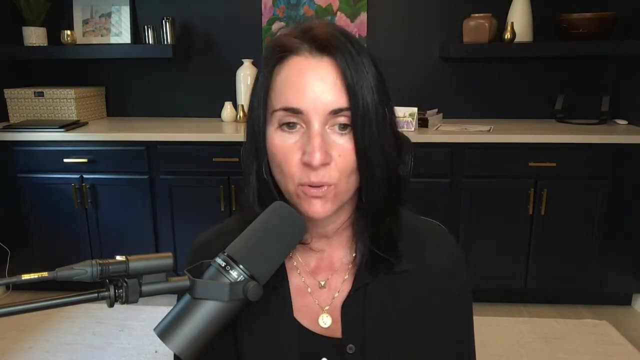 Elementary education, multiple subjects here? Okay, good. So let's just take a quick look at the blueprint Now. I always say the blueprint is one of the most important things you can. you can look at when you're, when you're trying to study for a test. This breaks down all the 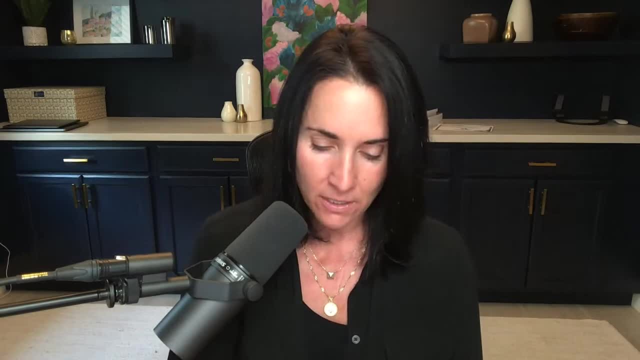 sections of the test and you can see here the approximate number of questions. All right, I covered up my. please hold I covered up my. there we go. All right, So it's important to know this Now. notice that the five zero zero. 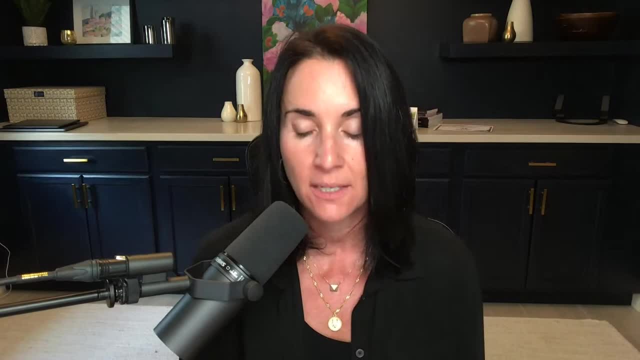 two, which is the reading and language arts, is the biggest portion of the test And it does give people a tough time. The math is also tough on this exam. Yeah, it's elementary, but there's pretty tough math problems on this exam, So we want to make sure we're prepared here. 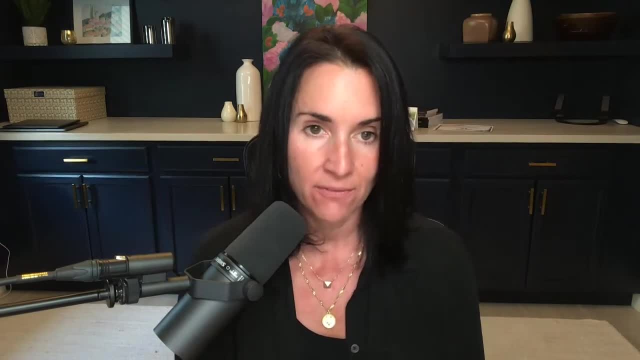 for sections You get four hours and 25, 4.25 hours. So you're talking four hours and four hours and 15 minutes there And it is straight up selected response, meaning it is all multiple choice. There's no rating on this. 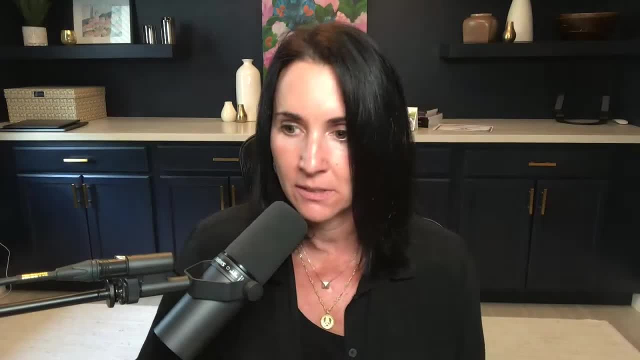 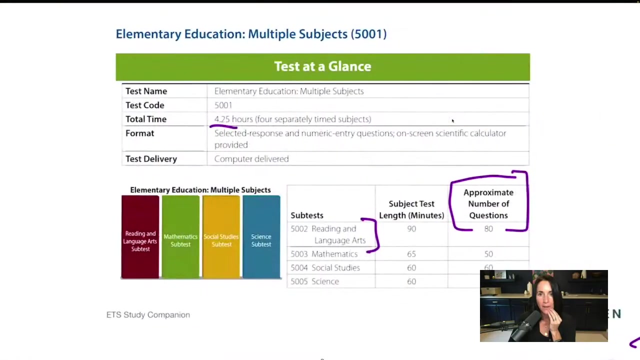 So that's really good. Okay, Just make sure again that you guys can see me. You guys can see this right, The screen share on this particular. okay, hang on, Let's do it again. How about now, Can you? 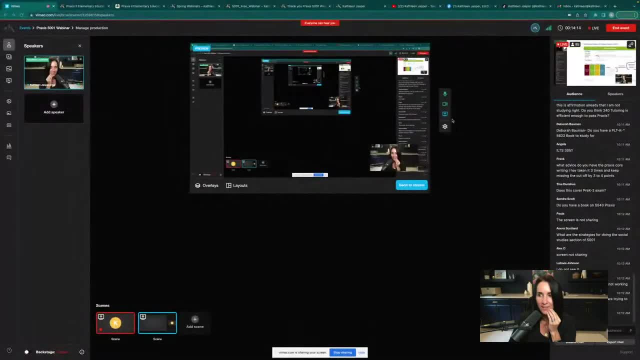 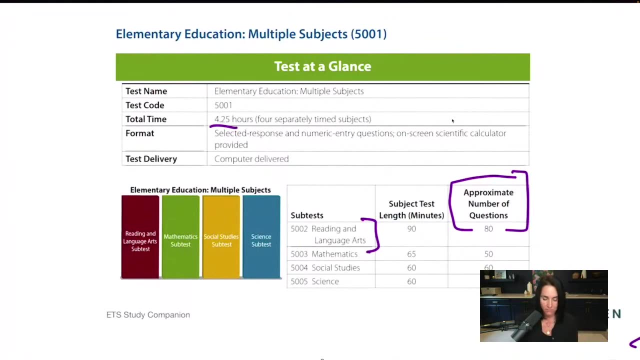 see it now. There you go, I think you can see it now. Okay, cool, Sorry. So this is the blueprint of the exam and you can see four sections: 4.25.. 4.25 hours And we have the language arts and reading and we have all the questions. Notice. 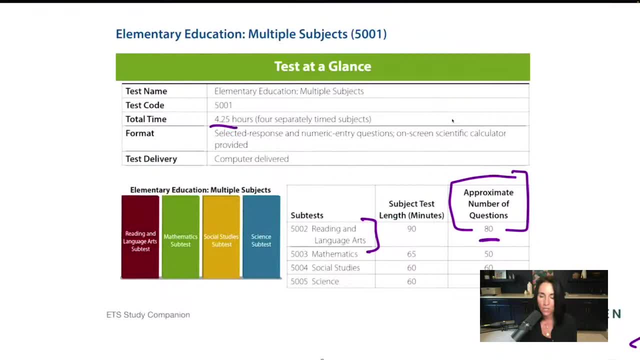 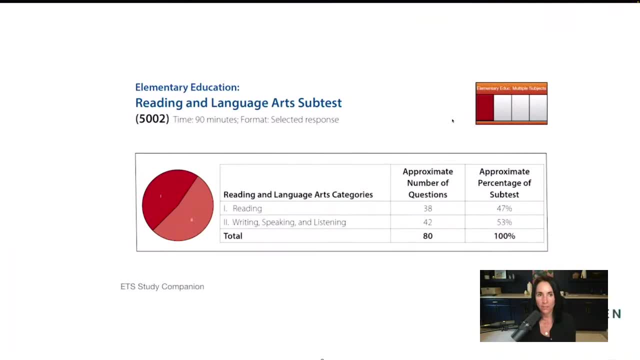 the bulk of the test is coming from that- reading and language arts there. So this is really important. Now, below that, you're going to need to go into the actual specs for the subtests. Okay, So right here you can see that now we're in 5002, which is the reading and language arts subtest. 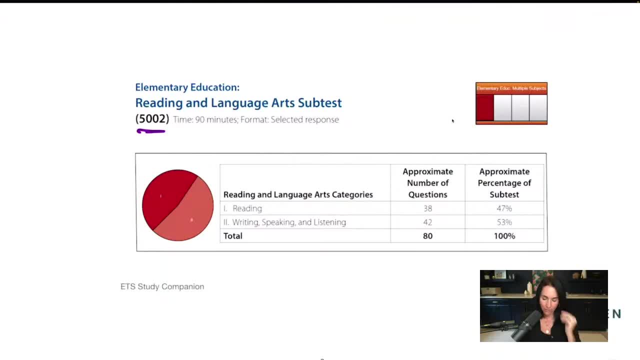 And you can see that we have 38 questions are coming from reading and 42 questions are coming from writing, speaking and listening. So the writing, speaking and listening is a bigger portion of the reading exam. reading and language arts exam. This portion of the test can be: 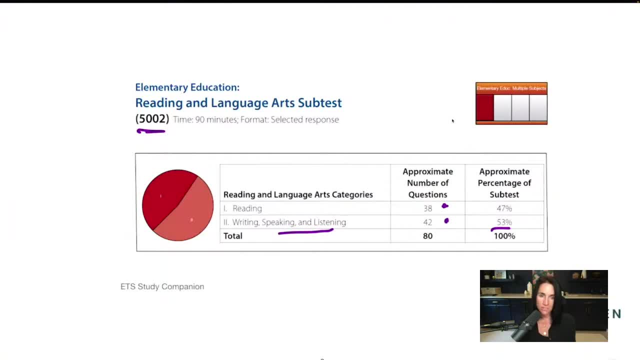 difficult for people, but we're going to go over it today. So the way this is going to work, I'm going to section out each part of the test, I'm going to go over the main components of the specifications and then we're going to get into specific practice problems. All right, Whenever. 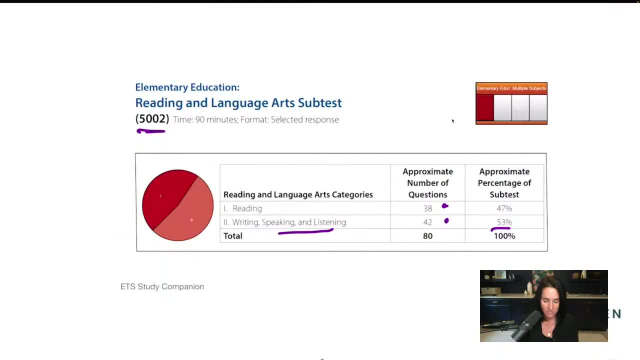 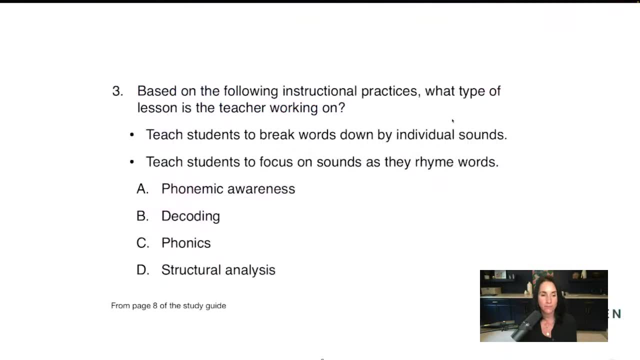 you see on this presentation something that comes from ETS. you're going to see this ETS study companion on the bottom. You're going to see a question from the study guide that I gave you when you signed up for this. You're going to see from page eight of the study guide, That way you can follow along with me in. 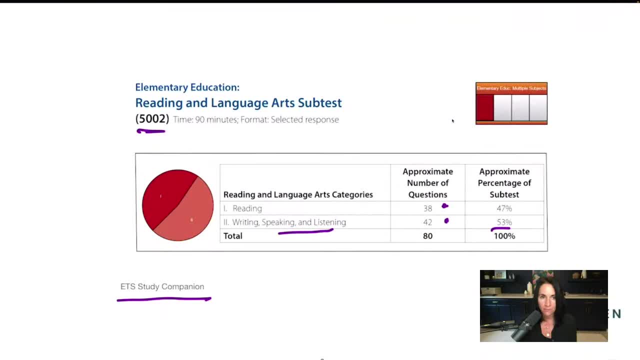 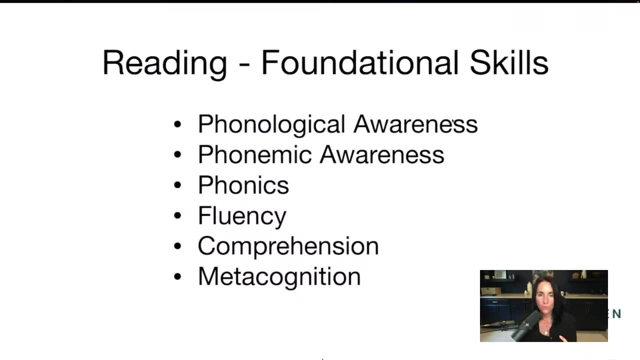 the study guide. Okay, All right, Let's go back to here. We are working on the 5002 subtest And let's talk a little bit about what is on that subtest. So the reading portion of an elementary education exam is going to be everything: foundational skills. Okay, So we're talking. 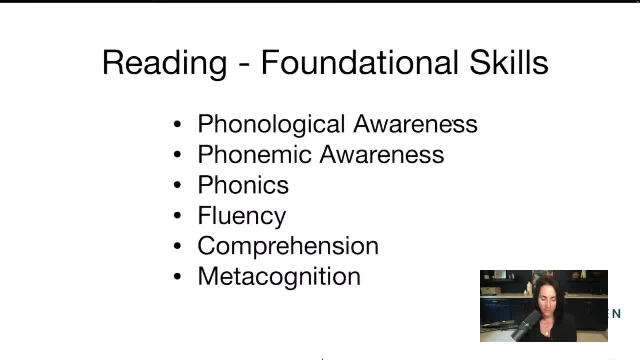 phonological awareness, phonemic awareness, phonics, fluency, comprehension, and there's a big, big importance of metacognition. right, Metacognition is teaching students to use their brains. It's thinking about thinking Those types of things where we say, okay, how would you figure out this word? That's a tough word. Let me read. 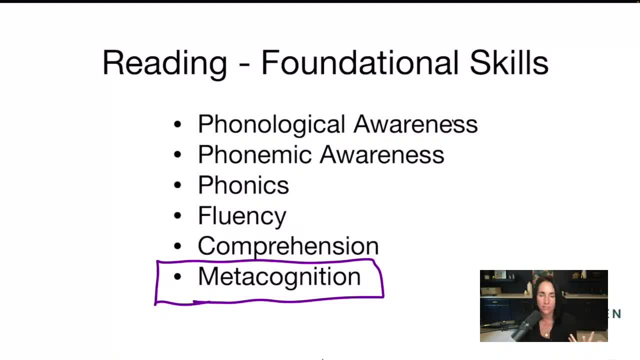 around it And you kind of model those skills of how to use your brain to figure things out. That's a big part of the reading portion. You also have to have a very good grasp on these foundational skills And I cover them in depth. 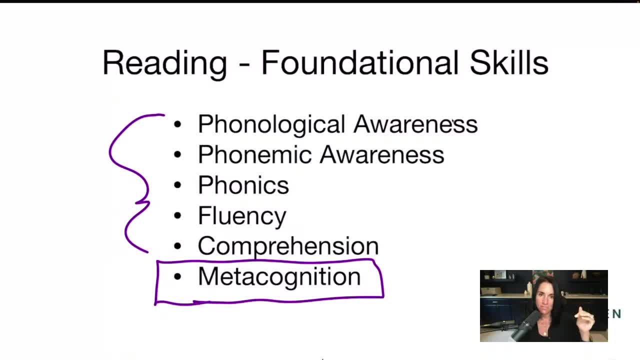 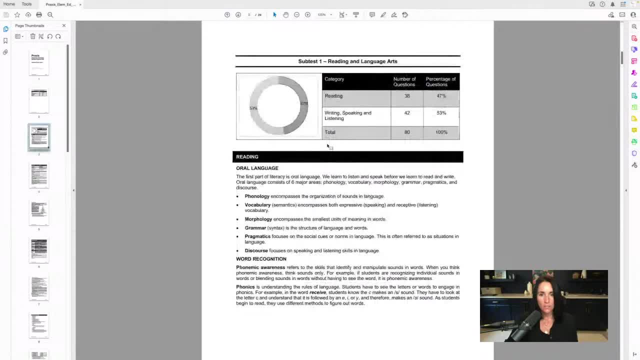 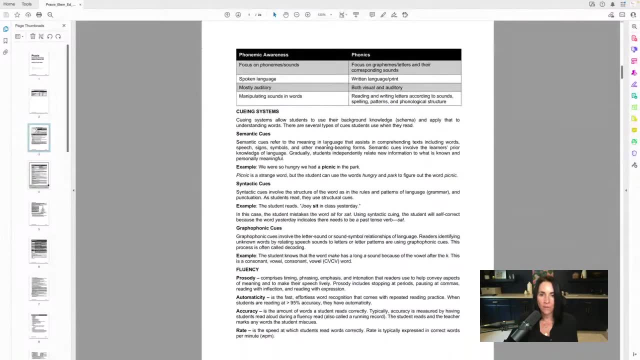 in the study guide And I even cover them in the free study guide. You'll notice that in the let's see if I can just go over here, Let me go here. You'll see here that I have a lot of information in the reading portion of this free study guide because it is so packed full. So 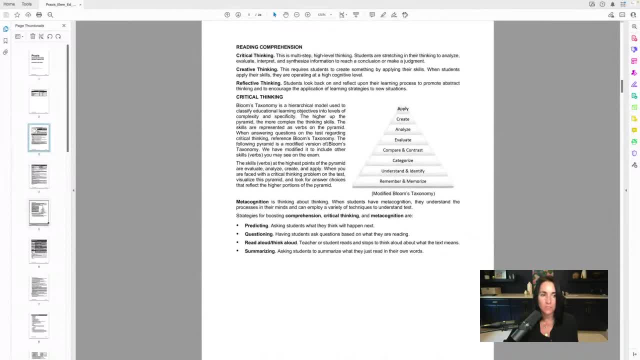 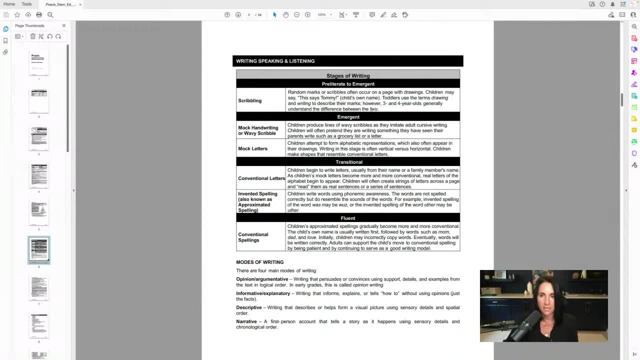 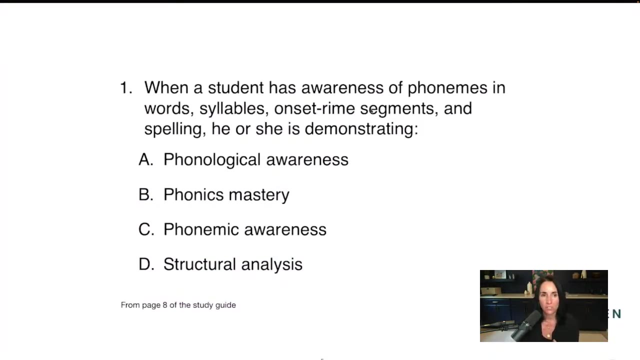 definitely read this part of the study guide. Don't just go to those practice problems, because there are really good information. There's really good information here in terms of the sections of that exam. Okay, All right, Let's go back to my presentation. All right, So if we're talking about these foundational 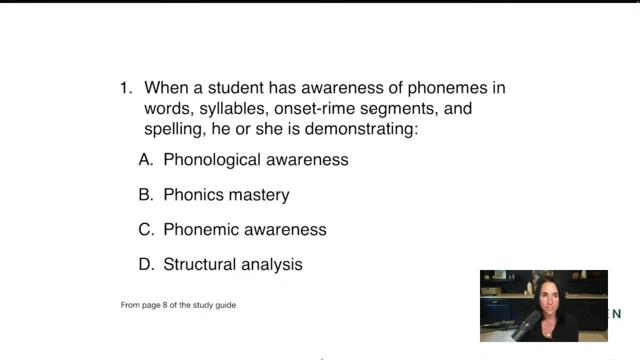 skills, which are the bulk of this test. let's have a look. This is on page eight of the study guide, So I'll give you a second to flip or click or whatever, And remember my my. if you've seen some of my videos, you know that I always say: start backwards. We're going to start with the 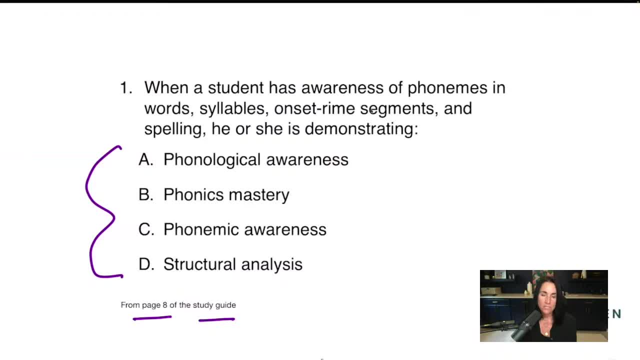 answer. The answer is first Now. the reason why I do this is because it sets me up To understand what's going on now. this particular question only has single- you know single- answer choices. They're not like paragraphs, but if this had like a bunch of information in the 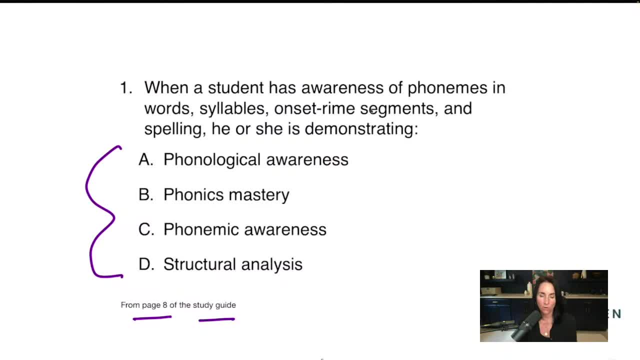 answer choices. it really helps to work backwards, because then you can start to cross out bad information and underline good information. I have a whole video about this on my YouTube channel. It's called work backwards. Definitely check that out. I'm going to give you a tour of my 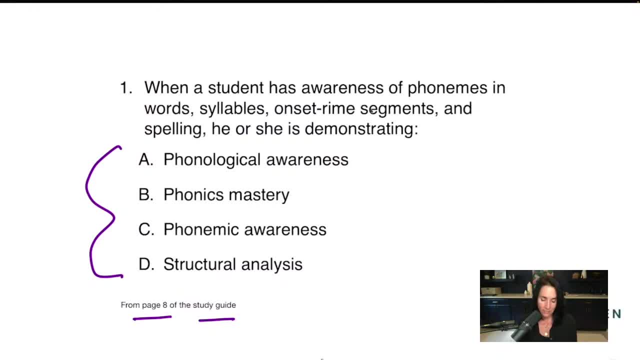 YouTube channel when this is over. but we always want to start backwards, And here I can see phonological awareness, phonics mastery, phonemic awareness and structural analysis. So right away, my brain is like: okay, I know that I'm going to have to figure out which skills these. 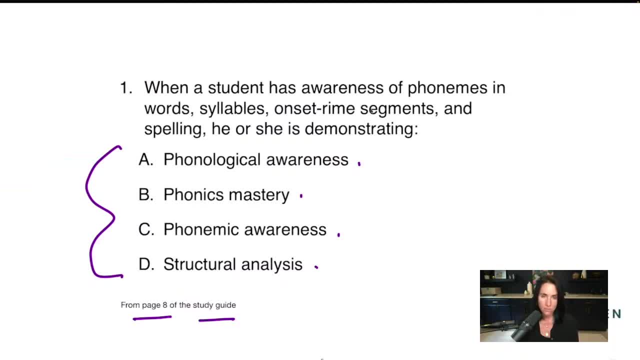 students have because these are skills in the answer choices. All right, So now let's read the question. When a student has awareness of phonemes, words, syllables, onset, rhymes, segments and spelling, he or she is demonstrating. Well, this is phonological awareness. Now, 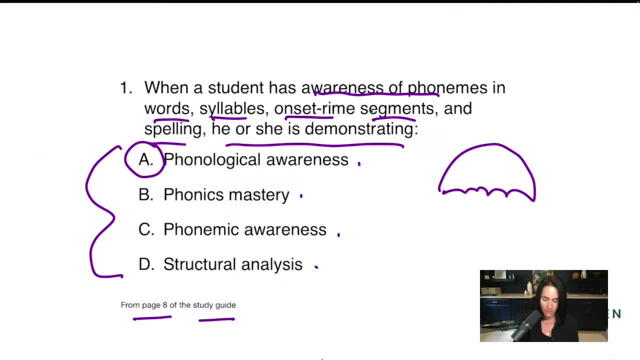 let me show you real quick in a really bad drawing. I also have a video on this. What I want you to do is pretend that phonological awareness- I'm just going to abbreviate- is the umbrella, And underneath it we have phonemic. 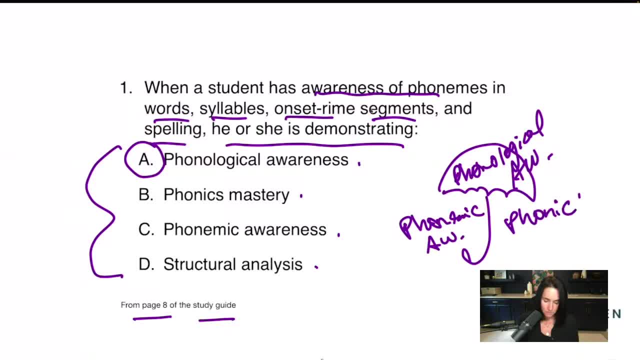 awareness and phonics. All right Now, phonemic awareness is sounds only. You don't need to see it, You do not need to write it, You do not need to know that a B, when you see the letter B, makes a B sound. All you need to do is use your ears. And when I was 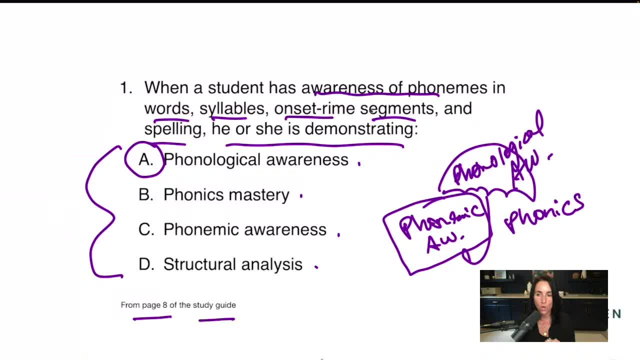 a reading teacher. my reading coach said you can teach phonemic awareness in the dark Meaning if I was like a first grade teacher or a kindergarten teacher And I said to my students: okay, students, say the word bat and they say bat. And I say: say the word bat. and they say bat And I say 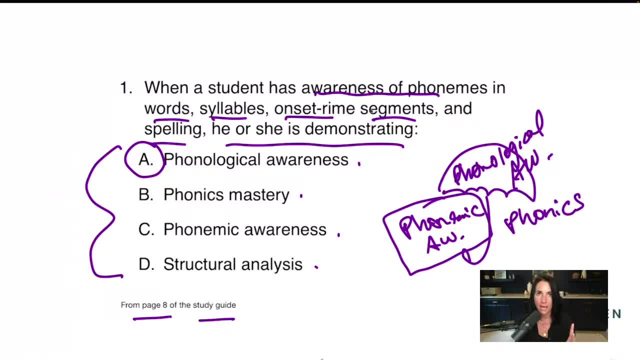 say the three sounds in bat And they go B A T. They don't need to know it's a B in the beginning, a T at the end and an A in the middle. They just know the sounds. This is the very. 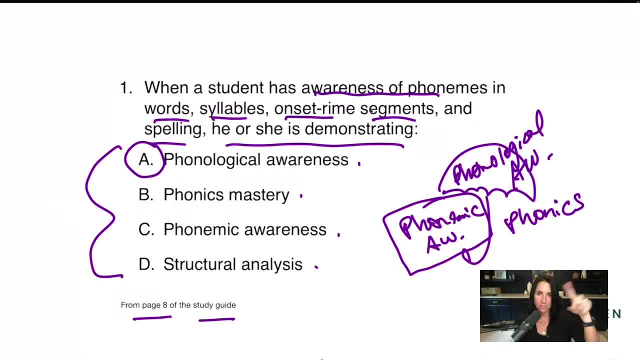 beginning piece And this question is saying all these other things: syllables, words, onset, rhymes, segments. That is not phonemic awareness. Phonemic awareness is sounds only Now phonics. Phonics is when we actually bring in the symbols. So when we see the word B, we know it makes a B sound. 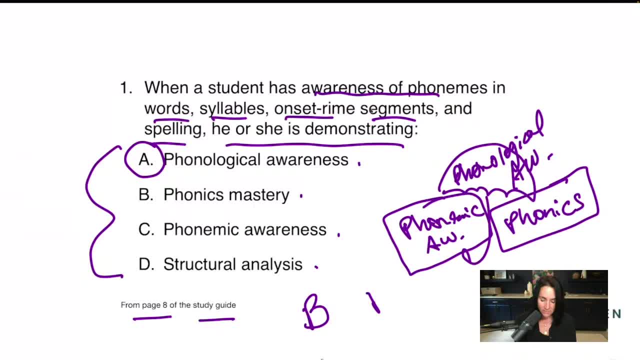 When we see not the word B, the letter B, sorry, When we see the letters P and H together, we know it makes a F sound, or an F sound, I should say. And when we see in like let's say in the word make, When we see a vowel next to a, 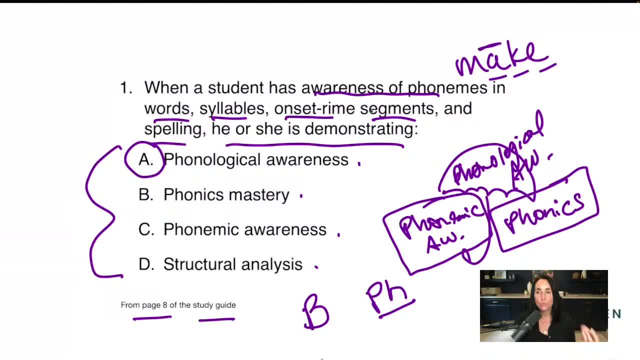 consonant and a silent E. we know this. A is long. These rules to symbols using letter symbol correspondence or sound symbol correspondence. this is phonics. You have to see the word Now. when you combine these things together, you get that phonological. 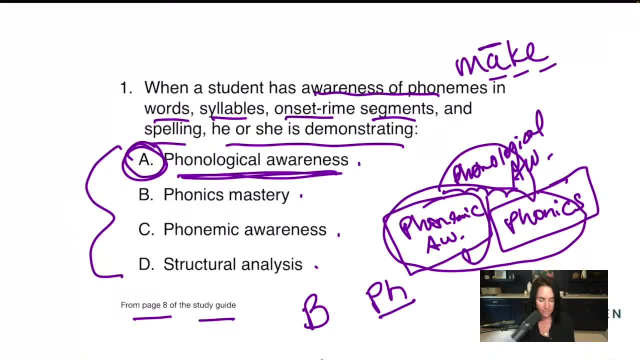 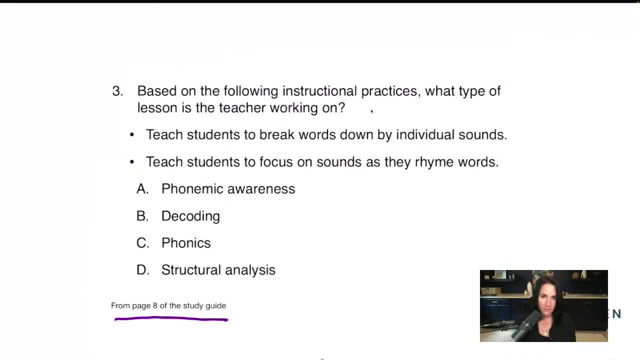 awareness, And that's why the answer is A. All right, Let's have a look at another one here. Oops, Sorry about that, Let's go back. All right, Number three: this is also from page eight in your study guide. Now again, I'm going to just glance quickly at my answer choices and I have phonemic. 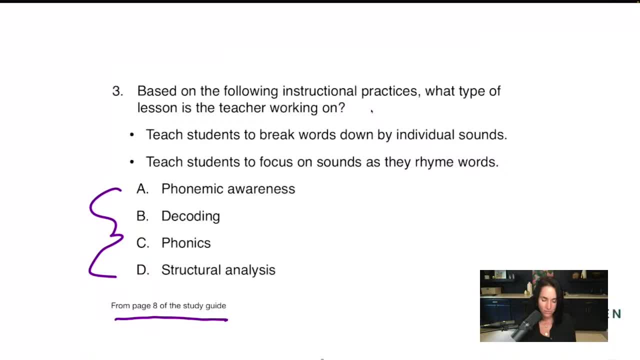 awareness, decoding, phonics and structural analysis- Again, these are all skills. So I'm setting myself up to understand what's going on And then I'm going to keep working backwards. I'm going to go here. Teach students to break words down by individual sounds. Teach students to. 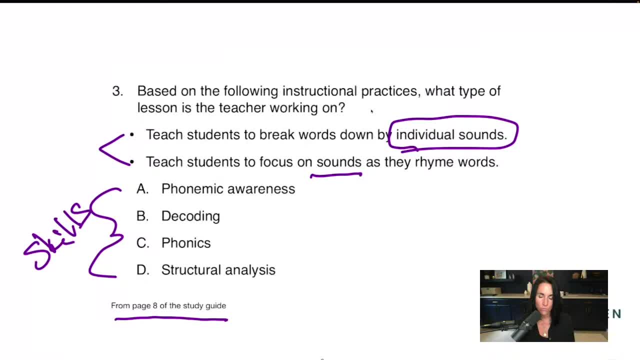 focus on sounds as they rhyme words. Rhyming is a phonemic awareness activity. Notice, I have sounds and sounds. Well, right away, I know it's not decoding. Decoding and phonics are the same thing And structural analysis is breaking up words. D is out A. I already got A before I even read this. 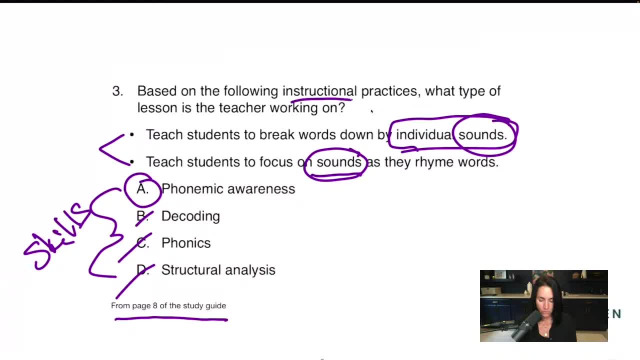 part. Let's try A. Let's just read the top part, Based on the following instructional practices: what type of lesson is the teacher focusing on? Well, we have those sounds. We have those sounds. We're not talking about looking at the letter and figuring it out. This is going to be phonemic. 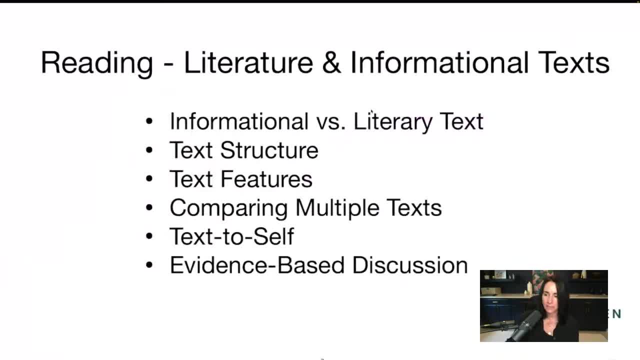 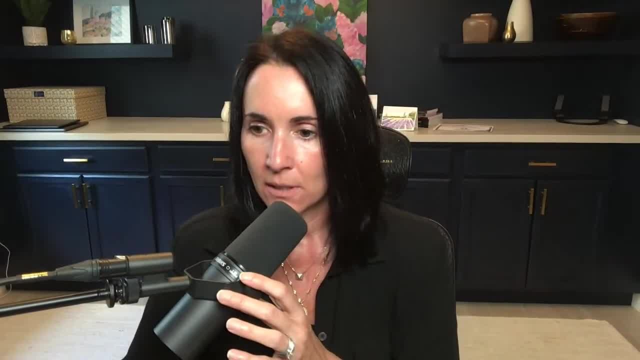 awareness. All right, Now let's have a look at reading and literature. All right, So let me go here and just see if anybody has any questions. All right, Anybody have any questions. I see Yes, yes, yes. 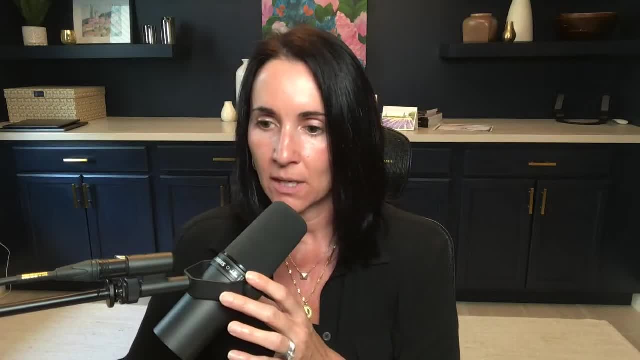 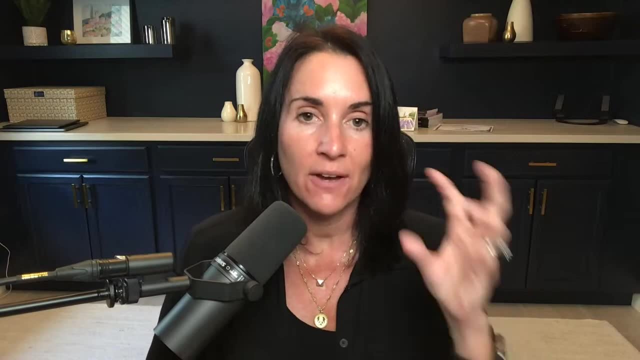 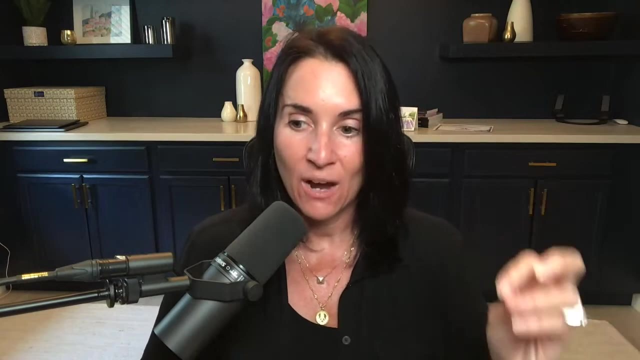 You can see my screen, Perfect, Okay, All right. So those are the. let me go back here. Those are the foundational skills for reading And you're going to need to know those, And those are in depth in the study guide. Now we're going to talk about the writing: speaking. 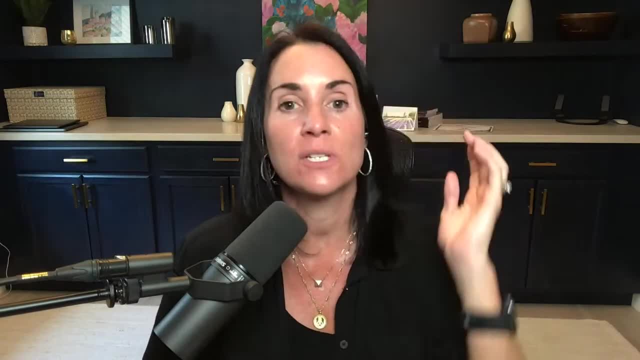 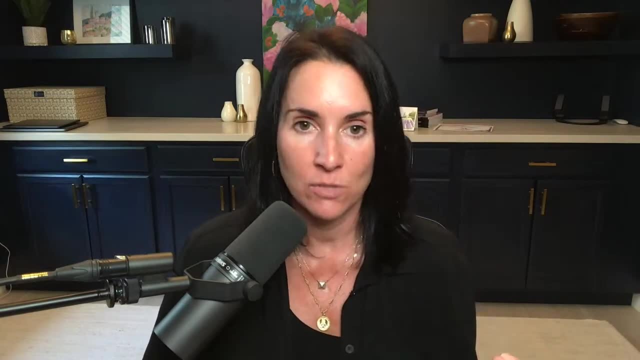 and listening part, which is also very big. We have to teach students how to speak, how to listen actively, how to write the writing process, things like that, And that is going to be a big part of the English language arts exam as well. So let me go here. Let 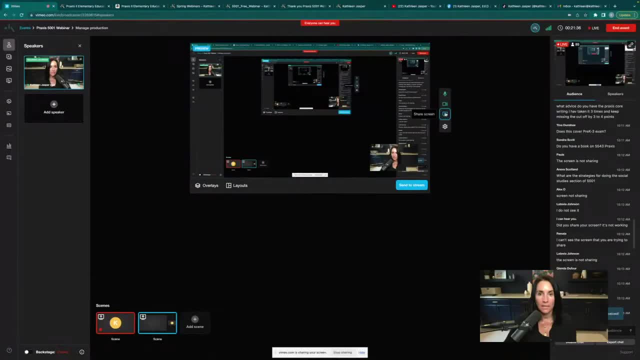 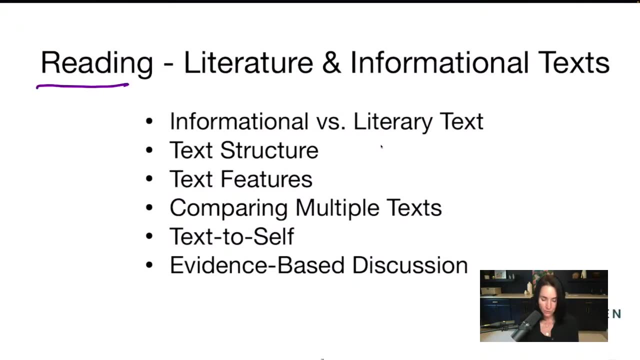 me share my screen again And we should be good. Yes, we are good. Okay, So now we're talking also about reading, literature and informational text. This is a part of reading. Oh, I said we were going to writing. Actually, there's one more part of the reading. One thing about this exam is you. 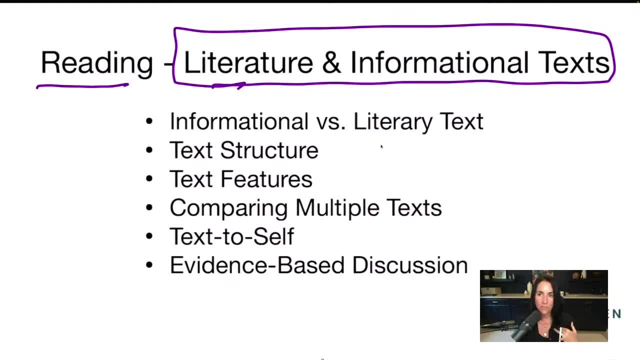 want to make sure that you understand the difference between literary text and informational text, And this exam is: you got to use them both. Good reading and language arts teachers use a balanced literacy program Now. we're hearing a lot about balanced literacy in politics right now And 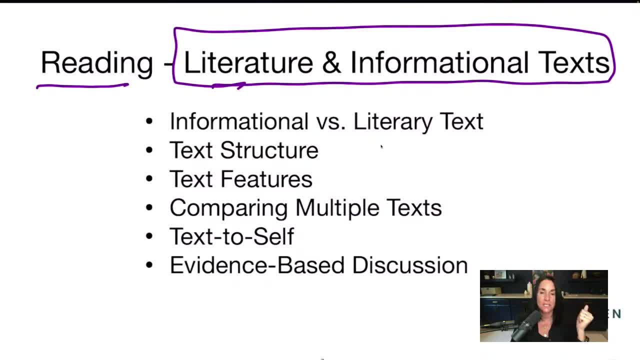 people seem to confuse what balanced literacy is. Balanced literacy means that you're using a variety of texts in your classroom. You're using stories, You're using newspaper articles, You're using brochures, You're using timelines. You're using all these different types of texts. You're. 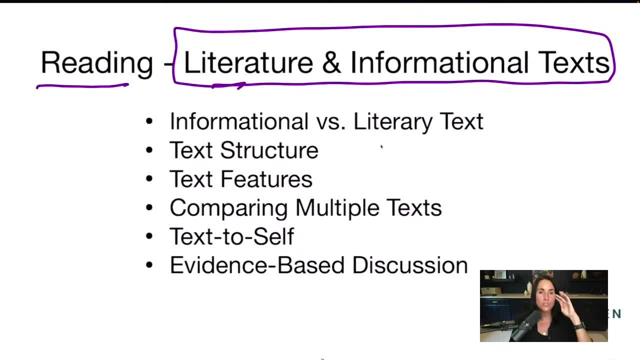 using different ways in which we get information And a print rich environment in your classroom is really important. So these words- balanced literacy, print rich, variety of text- those are all good words you want to look for in the answer choices. Okay, You need to know the difference between the: 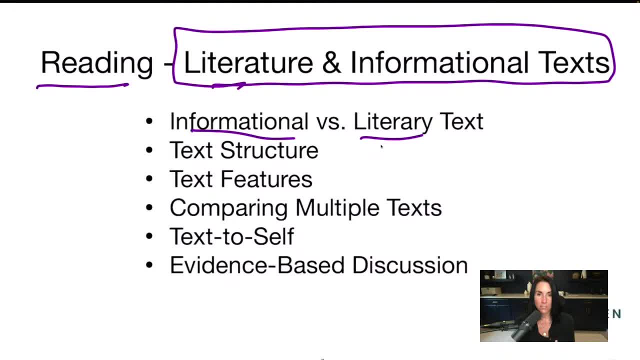 two. So informational text is going to be nonfiction. It's going to be, you know, your social studies passages, your science passages, things like that. Literary text is going to be those articles and things like that that we use in elementary school and middle and high school. You're. 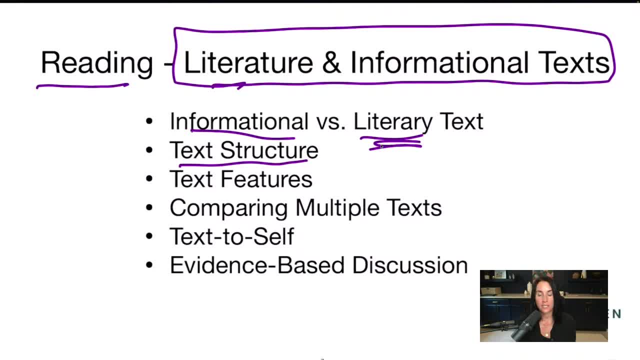 going to want to focus on text structure. So text structure are things like: is it a cause and effect? Is it descriptive? Is it a narrative? Is it a problem solution? Is it chronological Understanding? those will help students sequence events and understand what's going on. Text structure is: 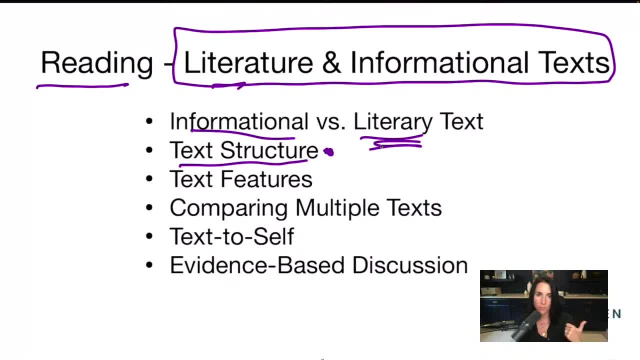 also important for the writing section, because if you're telling students to write a persuasive piece rather than a narrative piece, they need to know the difference between those, And then, of course, you're going to want to know the difference between the two, So you're going to 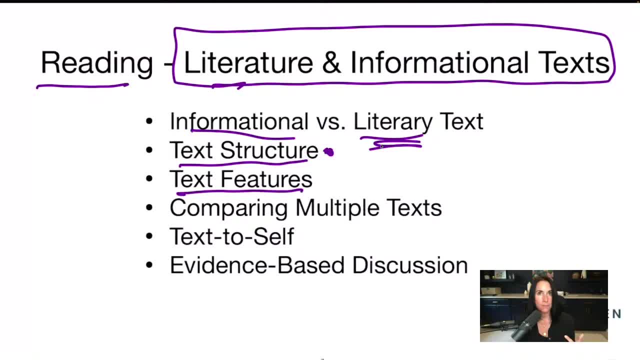 want to know the difference between the two. And then, of course, text features: right Headings, bolded words, graphs, charts, pictures. those types of things are really important. We're always going to be able to compare multiple texts. So will students. Here's another good word text to self. 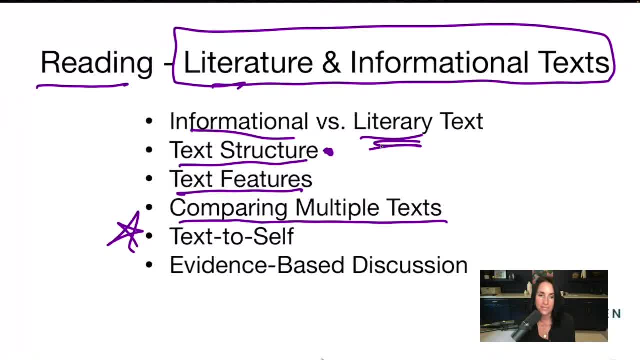 What are we trying to do with students? We're trying to help them see themselves in text. That's why it's so important to have books and stories that represent everyone in the classroom, not just a certain group of people who may be pushing an agenda, But instead all students are represented. 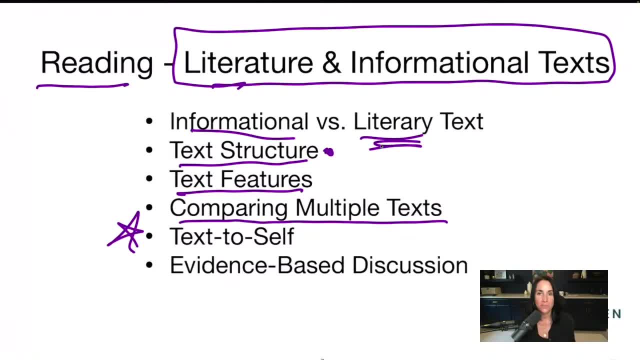 in literature so that we see students from all different communities, all different genders, all different races, religions, everything. Our library should be full of that information. And then, of course- this is a big one- evidence-based discussion. We want students to make claims after they read. You know, you might say: how did this happen? Or 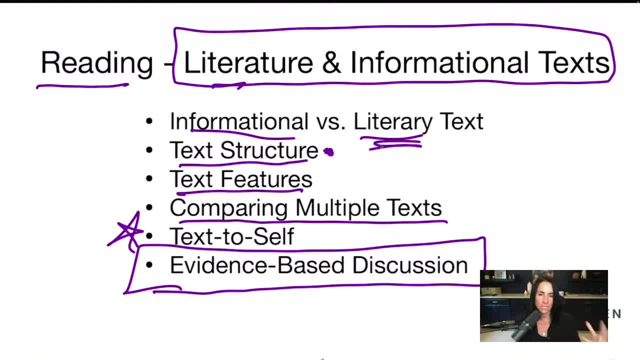 how does this make you feel Or what do you think would happen here? You know we're predicting, we're summarizing and things like that, And when students can back up those claims or support those claims with evidence in the text. that is the key, Because a big part of the English reading and 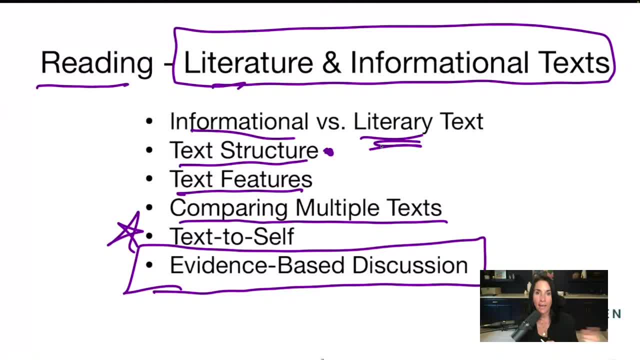 language arts standards is that they can say, okay, I think this, right, I think he was mad because of this. And, as the teacher, you say: where in the text did you see that? And the student says, right here, It says this. And that is starting to show students that they have to back up those claims. 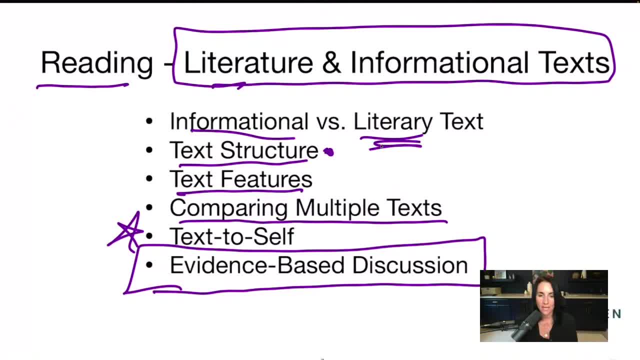 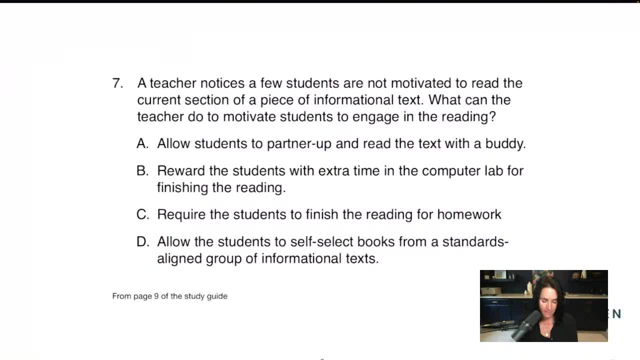 with evidence in the text. We start it young. We got to get them using that evidence, using that information, And that really helps. All right, Let's have a look at number seven, And this is from page nine in the study guide. So go ahead and turn to page nine Now. in this one, this is: 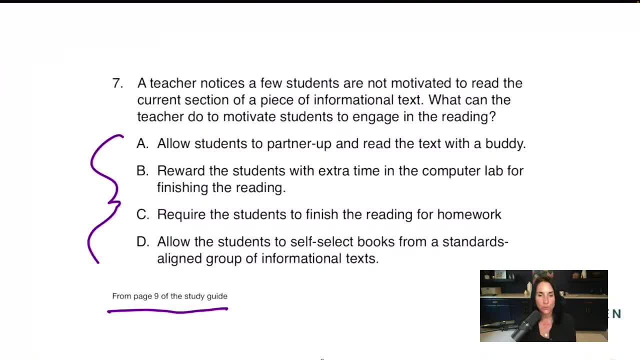 a good work backwards one, because we have four answer choices with tons of information And I get a lot of calls from people. Well, not calls, I get a lot of calls from people. I get a lot of emails from people that say what if there's more than one right answer? What if there's multiple? 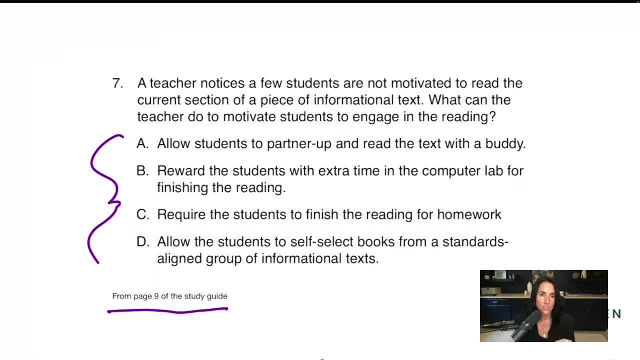 right answers? There is not, Unless the question says: choose all that apply or choose two. you know, and you'll get those as well, But this one is asking for one answer. That means there is only one proper answer. Now let's look at the answer choices so I can show you why some of 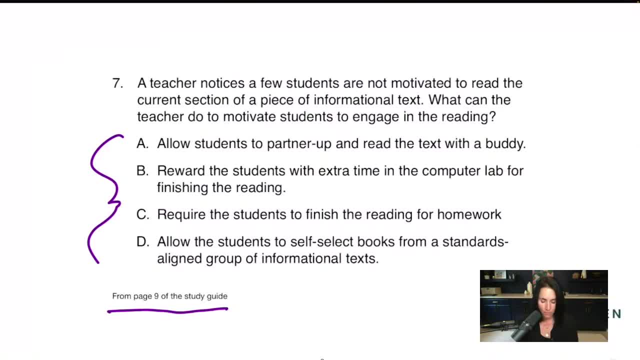 these things are correct and some of them are incorrect. We have: A- allow students to partner up and read the text with a buddy. All right, That's a good answer. B- reward students with extra time in the computer lab for finishing reading. Okay, I'm going to. 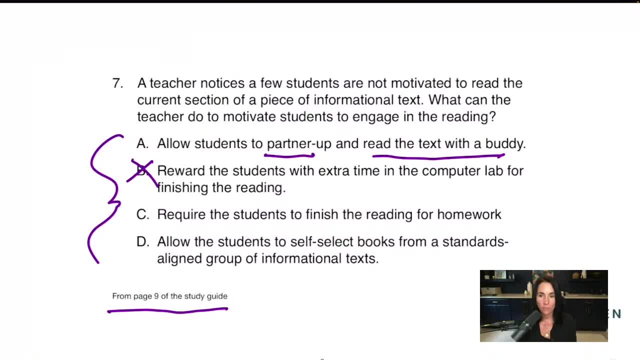 cross that out right away. Rewarding students works. I would probably use this in my own classroom, But on the test, extrinsic rewards are usually not the way you're going to motivate students to finish their reading. We've got to use intrinsic rewards according to this test Now. 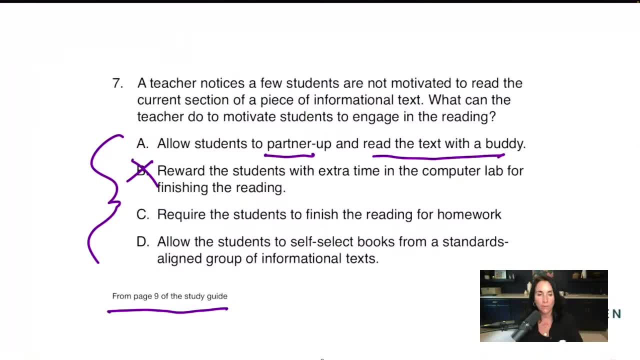 I use Jolly Ranchers chicken sandwiches. extra time homework passes. all that stuff works. You know it works if you're teaching, But on this test we're looking for intrinsic rewards. All right. C: require the students to finish the reading for homework. Homework is typically a 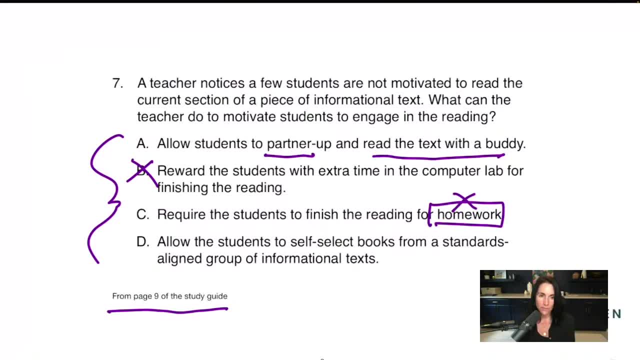 bad word on this test when presented like this. We want to engage students in classwork. Most of these questions are about classwork activities. I'm going to cross off C And D. allow students to self-select books from a standards-aligned group of informational texts Has all the 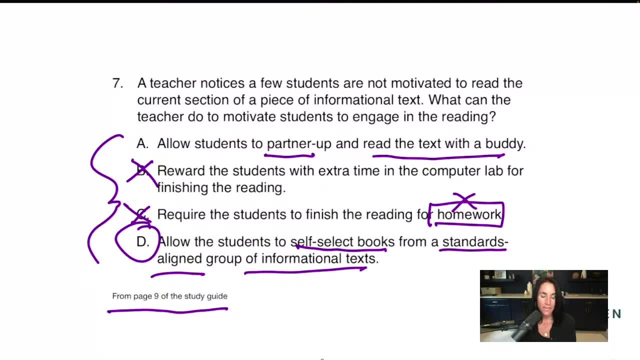 good stuff in it. I love D. I'm going to choose D And I already have the correct answer: by working backwards. But let's go ahead and have a look at the question. Let's keep working backwards. What can the teacher do to motivate students to engage in reading? Well, self-selecting books is a really 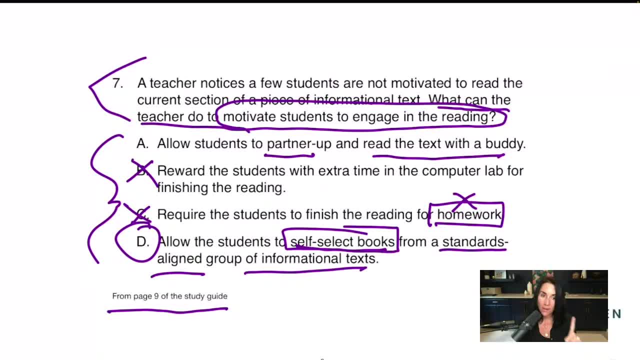 good way to motivate students. They get to pick the book they want, But we make sure those books are standards-aligned right, Because we want to make sure we're always using those standards to plan instruction and to motivate students. So we're going to cross off C And D: allow students. 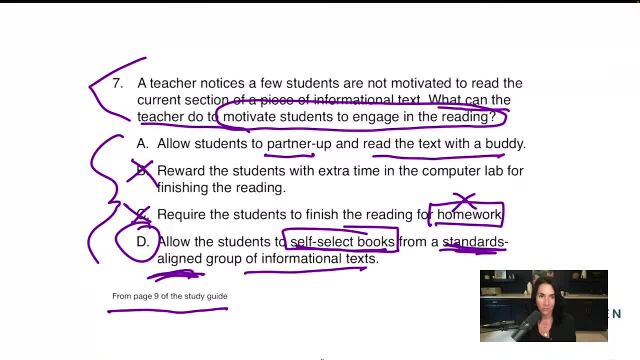 to choose books and things like that. So that is going to be there, And I didn't even have to read all this stuff up here. Doesn't make sense. Okay, So that works there. All right, Now let's talk. 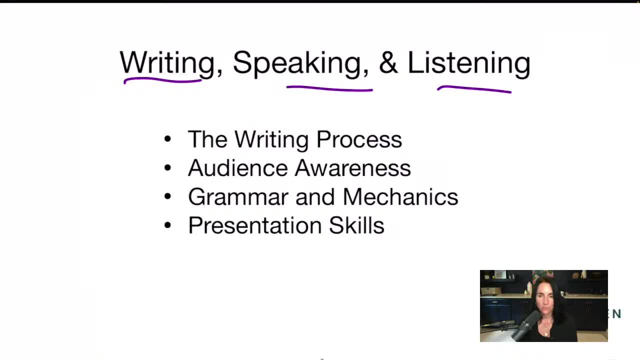 about writing, speaking and listening. So in this portion of the reading and language arts, we have the writing process, So the draft, or let's say the pre-writing stage, which is going to be brainstorming, watching a movie, looking at a picture, talking about it. Then we have the 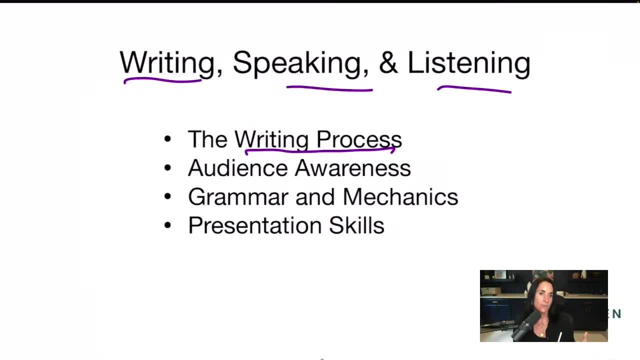 drafting stage, the revising stage and the reading and language arts. So we have the writing stage, we have the rewriting stage, we have the editing stage and I have those all in the book. But the writing process is really important. And one thing about the writing: 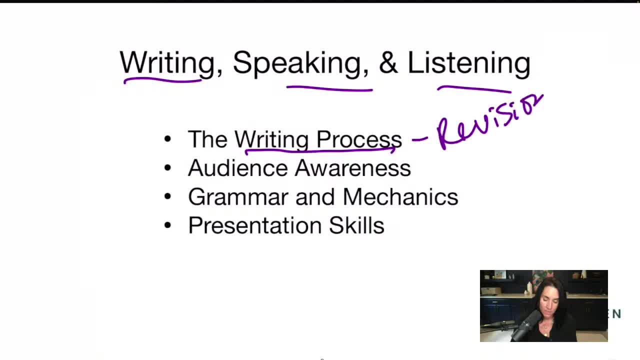 process that is most important is that we focus on revision. Nobody writes a perfect paragraph, perfect sentence, perfect book, perfect essay the first time around. We have to teach students that the power is in the revision, And so any answer choices that have to do with focusing on revision. 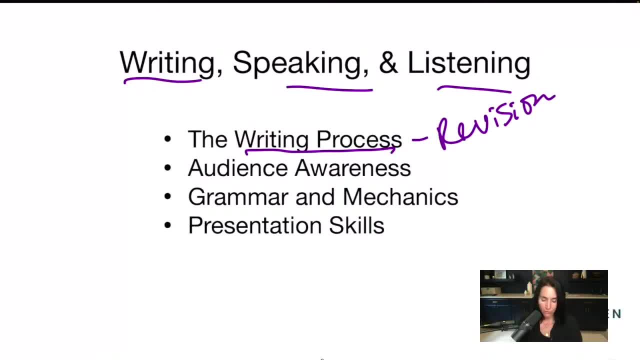 is going to be the correct answer. And for writing and speaking, audience awareness. Who's your audience? Who are you writing to, Who are you speaking to? This is also a skill we need to talk to students about If you are trying to. 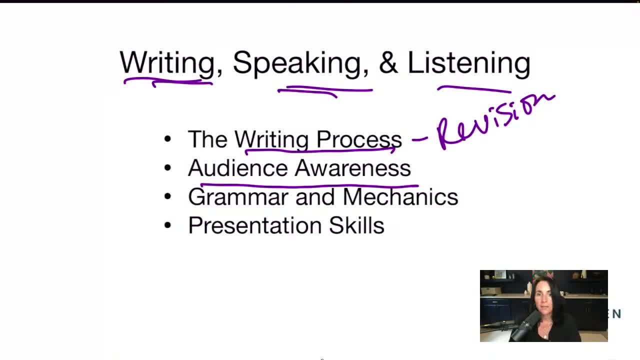 talk to the school board about a school policy. you're not going to write a narrative, right? You're going to write a persuasive essay to try to persuade the school board. So this you will see on the test. It'll probably have some sort of- you know, sample writing And it might say: 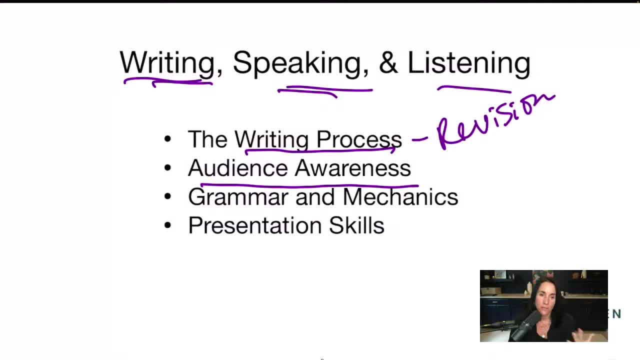 how can the student be better at this? And you might say: how can the student be better at this? And you might say: how can the student be better at this? So audience awareness is big, And then there's a little bit of grammar and mechanics in there. 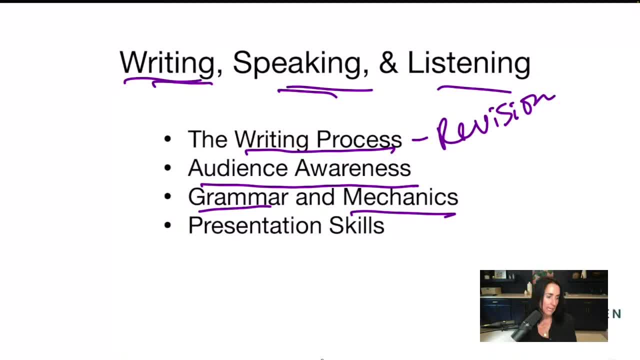 Not a ton, but you do need to understand the fundamentals of grammar and mechanics And I have that all in the book. It's a huge section And it's the basics: verbs, nouns, compound, complex sentences, punctuation- kind of those basics in grammar for elementary education. 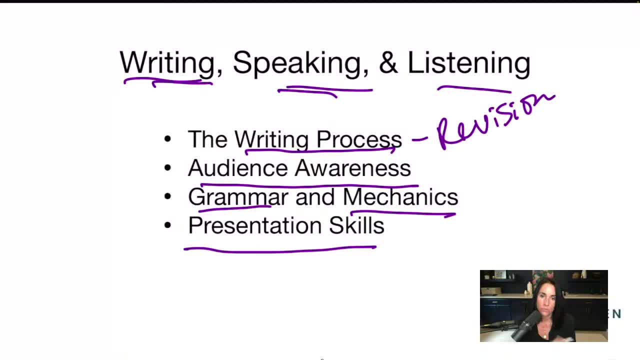 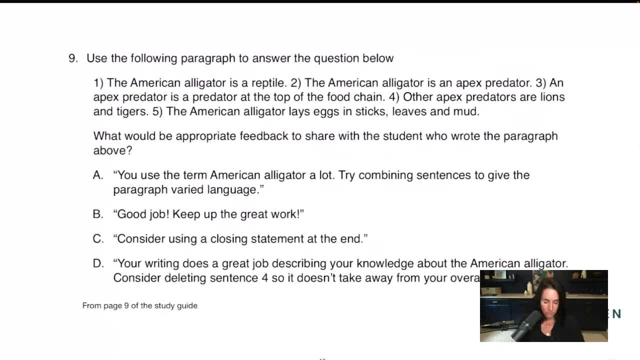 look at what a question might look like from the writing And again we have a big old question here which tends to give people agita. This is from page nine in the study guide, So if you want to turn to that And you can see most people start up here And that is not where I'm going to. 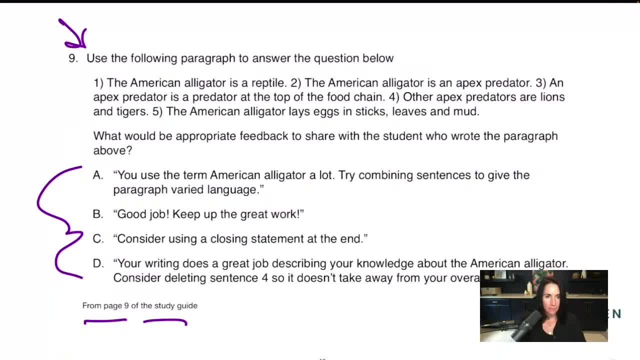 start. I'm going to start here And I might just peek in the question stem. And I'm going to start here And see the word feedback. All right, So let's have a look at A. You use the term American alligator a lot. Try combining sentences to give the paragraph varied language. Okay, 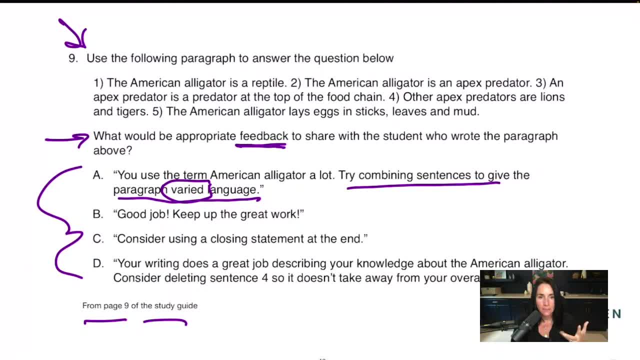 That's pretty good. It talks about varied language- Good word- And it's specific And I'm looking for feedback here, And so specific feedback is really good. So I'm going to keep A B Good job. Keep up the great work. Nope, Wow, That's a really nice thing to say to your students. 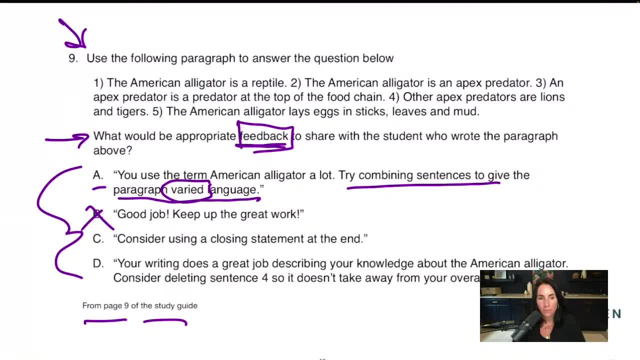 It's too vague. It doesn't give them any information on what they are good at and what they need to keep going on. That is not appropriate feedback, even though we use it all the time. But we're looking for appropriate feedback, Also called specific and meaningful. 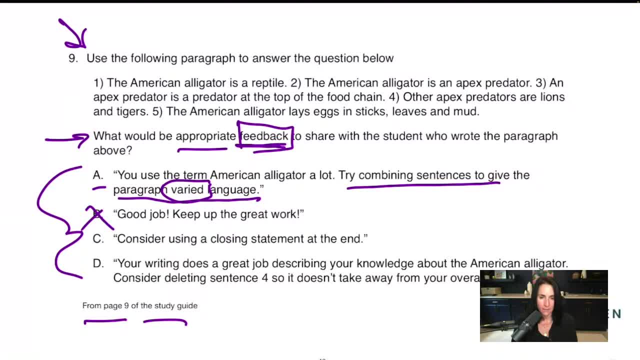 feedback C: Consider using a closing statement at the end. Okay, This is specific, But it's just like boom, here's what you did, wrong, Right. And so, in really good feedback, we want to start with the positive and then hit them with the this is what you need to work on, And then 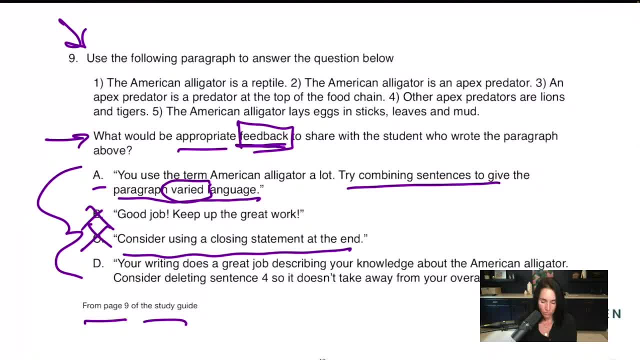 C- I'm going to cross that off. D- Your writing does a great job describing your knowledge about the American alligator. All right, So I said a good job, But I was specific about what is actually good. And then I say: consider deleting sentence four so it doesn't take away from your overall 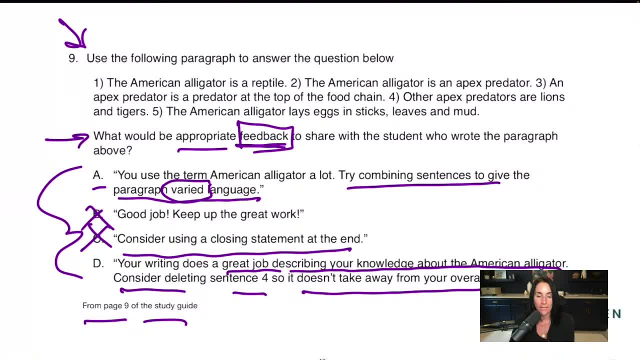 theme. Again, I give a critical analysis And I give a suggestion And I say: why? Why do you want to do that? So D is specific and meaningful. It beats out A. I don't even have to read the. 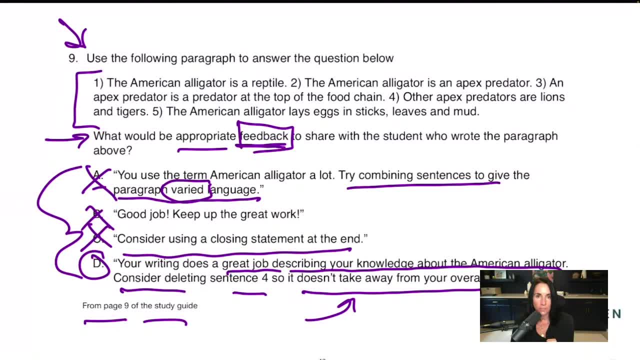 question. But let's have a look. We have a student writing sample here. He talks about the American alligator- the American alligator- And then we have this sentence here: Other apex: predators are lions and tigers- And it doesn't fit, And so we want to show the student to take that out, And that's why D is most. 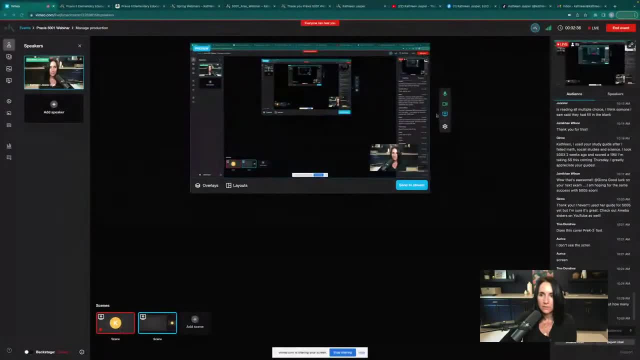 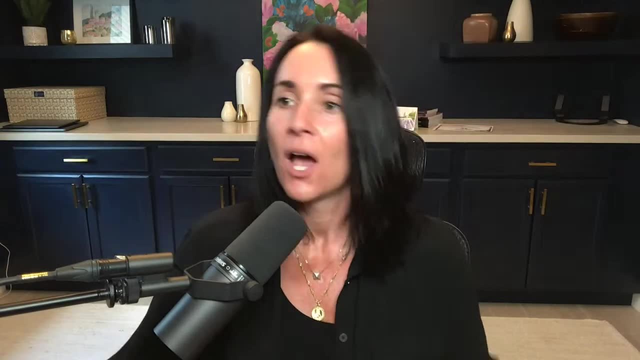 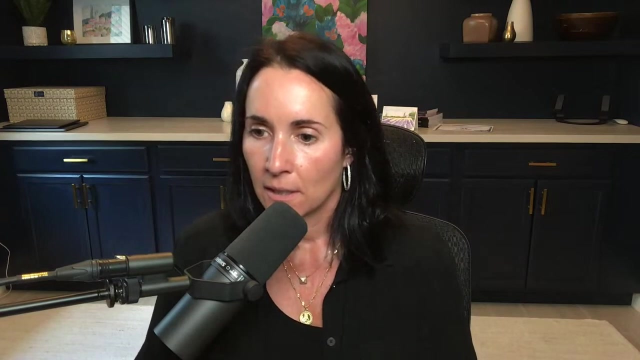 appropriate there. All right, All right, So let me stop sharing here And let's go back to here. Okay, So how are you guys doing so far? Let's see. Can you answer a question about how many syllables are in a word? It depends. 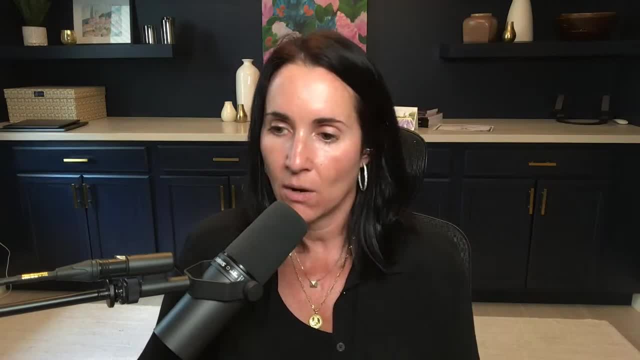 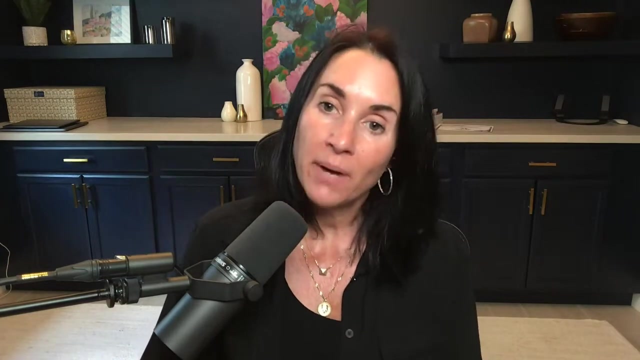 on the word And I can't really answer that right now. But you break up the word by syllables, by structural analysis. Is there a lot of questions about moving sentences in paragraph or deleting them? I struggle with those. Okay, There might be a couple of questions, So on this, 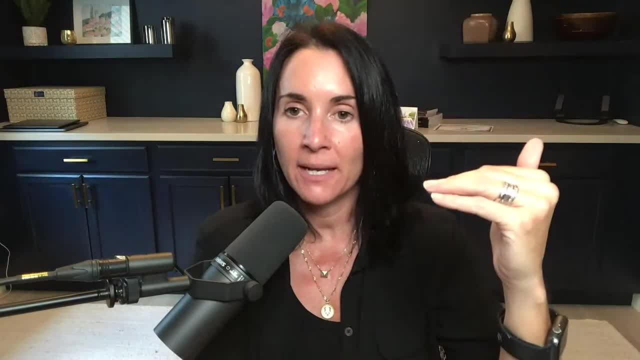 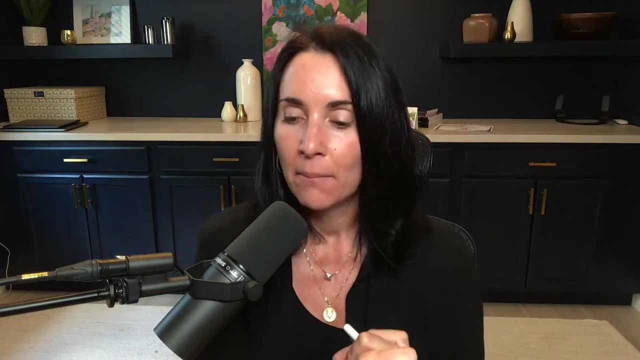 test. we have a paragraph that you have to analyze a little bit and see where you can delete and stuff like that. That's more prominent on the Praxis Core grammar section, But for this test you might have a piece of student writing where you have to do that, Typically a deleted sentence in a paragraph. 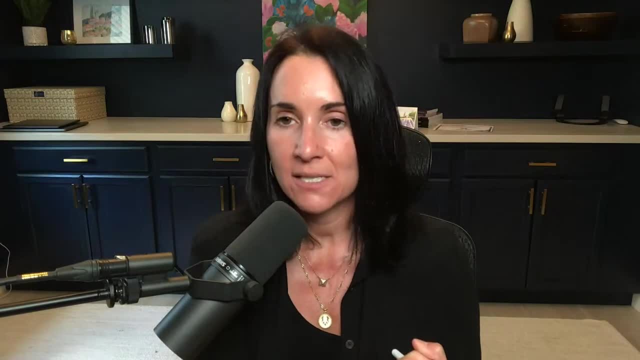 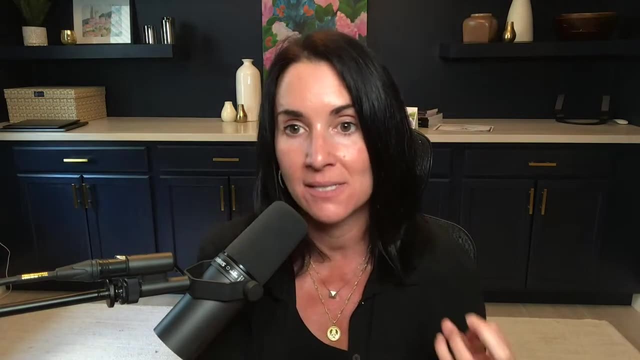 comes from, you know looking at something, and when it sticks out like a sore thumb, they want you to do that. It's not that ambiguous on the exam. Some of these are pretty. I mean, they're obvious to me because I study exams all the time. But you want to look for that. 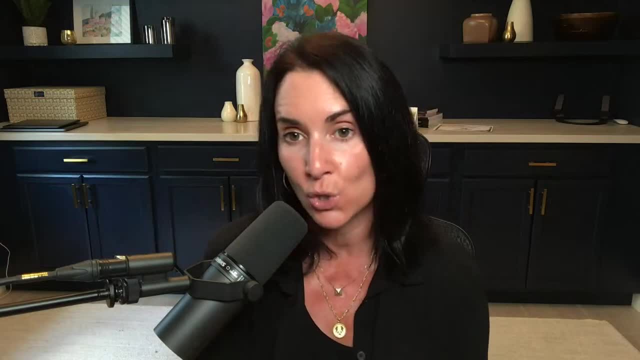 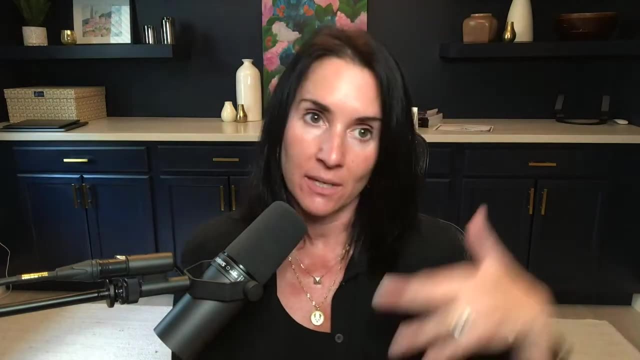 piece that is missing, But that's more of a. those are called rhetorical questions, And rhetorical questions are like this: If the author wanted to make this better, what could the author do? It's like rhetorical right. So those typically happen. on the Praxis Core writing test You might see one. 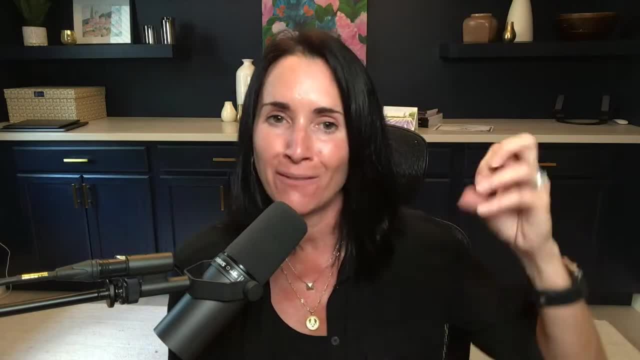 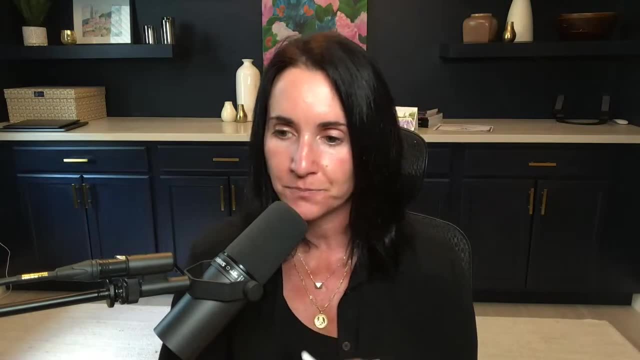 or two, but usually it's like the one I just showed you, where you have a student writing and then you have this glaring like random sentence in there and it's like, uh-uh, It's going to be pretty difficult. So that's what the student is doing wrong. All right, I wish you were my mentor. 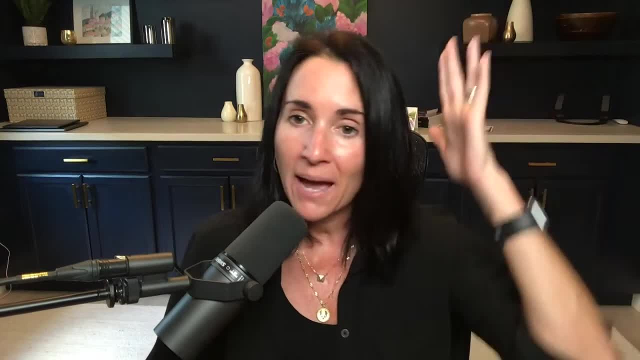 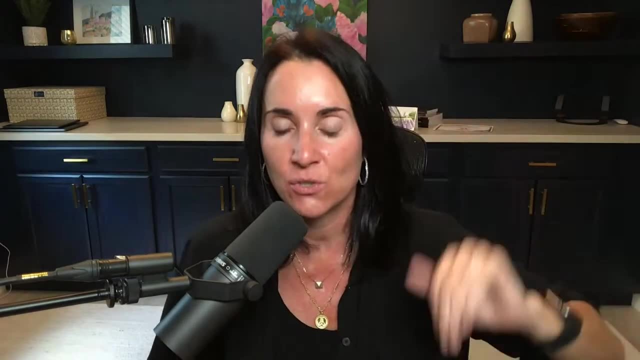 teacher. Oh, that's very sweet. Good Thank you for working backwards. Yes, work backwards, guys. Work backwards on everything, even if it's just quickly to look. But working backwards will help you get rid of those big long answer choices that you don't need to think about. Do you have a? 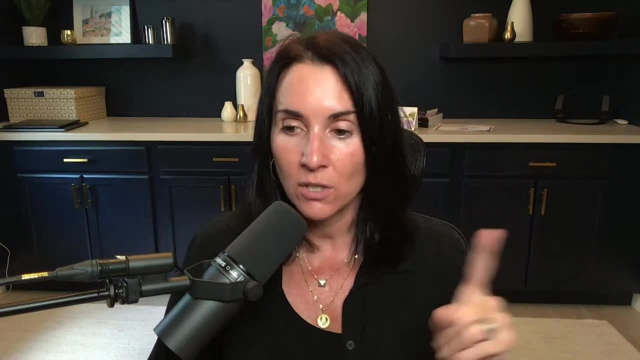 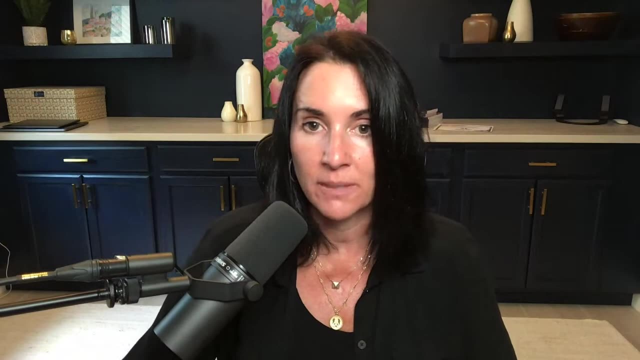 video on the stages of writing I do in the online course, So I'll talk a little bit about that in a second. okay, All right. So now let's move on to math, which is also pretty difficult. all right. 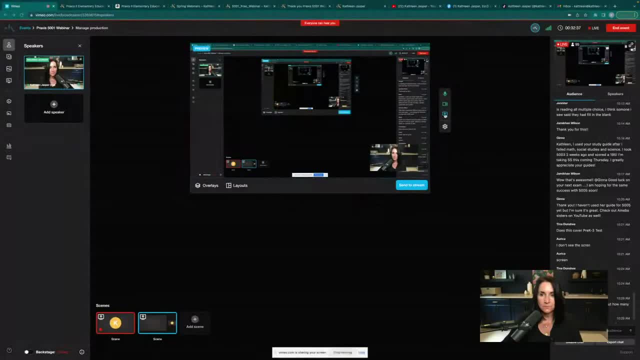 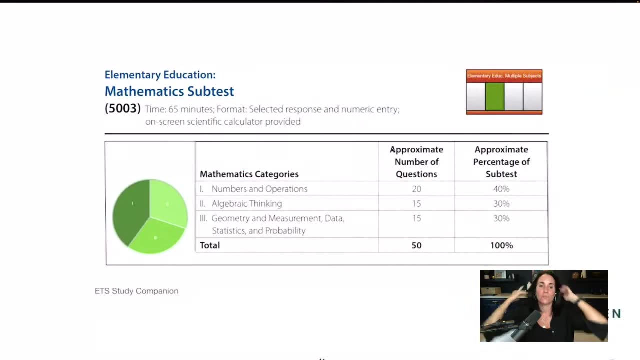 So let's go to the screen here again. All right, You see the math. Yes, you do, You see the math. Okay, This new webinar software. they don't allow me to just select the screen, So I have to do. 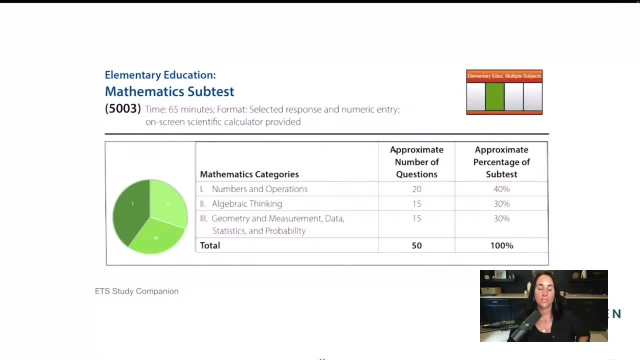 this infinity thing that I hate and I can't really see if I'm sharing. So I've already talked to them and asked them to add it as a feature, but we'll see what happens. Okay, So this is the mathematics subtest. This is 5003.. Oops, I just scribbled out my math. Hold on, And this is not. 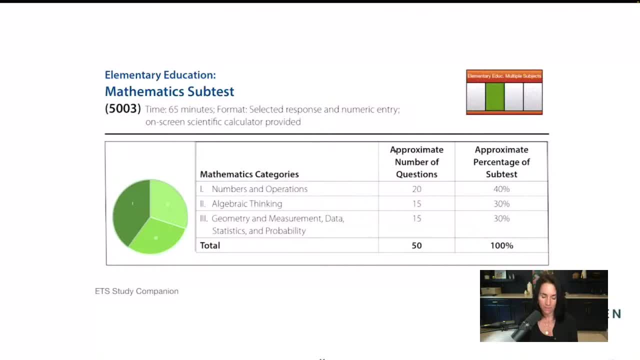 it. So most math exams, pretty much all math exams, have a numbers and operations section, algebraic thinking and then geometry, measurement, data, statistics and probability. Now, on higher level math tests, like for middle school or high school, they will section these out. But 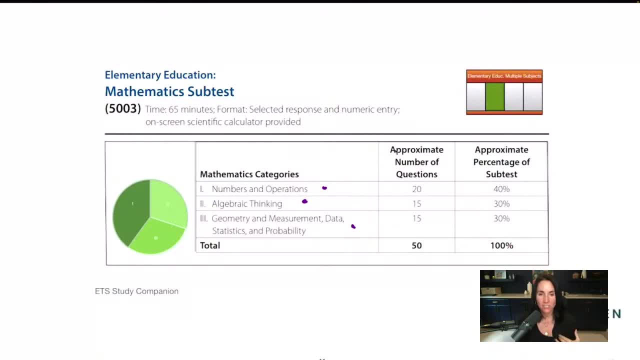 all math tests assess the same stuff. There's always an operations section, There's always an algebra section, There's always a geometry section, There's always a probability and data section And then, if you go a little higher, there'd be like pre-calc, things like that. But 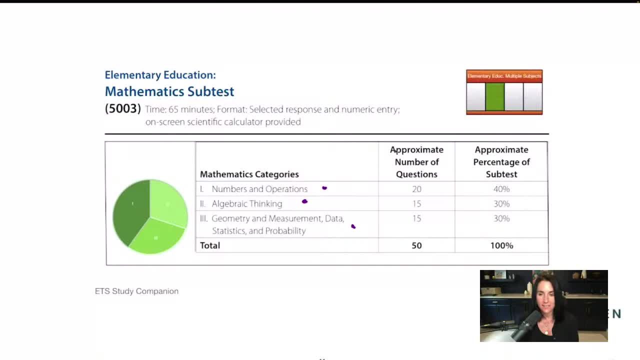 all elementary ed tests assess the same math skills. Now, on some elementary ed tests you have to figure out where the student made the mistake and how you would teach it. But you have to understand the skills themselves and be able to do the math in order to figure that out. 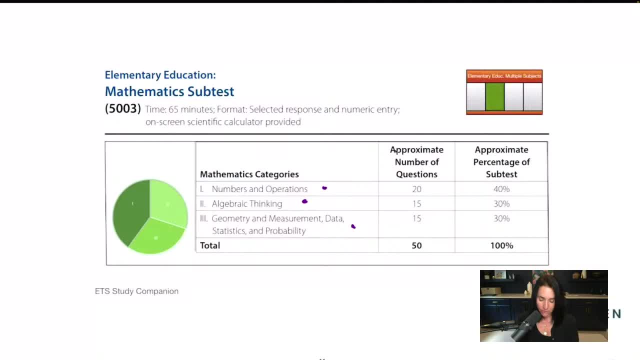 Okay, So we're going to talk a little bit about that today. Notice that the bulk of the exam for the math- 40%- comes from numbers and operations, And this includes all types of skills. I'm going to show you that in a minute. And then these two here are broken. 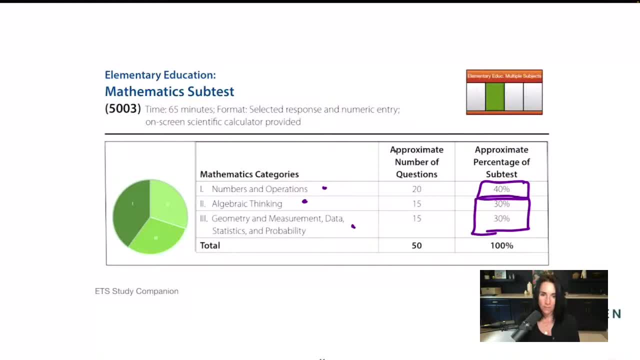 up the same 30%, All right. So really focus in on those numbers and operations. but you're going to have to understand all skills to get this And again, it's elementary but there's like some hard algebra on this. There's a couple about the coordinate plane. It's a tough exam. It. 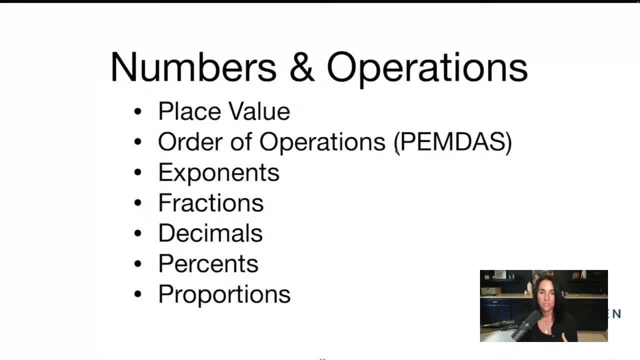 ain't easy, All right, So let's talk about numbers and operations. This is 40% of the math exam. It's huge. So you're going to have more basic things like place value. You might have even some things. 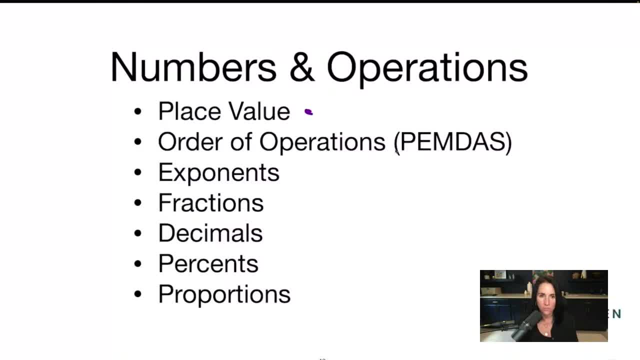 like number representation by like the number of blocks. how can we show that to students? It's going to be pretty basic, But then we get into PEMDAS. orders of operation, Parentheses: exponents, multiplication, division, adding and subtracting. 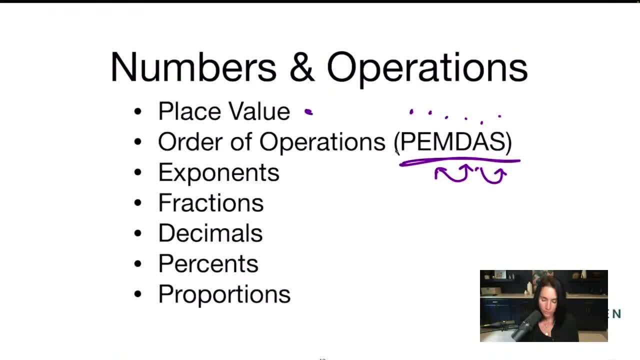 Remember these two can be interchangeable depending on which one goes first. I have a bunch of videos on that. But orders of operation, how do you solve these problems properly? You will have questions on exponents, fractions, which I know some of you cannot stand: decimals. 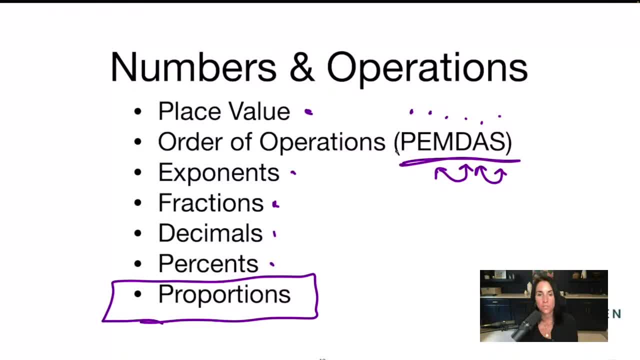 percents and proportions are a big one on the numbers and operations. So you're going to have to do some math in order to solve these problems. So I always say in my math videos that if you can do a proportion you can solve a lot of questions in the algebra section, in the geometry section. 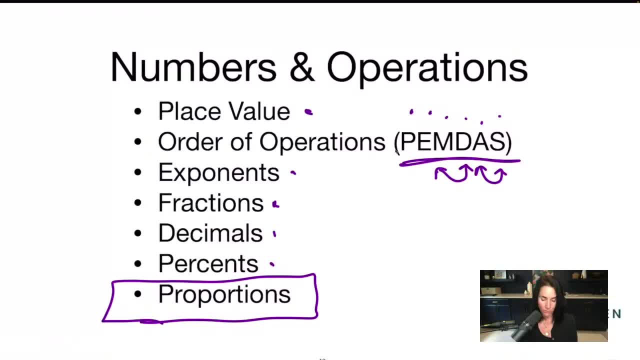 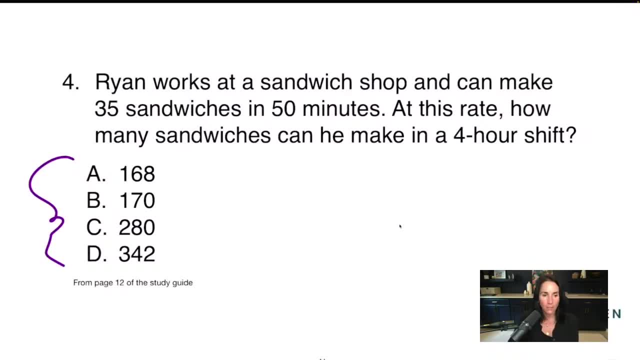 That piece of information and those skills is going to help you a lot. Let's have a look at a proportion. So if I'm working backwards I can see that A, B, C and D are just numbers, So I can't really do anything there. And let's have a look at the question: stem In math. 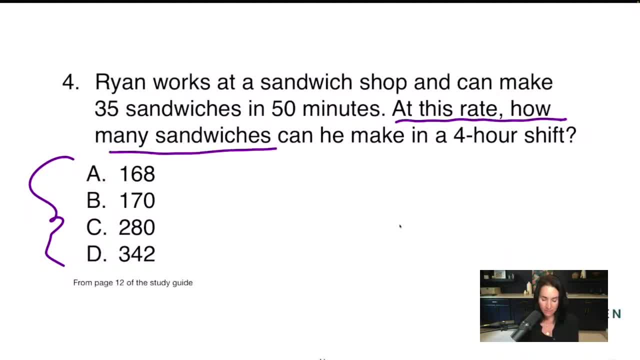 I always go to the question stem: At this rate, how many sandwiches can he make in a four-hour shift? All right, So I know right away it's a proportion, because it's saying at this rate, how many can he do? That's another keyword that it's a proportion. 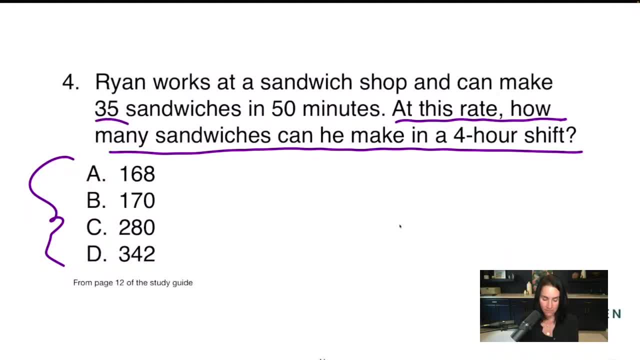 Now let's have a look up here. Ryan works at a sandwich shop and can make 35 sandwiches in 50 minutes. All right, So let's do it Matchy matchy: 35 sandwiches over 50 minutes. So 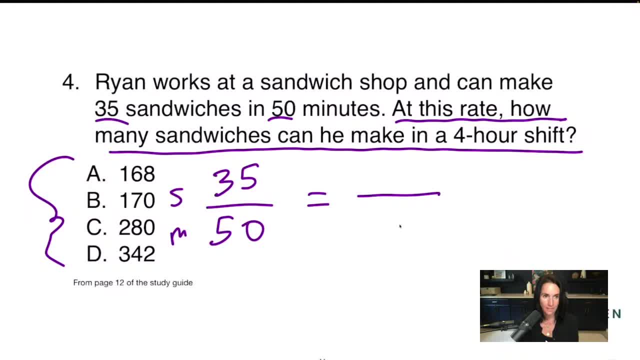 I have sandwiches over minutes, Okay, And for this one I want to do sandwiches over minutes. Well, it's asking me how many sandwiches. So I don't know how many sandwiches he can make, but it says can he make in a four-hour shift? 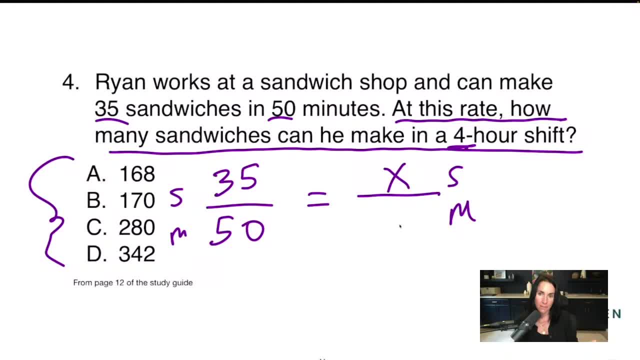 So he makes 35 in 50 minutes. How many can he make in four hours? Well notice, I have minutes and hours here, So I need to convert four hours into minutes. So I simply multiply four times 60 and I get 240.. Make sure you have matchy-matchy when it comes to your units And in this case, 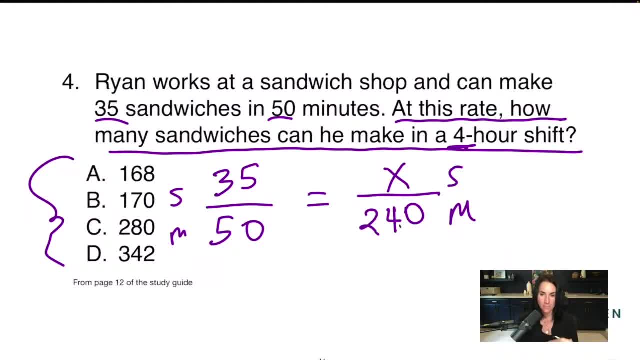 we want to keep it in minutes. It's easier that way. Otherwise 50 minutes is like point something, something of an hour, and it just becomes kind of annoying. So I just went to minutes here. So again, I have sandwiches over minutes. equals sandwiches over minutes. Same on the top. 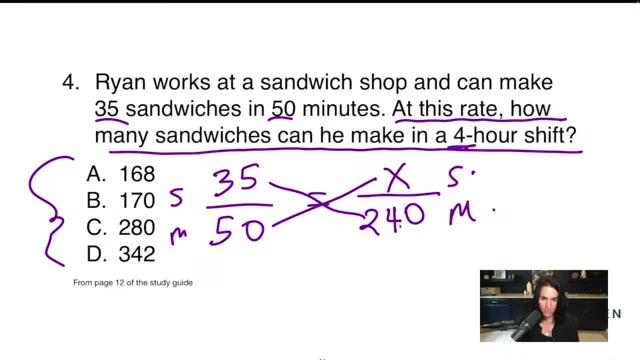 same on the bottom Matchy-matchy. Now I'm going to cross, multiply and solve. I have 35 times 240, and I get 8,000.. There we go, 400.. So I'm cross multiplied these two. 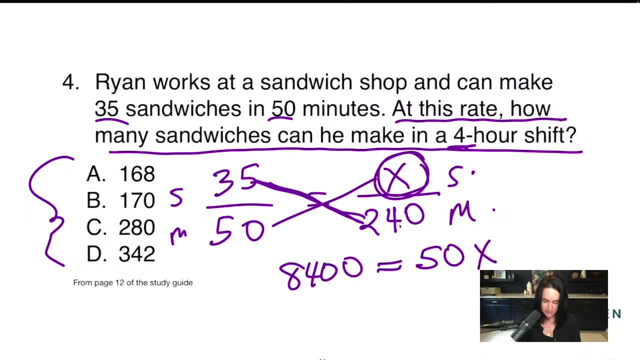 400 equals 50x. All right, Cross multiply here. Cross multiply. So then I divide by 50.. Divide by 50. And 840 divided by 50 is 168.. The answer is A. All right. So again in this question. 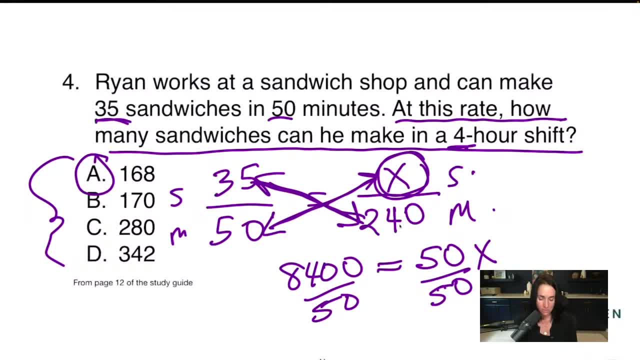 you can see we have three out of the four things. I have sandwiches and minutes and I need sandwiches and minutes but I only have here. I have hours but we turned it into minutes. I need to figure out that fourth thing, the sandwiches. I set up my proportion matchy-matchy, I cross. 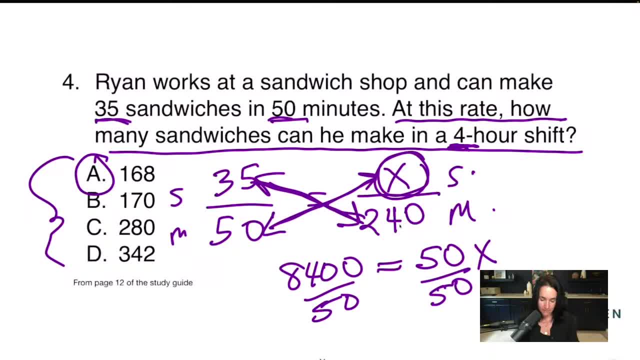 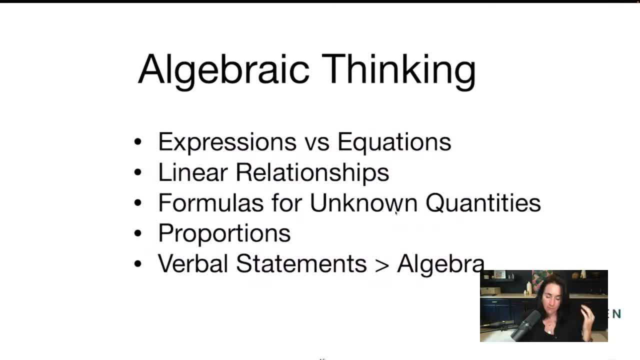 multiplied and I got 168.. Okay, All right. So now let's go to algebraic thinking. Algebraic thinking can be pretty tough. You're going to have to work on expressions and equations, linear relationships, formulas for unknown quantities. Again, proportions are in the 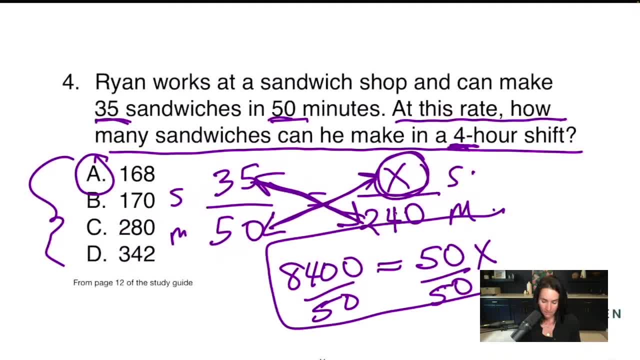 algebraic thinking. Notice that if I go back to here algebraic equation, It's part of numbers and operations, but I had to use algebra to solve it, So a lot of these things are intermingled when it comes to your skills. So be on the lookout for 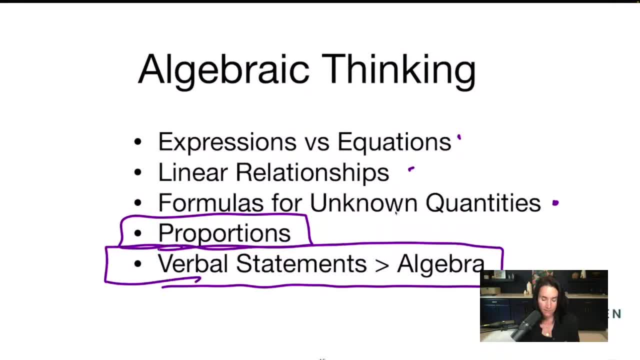 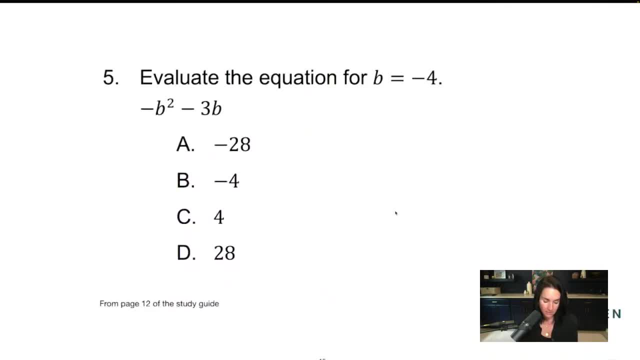 that, And then turning verbal statements into algebra. People tend to have a hard time with that- where it says: you know you get a word problem. you have to turn it into an algebraic equation. It's not easy. Well, what might this look like on the test? Well, let's just have a. 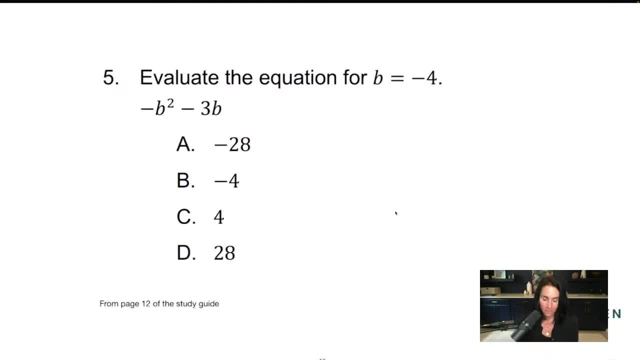 look at this algebraic equation. I mean this is elementary, This is hard. This is on page 12 of your study guide, All right, So I mean this. to me it feels tough for elementary. I don't remember doing this in elementary school, But of course, 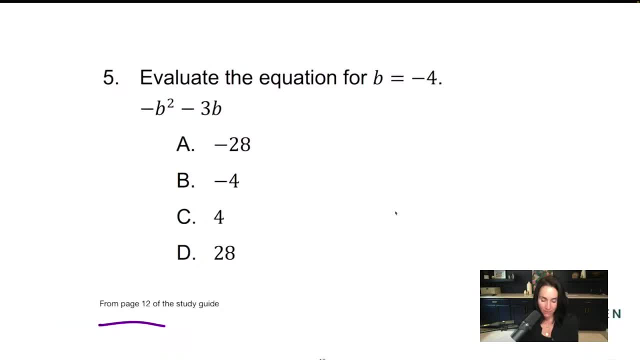 the standards have gotten higher for kids. So we have evaluate the equation, for B equals negative four. Okay, So we have. we have the B here. So what we need to do is we need to input this negative four everywhere we see B, So let's just write it out. So I have, I have room here. 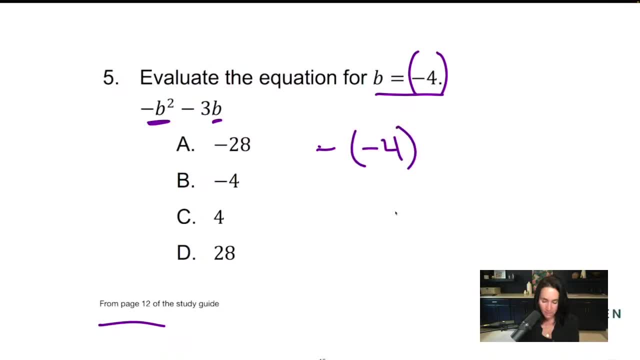 negative- and I'm going to put this in parentheses: times negative four squared minus three. times negative four. Now we got a lot of negatives, and this is where people get messed up. I was just going through this with my daughter. Remember your negatives, Check for your negatives. 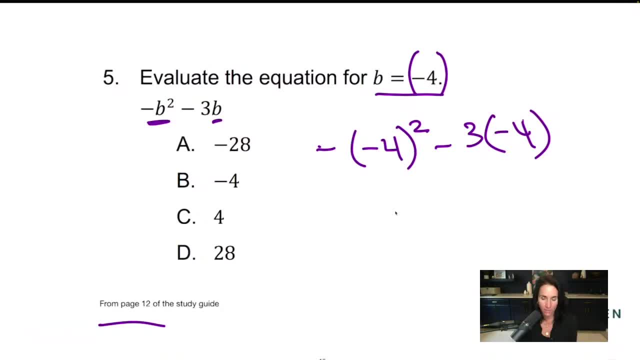 because on standardized assessments they always do this. They put a ton of negatives. all right, So if we're working in PEMDAS, all right, we could do the parentheses first. You could move this through here. But this is actually multiplication, because you're multiplying by a. 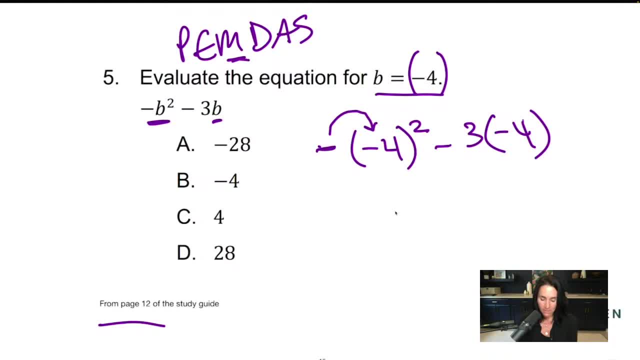 negative one and that would be here. So I'm going to go ahead and do that. I'm going to go ahead and be here, because this is essentially this negative is a negative one, okay, so we're not going to do that one first. oops, let me go to my eraser. we're going to do the exponent first, because that's my 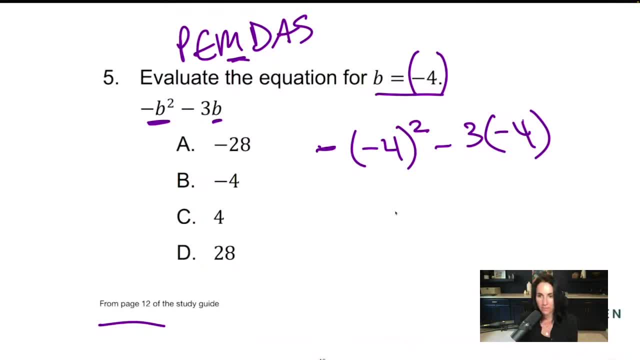 next thing in the equation. yes, there are parentheses here, but that's only to separate the items. when we talk about parentheses, we're talking about things like something like that that's holding a big part of it. okay, now, that's not part of this particular question, so i'll go ahead and erase it there. but let's do the exponent. that's my next order. 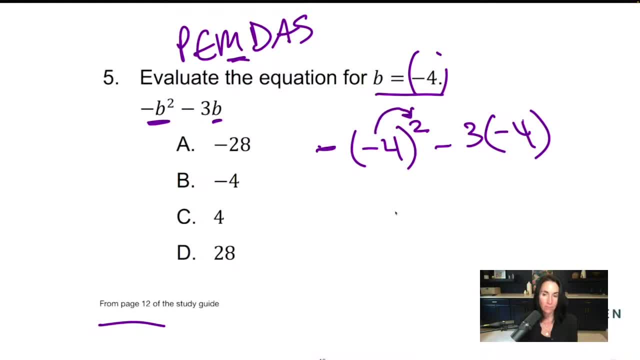 of operation and i have negative four to the second power, which is negative. four times negative, four negative times a negative gives you a positive. okay, let me just- i like to, when i'm demonstrating this, take it one step at a time. okay, now we can do the multiplication. so, essentially, 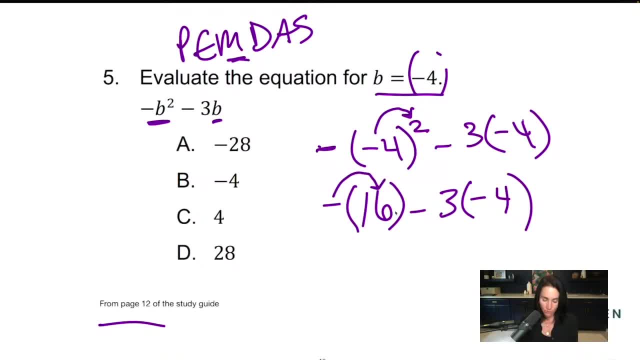 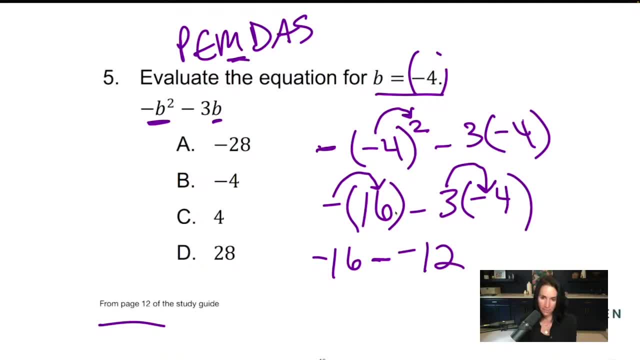 get freaked out when they see negative. minus a negative. anytime you see minus a negative, this turns into plus a positive. all right, so we have negative. 16 plus 12 is going to be negative. 4b is the answer to that. so we're going to do the multiplication. so let's go ahead and do the. 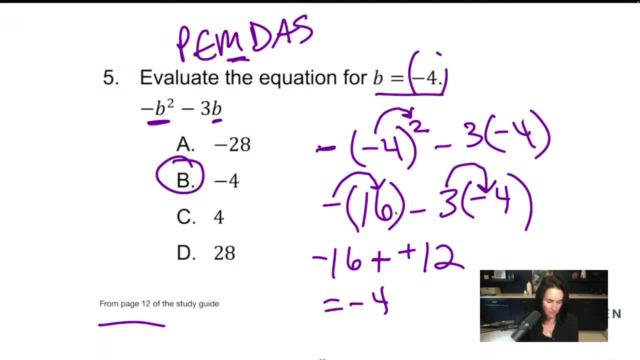 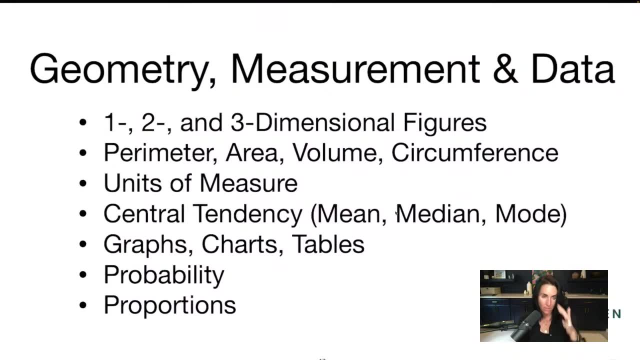 multiplication. so let's go ahead and do the multiplication. so let's go ahead and do the answer there, all right? all right, let's have a look at geometry, measurement and data. this is a big section as well, and it covers a ton of stuff, because not only do you have 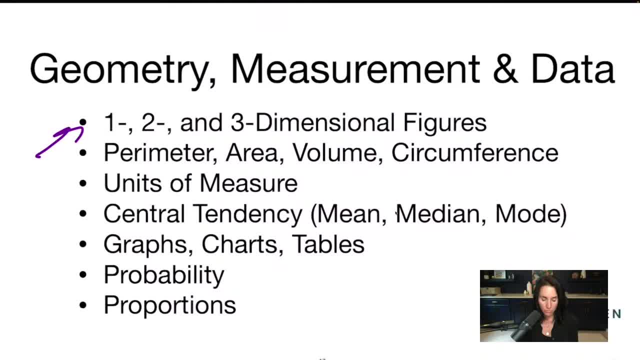 geometry. but you have all that probability so you're going to have to know one, two, three dimensional figures: perimeter, area, volume, circumference- there are a little bit of circles on there. units of measurement meaning meters to kilometers, things like that central tendency, mean median and mode. that's a big part of the probability portion. 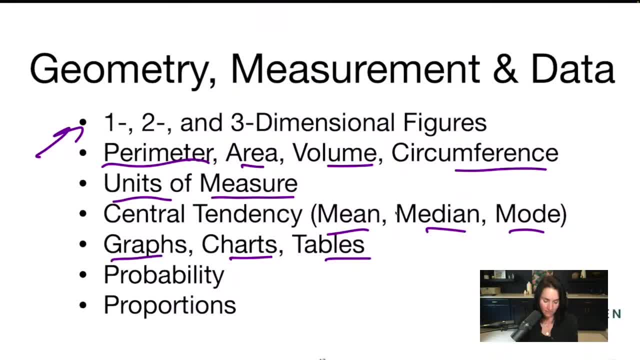 you're going to have to evaluate charts and graphs and tables again. we have proportions. you will use proportions to solve these problems as well and you have that probability. what's the probability of rolling a six? what's the probability of choosing a blue sock? what's the probability of you? 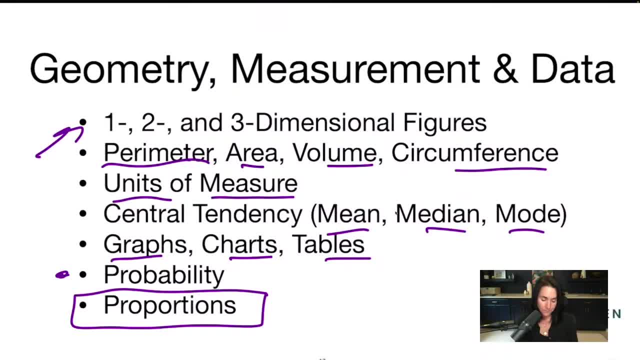 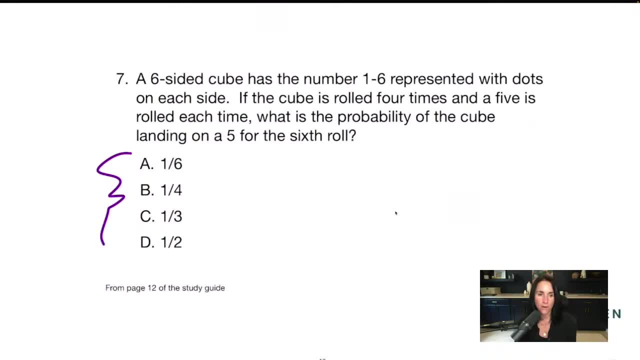 know whatever. so those will be usually in a word problem and I have one right here for you, all right? so I see in my answer choices that I have some fractions and let's have a look at the question stem. if the cube is rolled four times and a five is rolled each time, what is the probability of the? 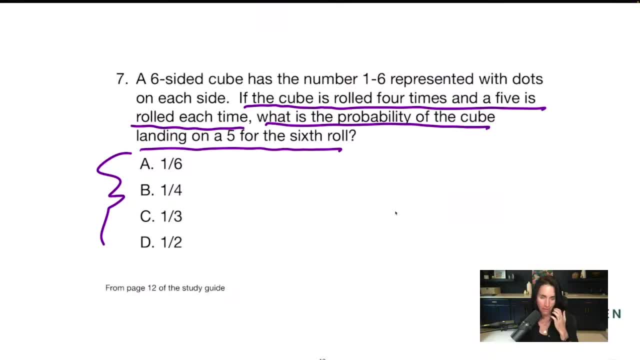 cube landing on a five for the sixth time. okay, so we have a cube, let's go up here. a six-sided cube has numbers one through six, so it's a. it's a die all right, with dots on each side. so this is a die. I have one of them, not two. one if the cube is rolled four times and five and a five is rolled. 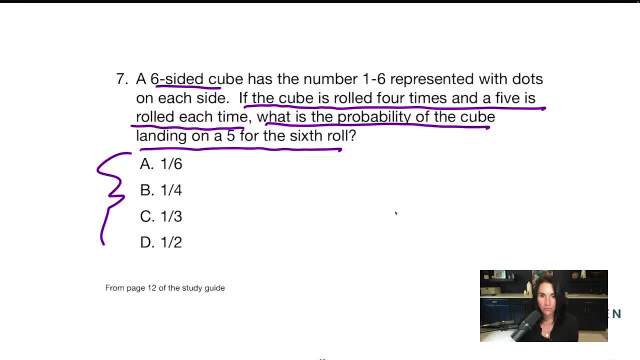 each time, what is the probability of rolling another five? the probability of rolling a five change. there are six possible outcomes, because there's a one, a two, a three, a four, a five and a six on a die and to roll a five is one pos one possibility, one over six, it doesn't matter. 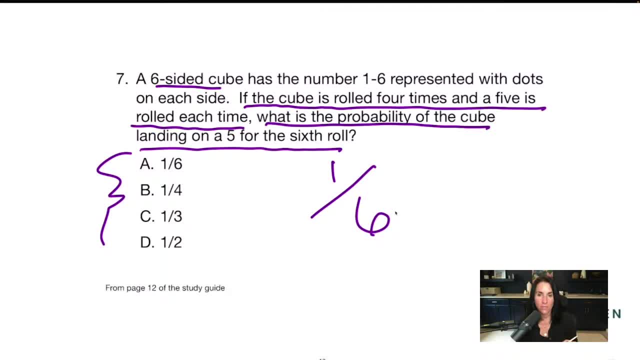 how many times you roll it. it doesn't increase your probability. you still have a one out of six chance of rolling a five. all right, so a is the correct answer there. I go into probability in depth in the book and in the online course, so if you struggle with this, you're not alone. a lot of 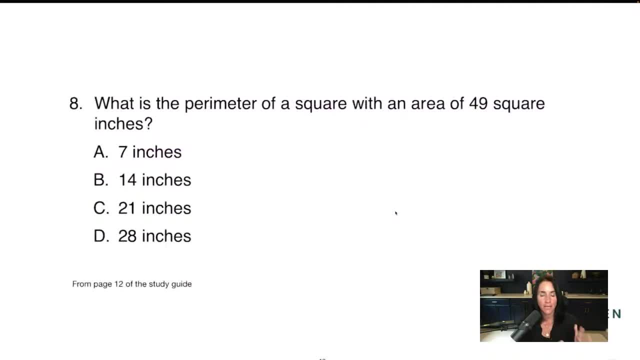 people struggle with the probability, but it ends up being pretty easy once you have an understanding. all right, we've got some geometry here, perimeter, and I have these answer choices here. I'm not sure what I'm doing here, but let's have a look. we can see, though, that it's all in, if I really wanted to. 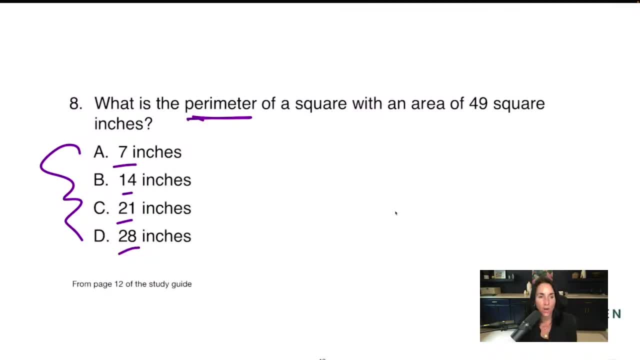 be. think like a test maker, which I try to do. you can see that they are all in sevens: 7, 14, 21, 28. all divide can be divisible by seven. so that gives me a clue. what is the perimeter of the square with an area of 49 inches? again, this is in units, and of Seven, and also, if you had some, 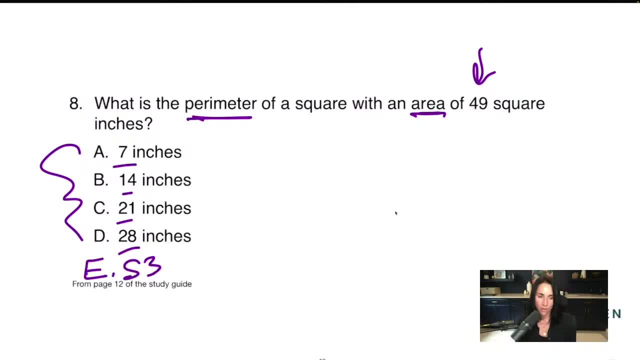 outlier here, like E, is 53, you would know that probably E is not going to be working out here because we're all in Sevens. so just a little quick advice there. this is not part of it, but if you had some weird number it's probably not going to be the answer. so anyways, let's have a. 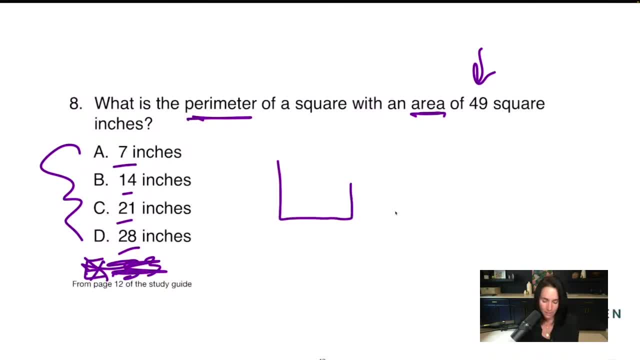 look, so we have. we're looking for the perimeter, but we only have the area. Square is four equal sides and we know the area equals 49.. Well, if it's a square and all sides are equal, what times? what equals 49?? 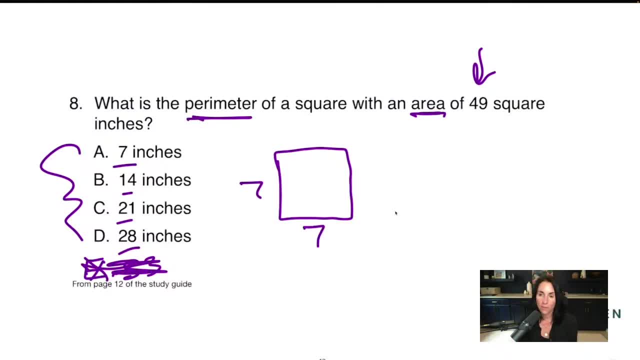 Well, 7 times 7 equals 49.. Well, I'm not looking for area, I'm looking for perimeter, which means all of the sides- because it's a square- are 7. And so I add all of them up, or I can multiply 7 by 4, and I get D 28 inches there. 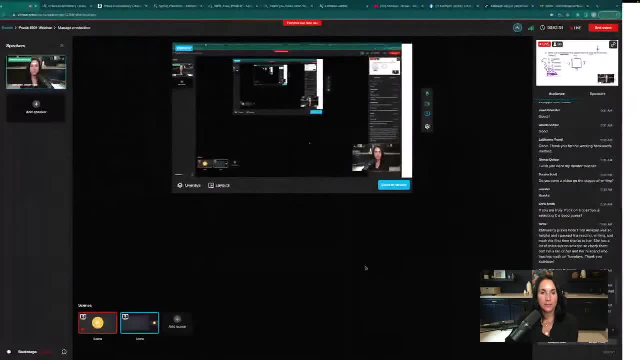 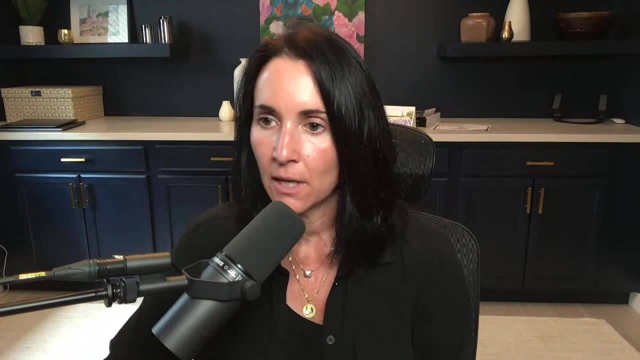 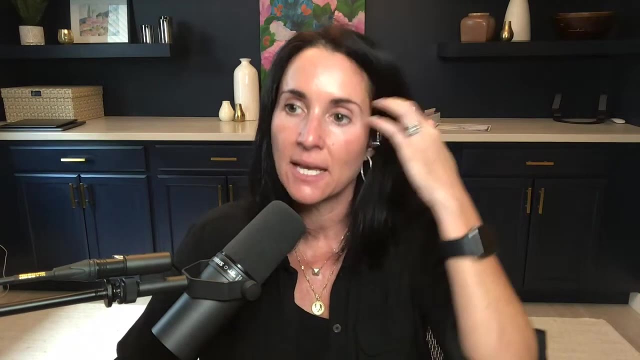 All right, All right. so let me go back to my presentation here. see how you guys are doing. All right. If you are truly stuck on the question of selection, see a good guess. I can't see which question we're talking about. 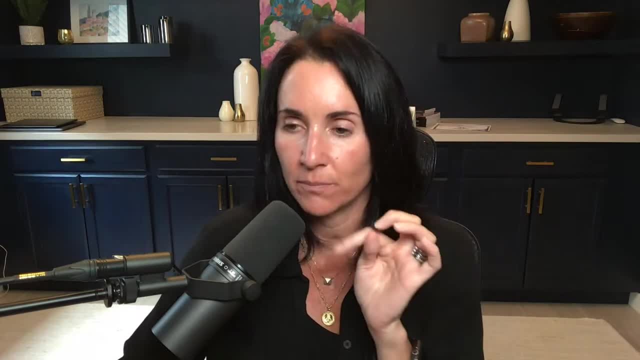 Chris, sorry I was sharing my screen. I can't see the comments. So if you want, you can put in a little comment and I'll try to figure out what you're talking about. Kathleen's practice book from Amazon was so helpful. 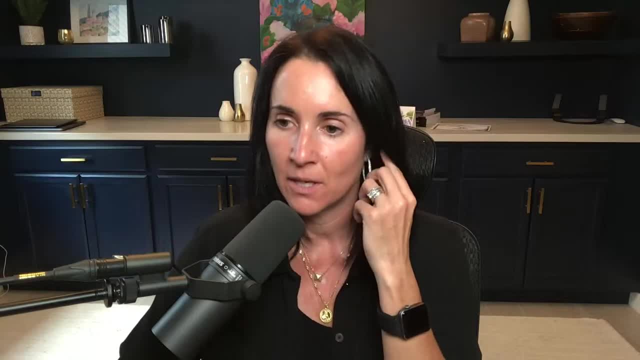 I passed the reading. I passed the reading, writing and math the first time. Awesome. Do you tutor individually? No, I don't. You can see there's 100 people on this webinar, 1,000 people signed up. 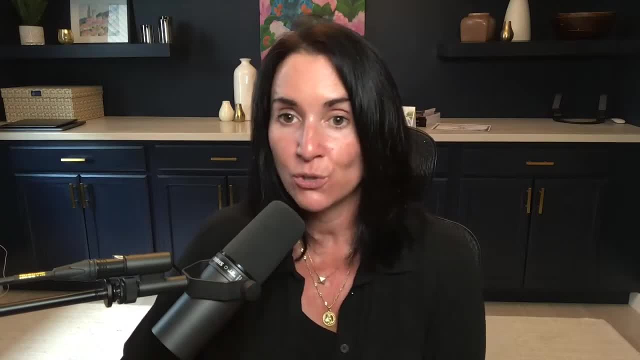 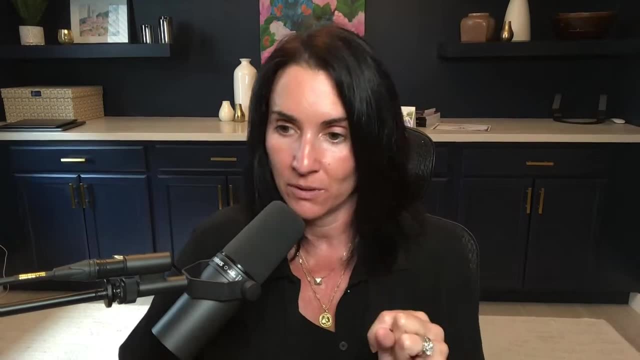 I just don't have enough hours in the day to do individual one-on-one tutoring, but my online courses are very, very comprehensive and I'm there with you for every problem. I go through every problem in the book. Did I miss the writing portion of the reading? 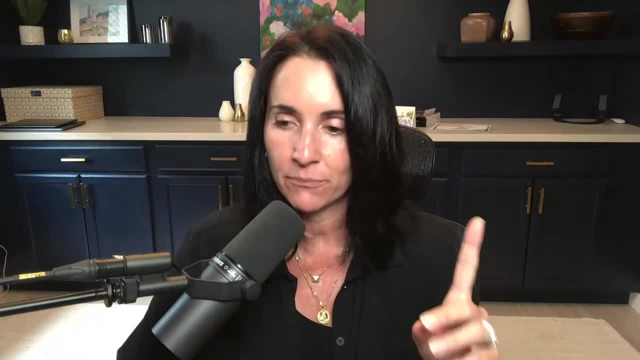 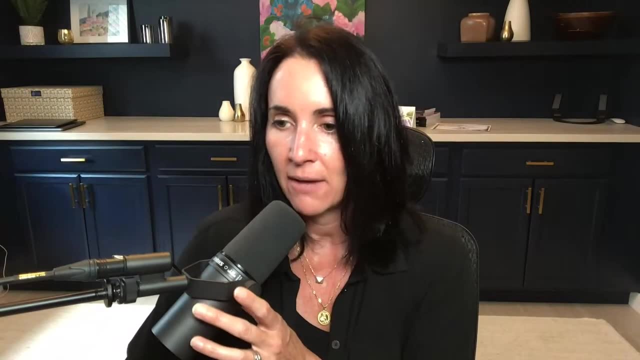 Did you cover it? Yes, I did. It was just a few minutes ago. I'll jump back to that: How to prepare for the math when you have math anxiety. Okay, so a couple things about math. A lot of people have math anxiety. 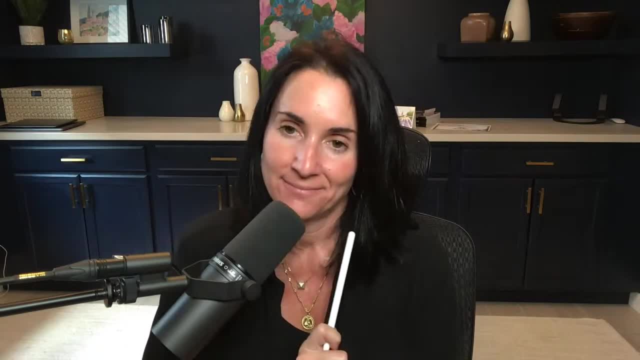 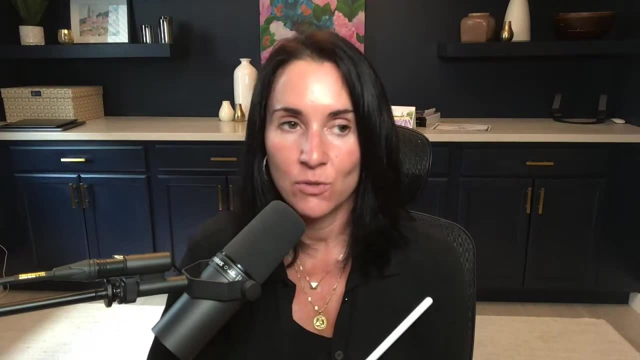 I get it. You have to challenge that thinking because you're going to be teaching students and they're going to have math anxiety And we get this in our head. I'm a reading and language arts person. I'm not a math person. 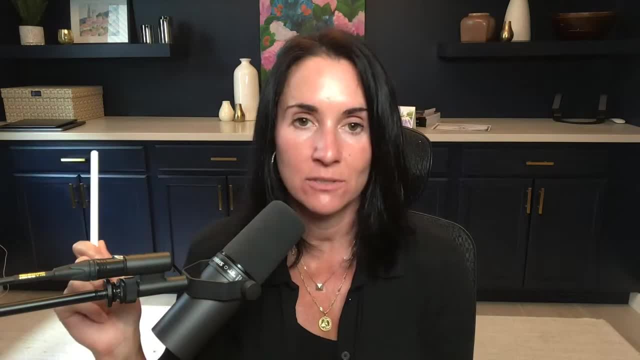 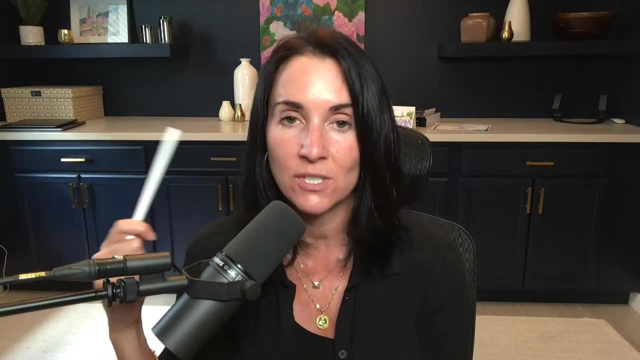 That's not true. You're a math person. You just have to practice your math. The way you do that is by really understanding the concepts and skills and challenging that voice in your head that says: you suck at math. You don't suck at math. 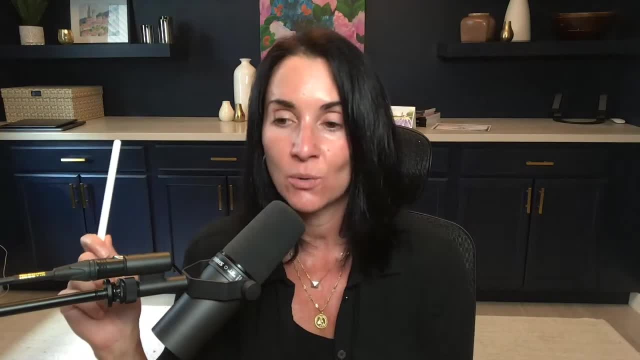 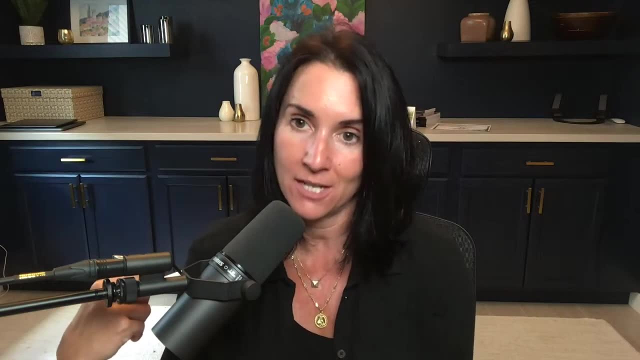 You just haven't practiced it enough. Everybody can be good at math, So I'll give you an example. I thought I was a reading and language arts person, and then I got chosen to teach biology in high school, and biology was my worst subject in high school. 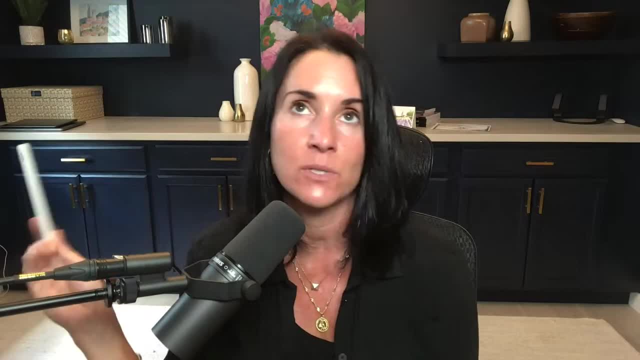 I thought I was not into science and I didn't like it. It wasn't my thing and I was a writer and I was. you know, that's what I studied in college. no, I'm not a biology person. 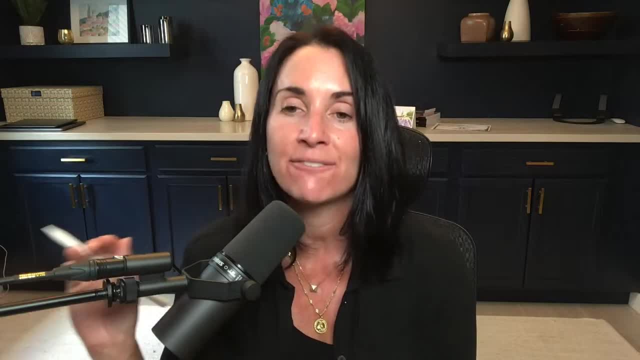 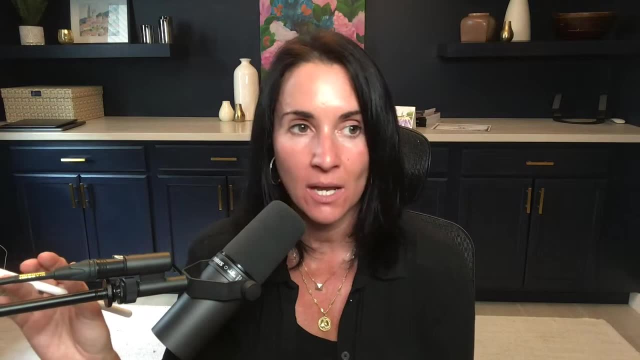 When I got thrown into the fire and became a biology teacher, I fell in love with it because I had to relearn it, because I was teaching it and it was amazing, And so there's always time to relearn these skills and to practice them. 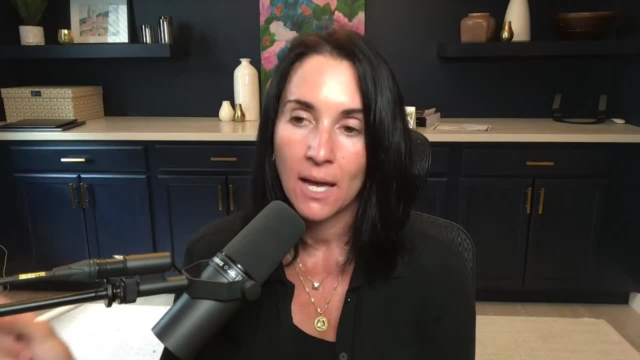 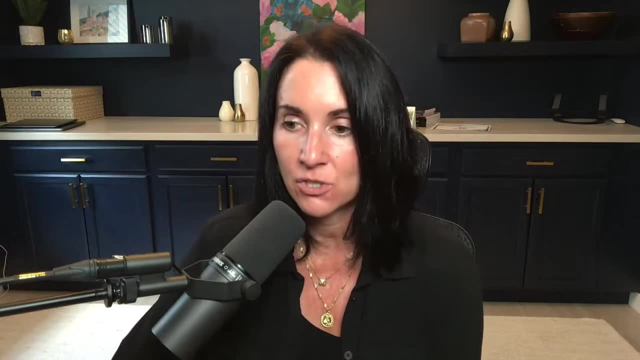 So I would check out my math YouTube playlist. If you need more help in this area, I have an online course, but you've got to challenge that kind of negative self-talk about math and because your students are going to do it too. 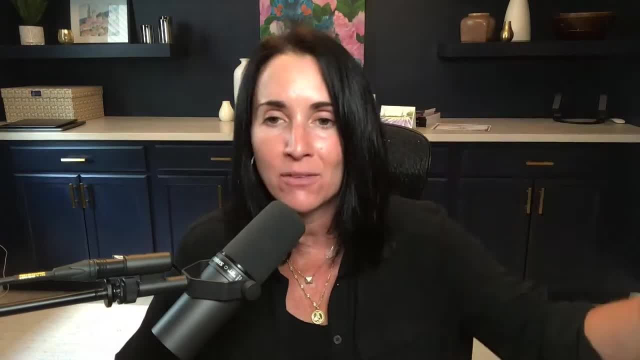 and we don't want them to do that. You want to be well-rounded. You want to be a good teacher. You want to be a good teacher. You don't have to be a math genius, but you've got to challenge that thinking. 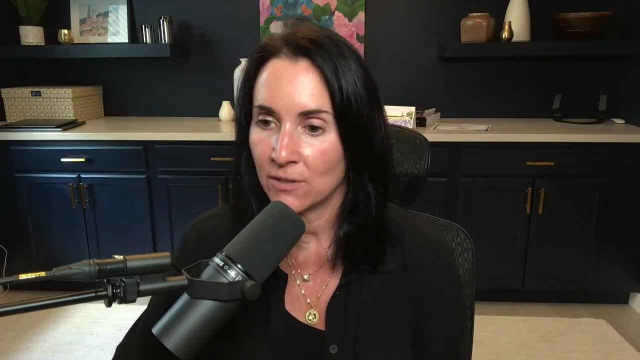 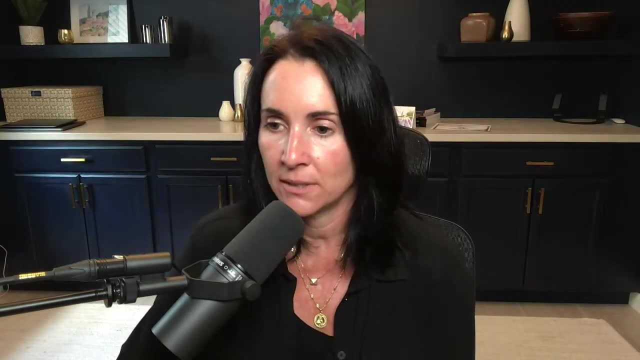 Say something different to yourself. okay, YouTube videos have helped. awesome Butterfly effect when multiplying. yes, I'm sorry, I messed up that proportion. Live TV: you know how it is. Are we able to use a calculator on the practice exam? 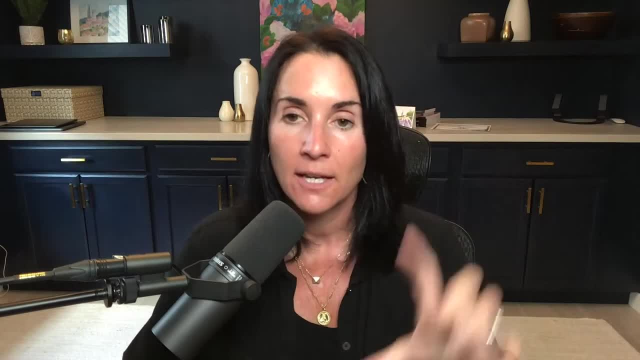 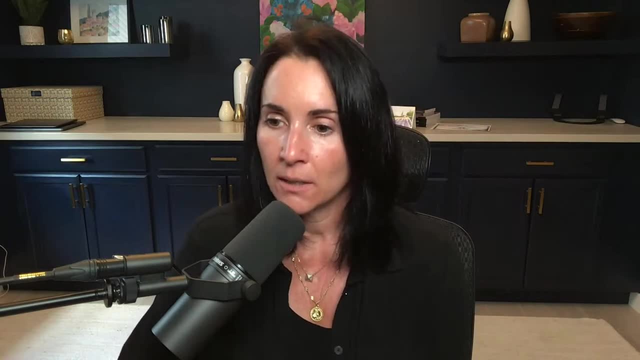 Yes, you can use a four-function calculator on this test. It's on screen, so be real careful when you input it in. but yes, you can use a calculator. They have a calculator, Let's see. Yes, I got this question correct. 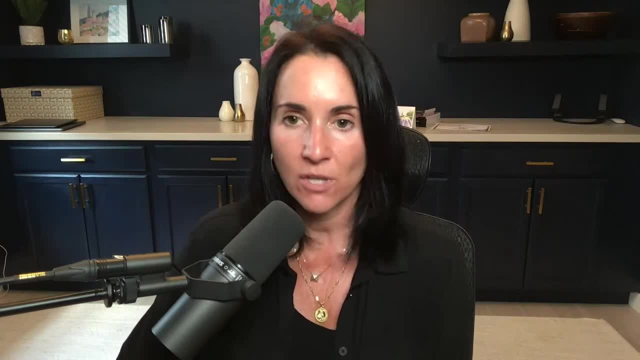 Good, I'm in Texas. How similar is the test to Texas? This will help you with the EC6 in Texas. Laura, I am taking for Missouri. How does this work? I'm not sure which test you're taking for Missouri. 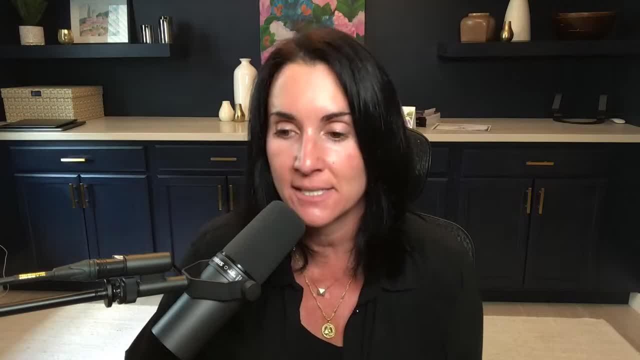 I'm not sure if it's the 5001 or another, but if it's an elementary ed test, this is going to help you. And again, I'm in Texas. yes, Texas, it will help. Okay, What time is it? 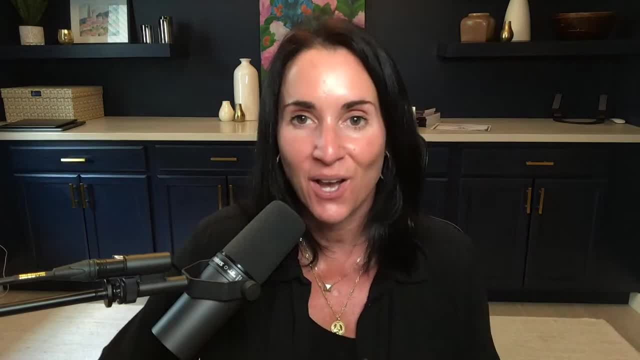 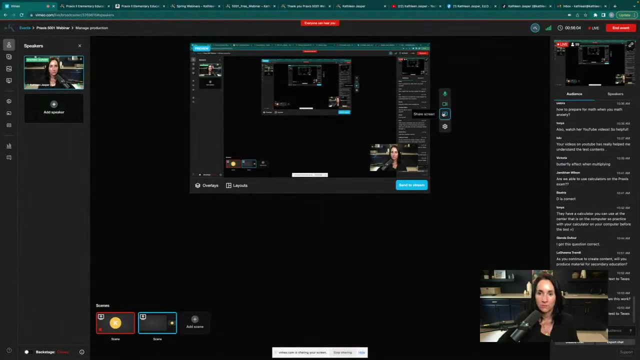 Oh my God, We've got two more sections. Let's keep moving. All right, guys, here we go. Now we're moving on. I always go way too long. All right, We should be able to be here, Okay. 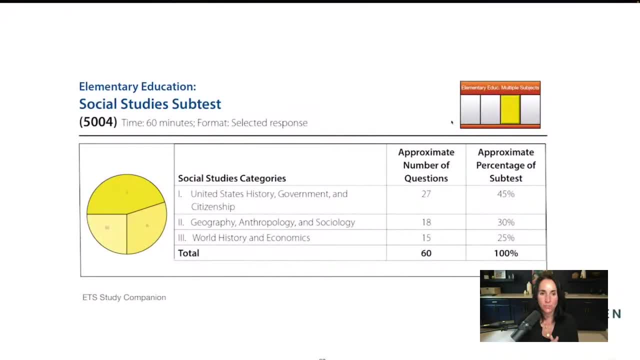 So let me just make sure again, You can see it. Yes, you can. Okay, So now we're in the social studies section. Not as difficult as the math and the ELA. This is more of like just memorizing random social studies stuff. 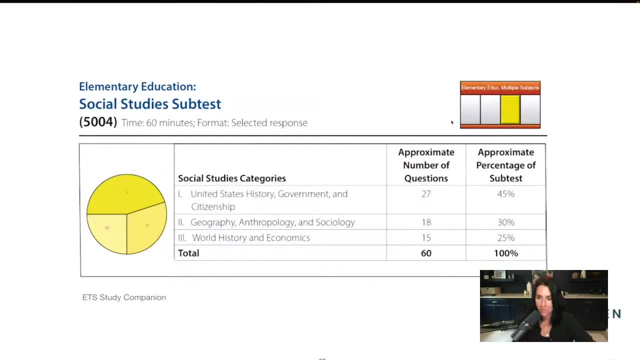 If you haven't taken a social studies class in 20 years. you got to brush up on this stuff. It's going to ask you about the branches of government. It's going to ask you about the Bill of Rights. It's going to ask you about the War of 1812.. 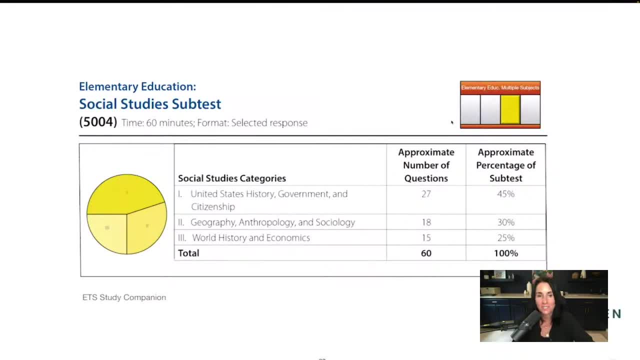 I mean just Just things. you have The potato famine, You know. these are things we don't normally think about. all right, So if you haven't taken a social studies class in a while, you're going to really need to. 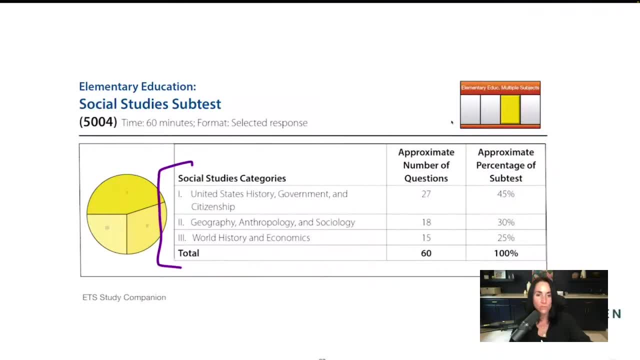 brush up on this. So again, there are three sections to the social studies exam. All social studies tests assess US history, government and citizenship, geography, sociology, world history and economics. All social studies tests assess this. Now, as you get up in the higher grades, like I mentioned, with math, you will get more specific. 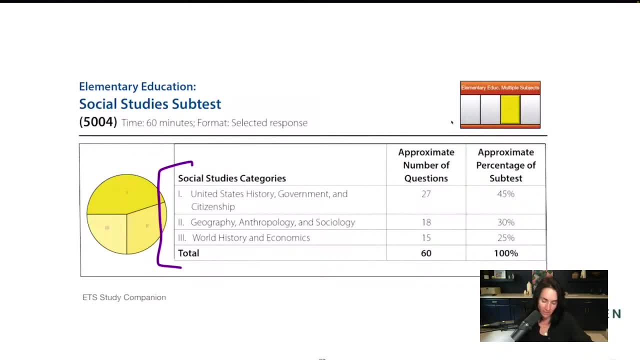 But These are the ones that you get on your last year's science exams. These are basically the The classes within the social studies department. If you went to a high school, there's a US history class, there's a government class. 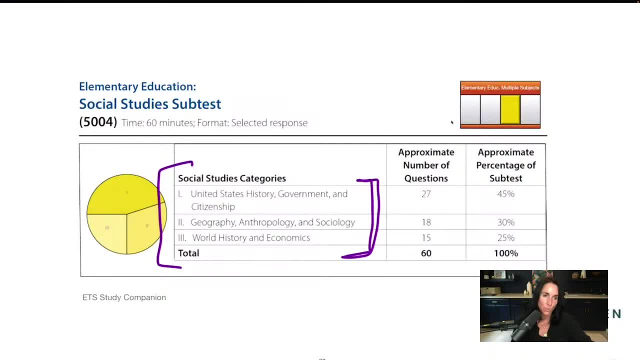 there's a geography class, that kind of thing. So these are all the disciplines within social studies, right, And you can see the bulk of it is going to be on US history and citizenship, but there is going to be a little bit on econ. 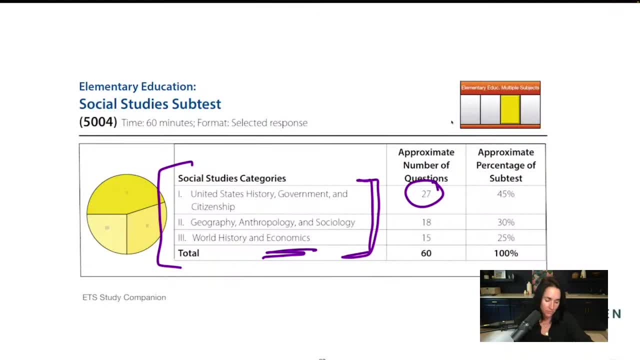 There's some tough economics questions on this test, So we want to make sure we understand that. So let's have a look at US history and government and citizenship. You are going to talk a little bit about US history and government and citizenship. 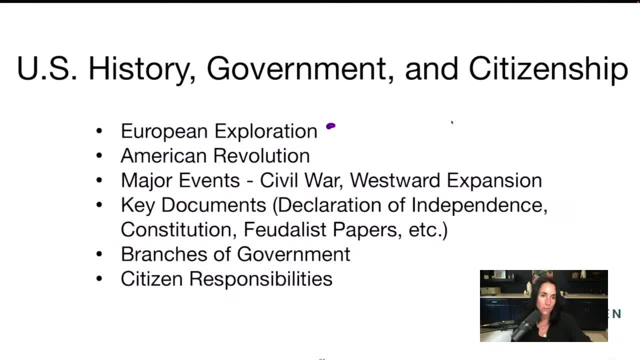 You are going to talk a little bit about US history and government and citizenship, european exploration of the americas here, when the europeans came over and what happened, and so we want to, we want to make sure we understand that um, the american revolution. 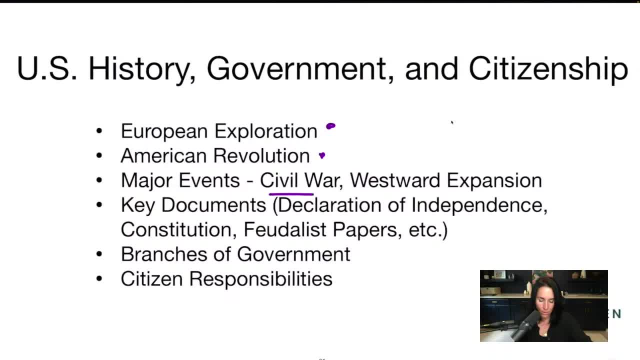 obviously that's going to be a big one. major events, civil war, westward expansion, and these are all coming from the test specifications. you can find these in the test specs. i'll show you how to get those in a second. key documents, of course. declaration of independence, constitution. 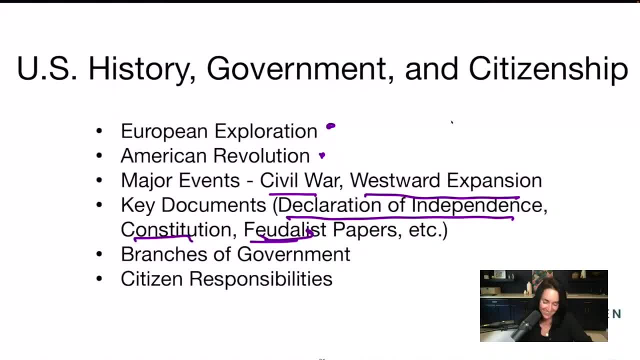 that should say federalist papers, not feudalist papers. sorry, that should say federalist papers. uh, branches of government, and then citizens and responsibilities- want to teach students about civics. all right, so let's have a look at what that might look like. now. this might seem easy for some. 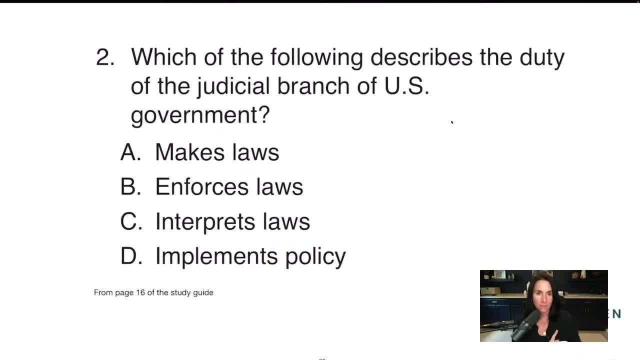 of you, but some of you may not have thought about this in a while, although you should, because there are a lot of things coming up in the judicial branch that you might be interested in, and we should all stay um informed on that. so we have our answer. choices here. makes laws and forces. 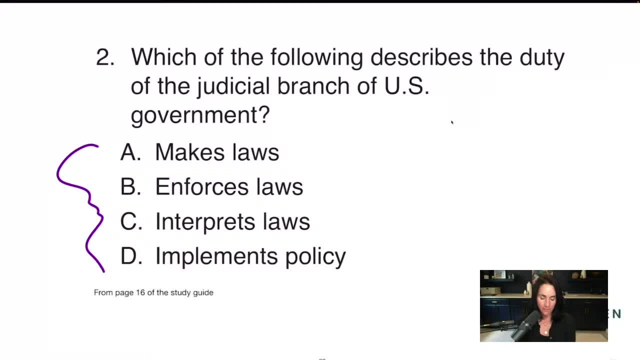 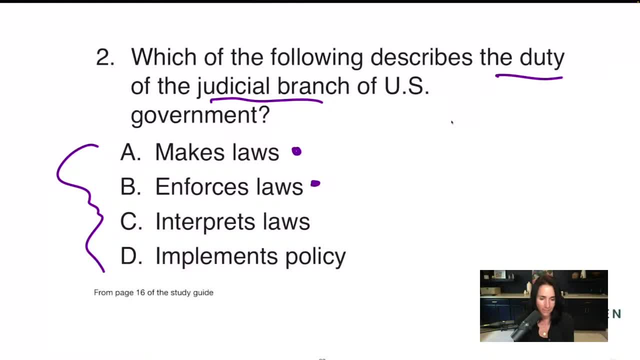 there. there really is none that really, uh, you know, enforces laws. i mean, that's usually done at the local level, or the federal level, or the United States Department of Justice, But the judicial branch interprets laws. Okay. So what do I mean by this? Well, let's say that the president 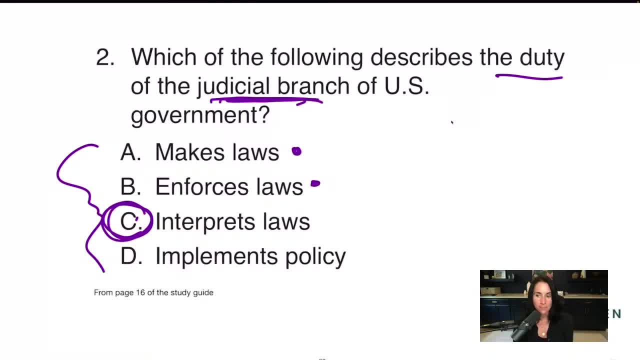 signs an executive order or a state legislature signs, you know, puts a bill and puts a law in effect and it makes it all the way to the Supreme Court, or it makes it to the state Supreme Court, right, Or the federal court. That court will then interpret: is it constitutional? 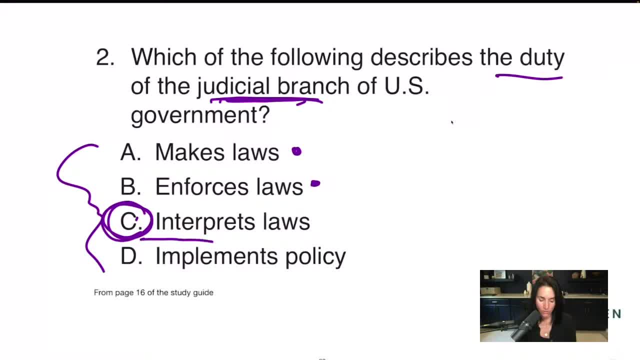 Should it be done this way? Blah, blah, blah. So that's what happens with the judicial branch: They interpret the laws. Now, remember the four. the three branches of government are there to provide checks and balances. So, for example, like I just said, the president can do an executive. 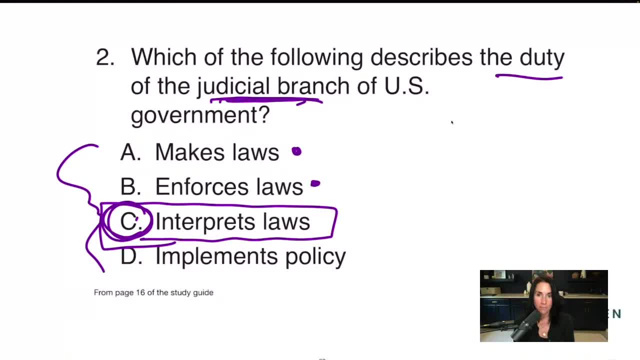 order right, Or the Congress can pass a law, but the judicial branch is the check on that, because sometimes the judicial branch is the one that does the work. So the judicial branch is the executive branch. So the judicial branch is the one that does the work. So the judicial branch is the. 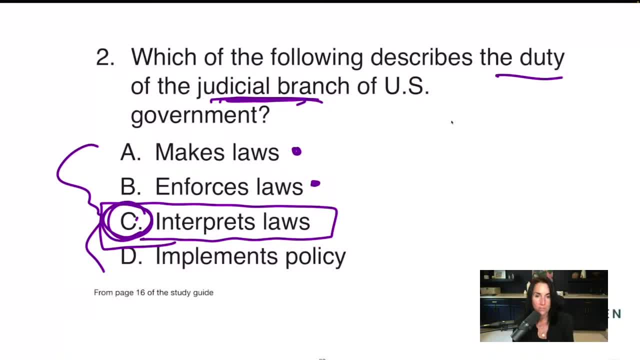 one that does the work. So the judicial branch is the one that does the work. So the judicial branch. someone can bring that to the judicial branch and say, Hey, I don't think this law is constitutional, And then the judicial branch rules on that. So all those checks and balances are. 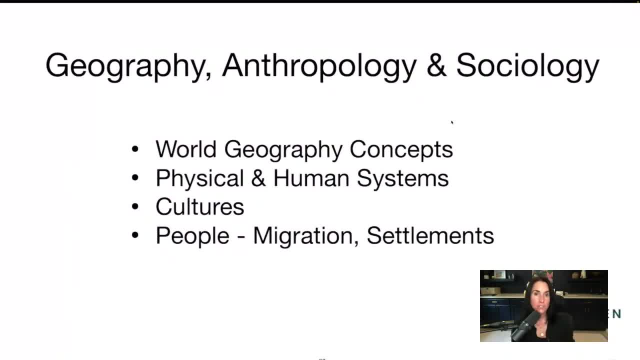 important. Make sure you know that for the exam. Now, the next part is geography, anthropology and sociology And some of these geography questions, you guys, they're tough too. You're going to have questions about, like, an isthmus and mountain ranges and things like that And that. 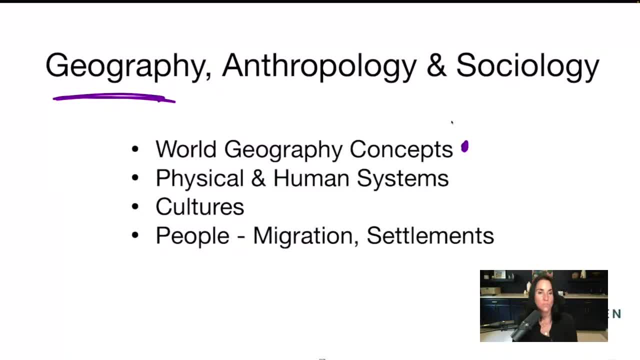 can be difficult. So we want to talk about world geography and concepts. What's going on? It might ask you about the continents and the different countries and things like that. So we need to know that Physical and human systems, how do humans affect the environment? This is a big one. 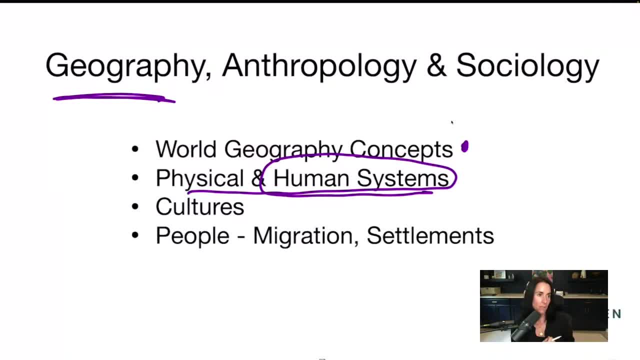 in elementary. We want to make sure kids understand how cities and cars and buildings and things like that kind of affect the physical environment, Cultures. this is that anthropology and sociology portion of the social studies. And then people migration settlements, both past and present. 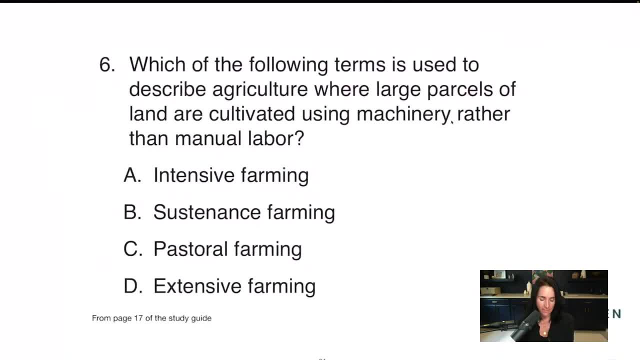 All right, Let's have a look at what that might look like on the exam. So answer choices. here We have intensive farming, sustenance farming, pastoral farming and extensive farming. Let's read the question. Don't know what to do here. Which of the following terms is used to: 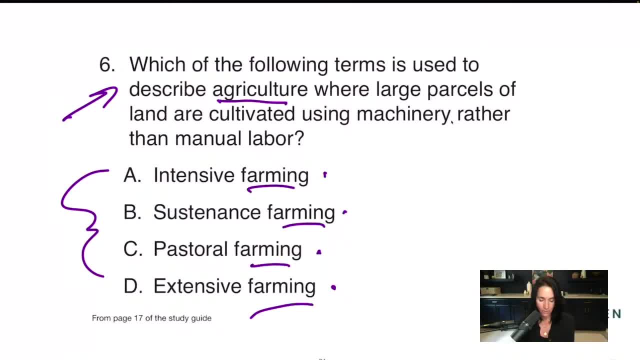 describe agriculture. So we have farming, farming, farming farming, where large parcels of land are cultivated using machinery rather than manual labor. So machinery rather than manual labor is going to be intensive farming. Okay, So intensive farming is when you get a bunch of land and you use a ton of machinery, And it's kind of what we do now: Pastoral farming. 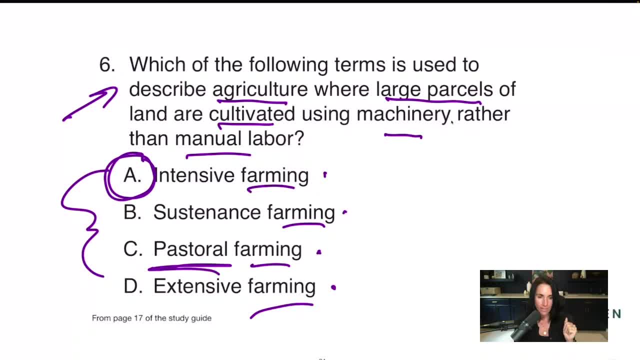 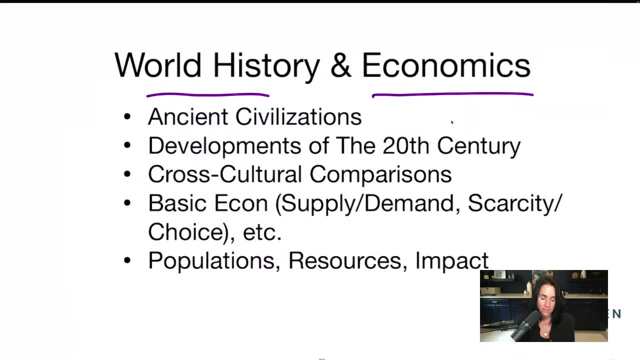 is when you use livestock, And then extensive farming is when you use more labor and not machinery. All right, So six is a there. Let's have a look at world history and econ. Those are kind of smushed together on this test. We have ancient civilizations, So you need to know. 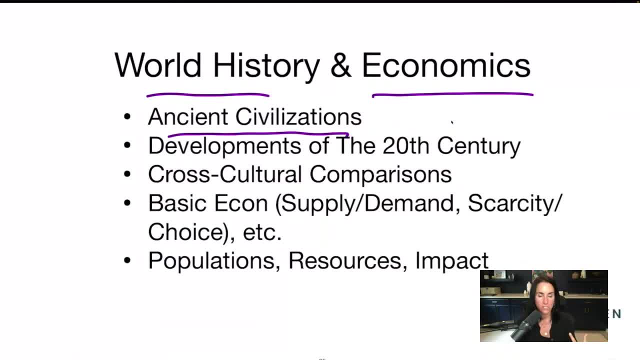 what the Greeks contributed, what the Romans contributed, what the Chinese civilizations contributed, all of that, Developments of the 20th century. So you know cars, the space program, all the different things- I can't really think of all of them. on the top of 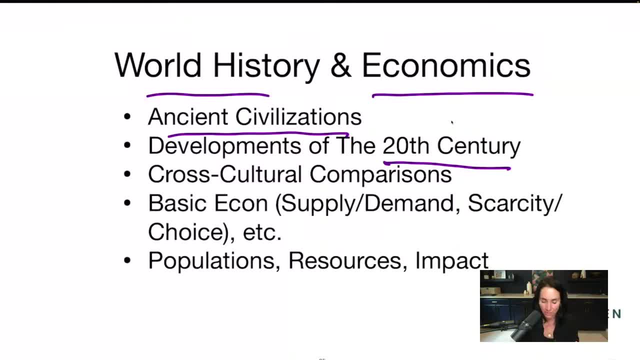 my head, But of course there have been so many in the 20th century. The 20th century was huge when it came to developments, Cross-cultural comparisons. So what's happening in different areas of the world? Basic econ, supply, demand, scarcity, choice, those types of things, And then 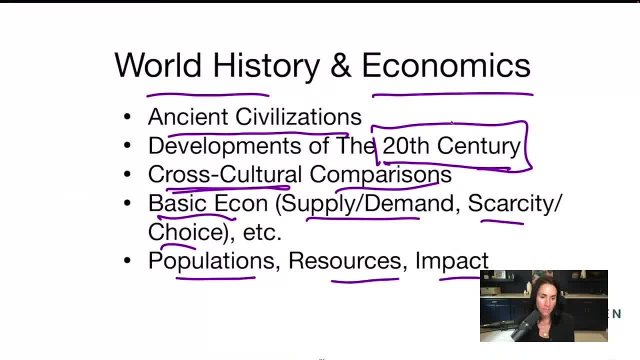 of course, population, resources and impact. That does have to do with economics, population density, what's happening with resources and how that impacts the world economy. Let's have a look at what that looks like. Which of the following example is an sorry? starting with the answer. 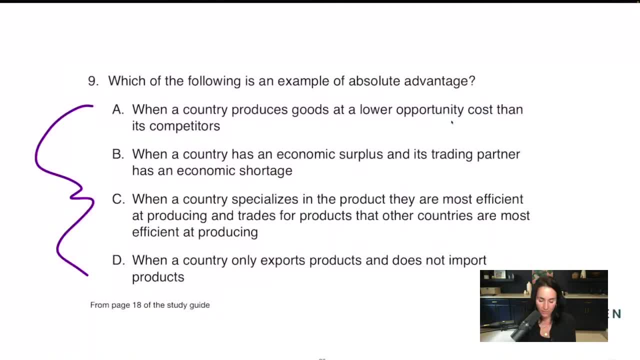 choices here. All right, We have when a country produces goods at a lower opportunity cost than when a country has an economic surplus and its trading partner has an economic shortage. When a country specializes in the product they are most efficient at producing and trades for. 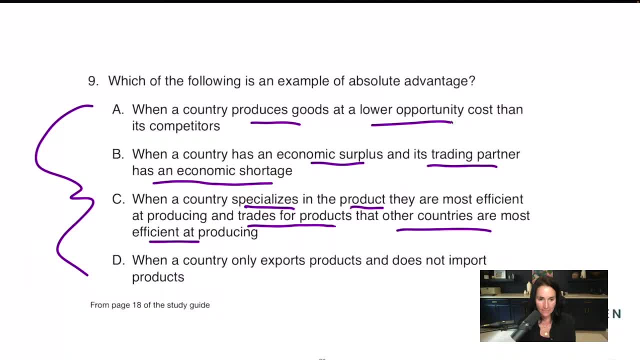 products that other countries are most efficient at producing. And. D, when a country only- we see this word only- exports products. Now, when we talk about only, this is what I call strong language in testing, Typically, if you are stuck and you see the word only or always, 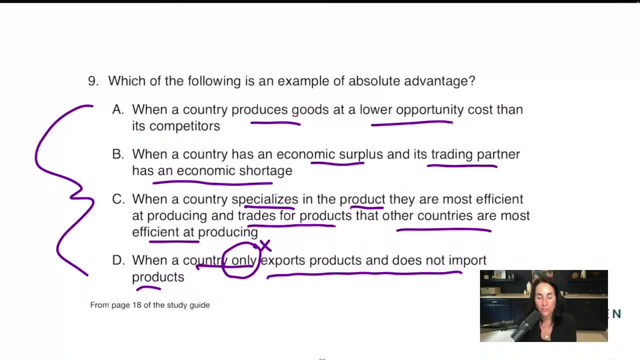 or never is typically not the right answer. It doesn't mean it can't be sometimes, but typically this is what we call strong language in testing And they will put this in to make a somewhat correct answer a wrong answer. So I'm going to cross off D just because it has only Now. 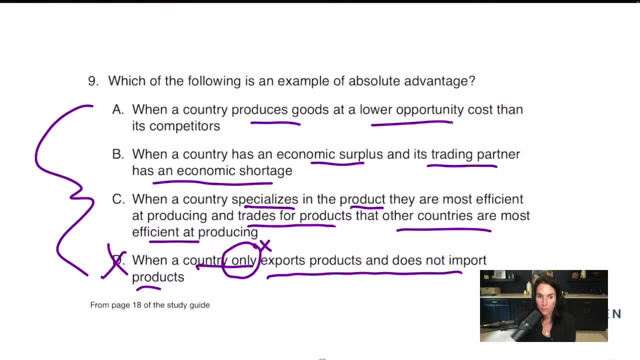 I don't know enough about what's going on in order to answer this, but I did get one taken off by going backwards. Okay, Which of the following is an example of an absolute advantage? All right, An absolute advantage is when a country has the resources, the specialty, to make a certain product and everybody else has to kind. 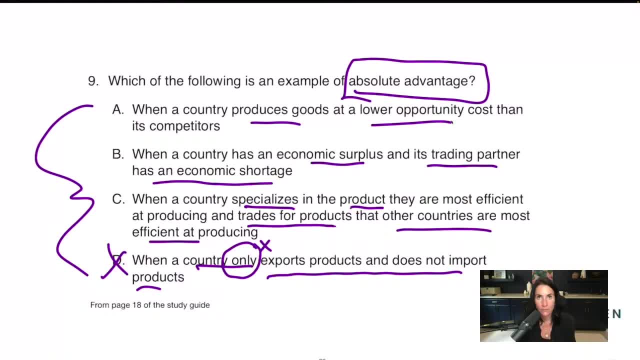 of buy from that country. All right, And you can see. I mean I don't know of an example of a total absolute advantage, but I would say something like: maybe computer chips. right now there are certain countries that have an absolute advantage. We are trying to get back into the computer chip game. 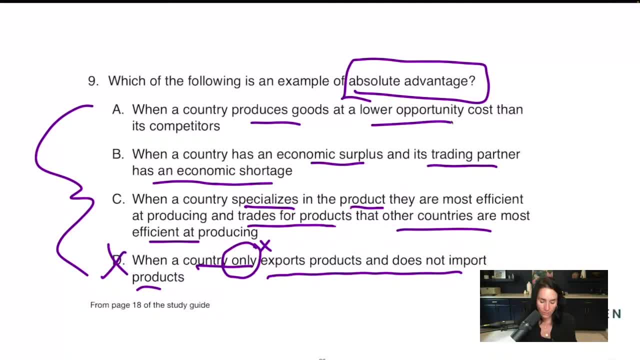 or semiconductor chip, game things like that. But it's when a country specializes in the product and they are most efficient. Notice those words: specialize, most efficient, Those give you an advantage. Even if you didn't know what was going on here, those keywords would help you. All right, And it gives. 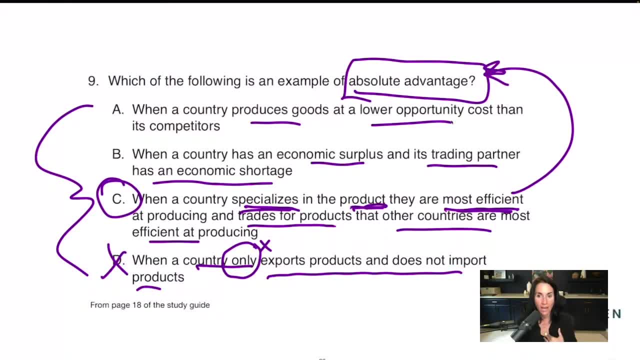 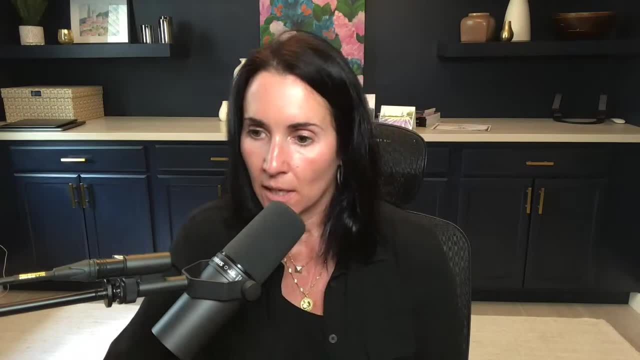 them an advantage because I can- if I, if I specialize and I produce it the best, I could set the price at whatever I want and they do, And so that's how that works there, All right, All right, Let's go back here and see if we have any questions. Um, as you continue to create, 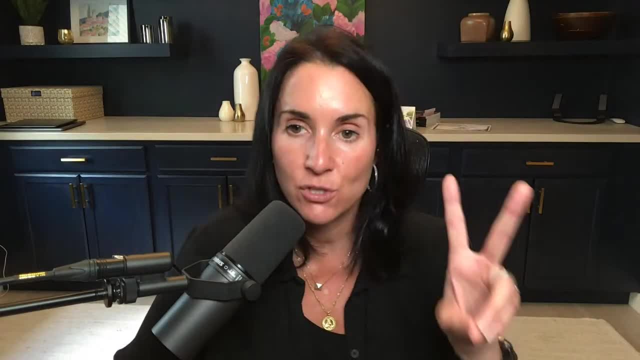 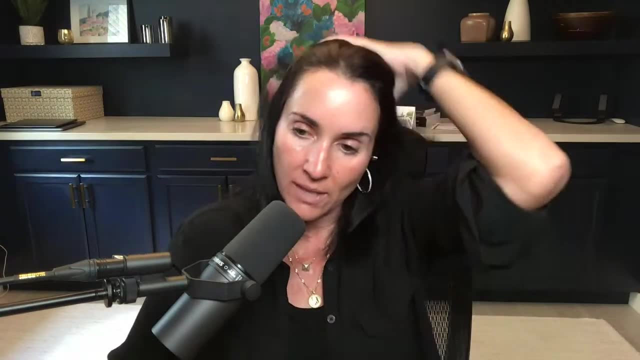 content. will you produce material for secondary education? Yes, I will. I have two secondary education books for English language arts. I have a third one coming out and I'm going to be working on some social studies stuff. So, yes, Any advice on how to overcome test English? 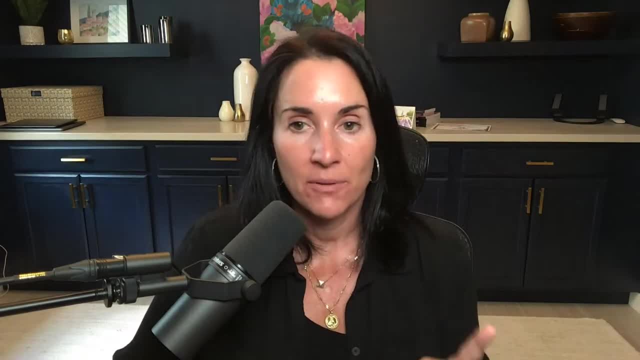 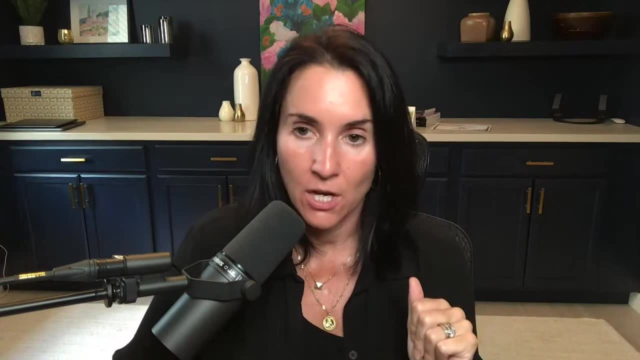 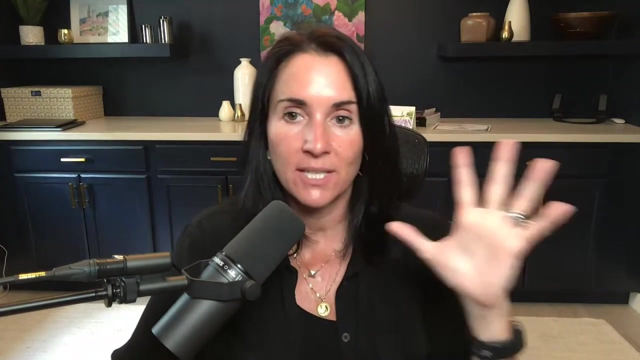 Anxiety. So with test anxiety, a couple things you should know It's common. First off, you do not need a hundred on this test. You need like a low C, high D to pass this exam. So try to get that out of your mind a little bit. The second thing is is that you can take the test as many. 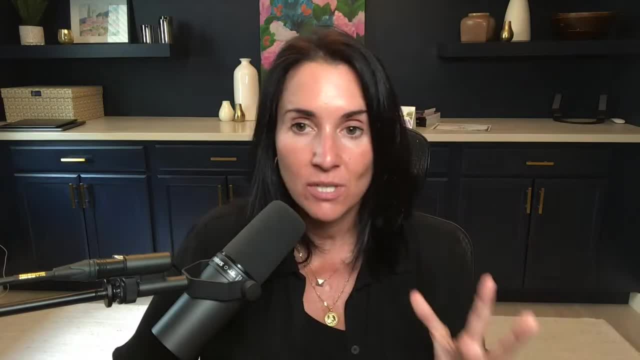 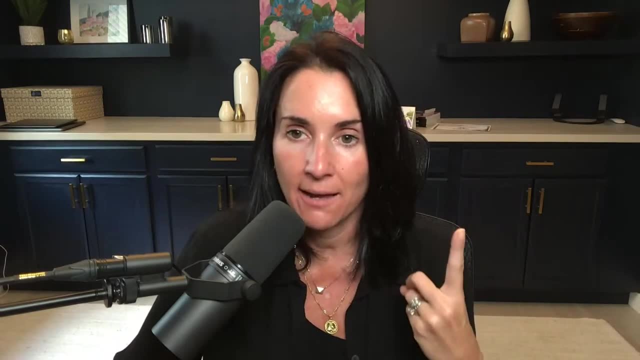 times as you need to, And so if it takes you two times, three times, four times, I know that's not ideal and it's expensive, But you've got to think in terms of I do not need an A, I need a D. Sometimes you need an F. 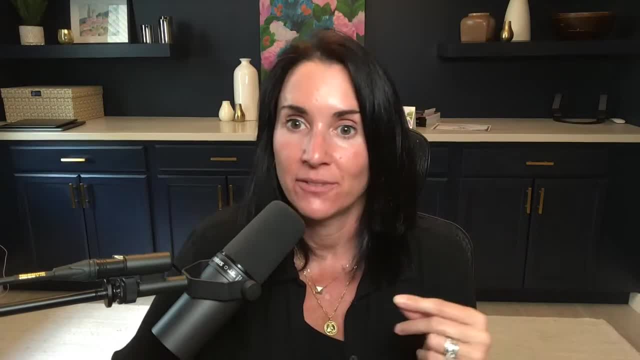 All right And on some of the harder exams, a low F like the physics and the chem for high school- you can get a really low score. So nobody's asking you to be perfect on this exam And if you prepare properly and you really read and understand, you will eventually pass. You will. 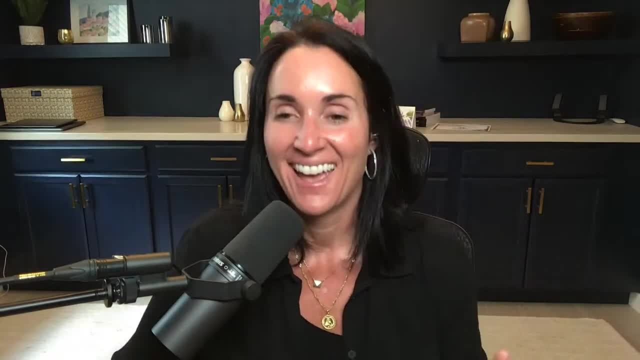 pass. You've got to. you've got to calm down And I know that's hard when you have anxiety. But if you're ready, you're ready to go. And I know that's hard when you have anxiety. but if you're ready to pass, you will pass. You've got to. you've got to calm down And I know that's hard when you have anxiety. 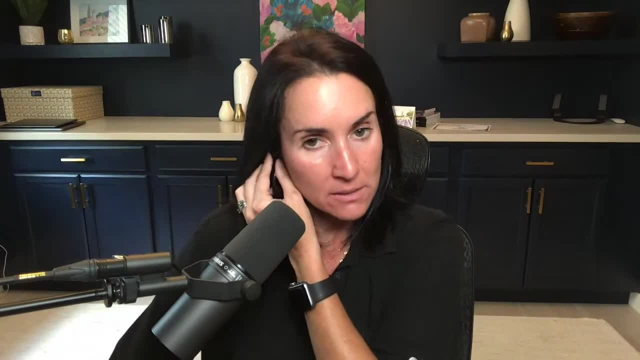 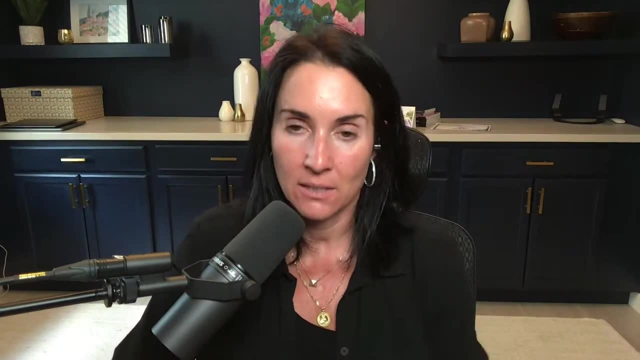 but what I typically do if I'm going to take a difficult exam. I listen to some really good music on my way there, and I remember that I can take this test as many times as I want. Beyond that, it's hard to get over anxiety, and so it might be another underlying cause there. 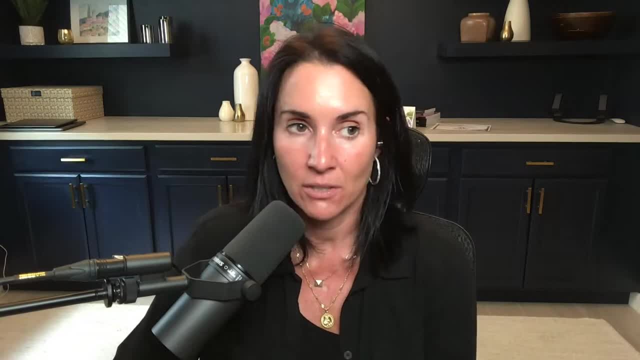 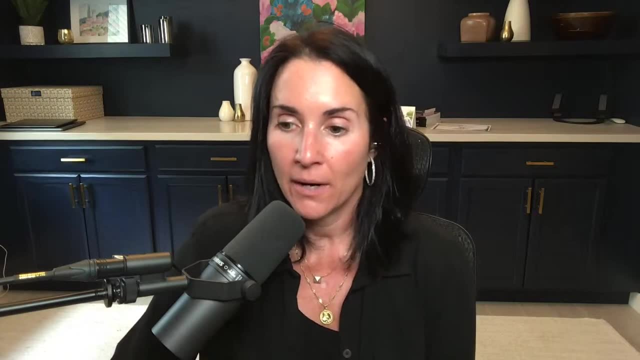 but that's going to be my advice to you. You can take it as many times as you want and you don't need an A, You need like an F, high D to pass. okay, All right, any tips for the science part? Oh, you're taking it at 12 today. All right, we're doing science. Paula, let's go. 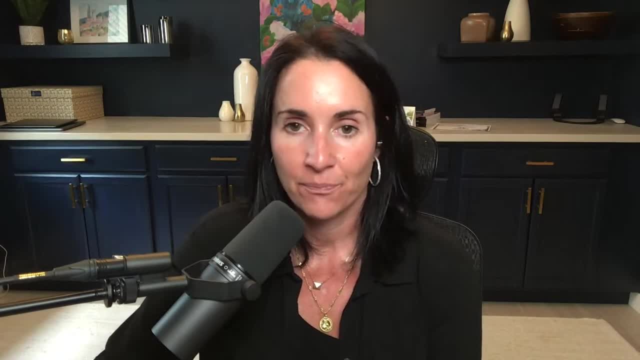 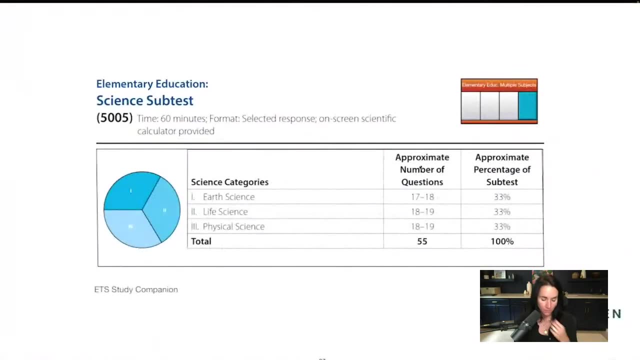 We're doing science right now. Here we go. Okay, let's talk science. Let me just make sure we're on science. Yes, we are, Okay, here we go. The science test always going to have the same content categories. We have earth science, which is going to be the sun, moon, stars. 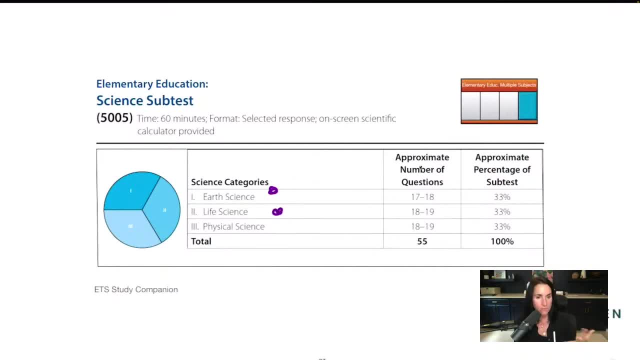 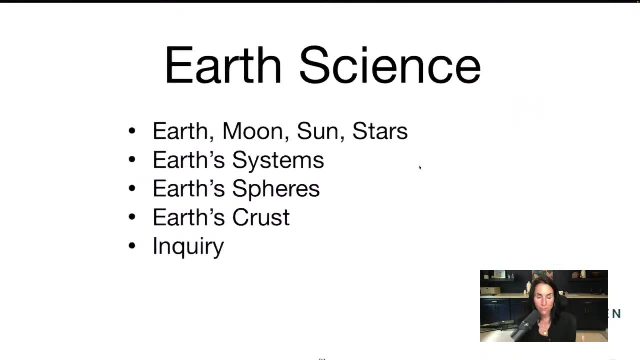 things like that: Life science, which is going to be biology, cells, ecosystems, animals, human systems, And then physical science. those are going to be your machine questions, energy questions, magnetism, electricity, things like that. okay, Now, with this, it's a lot of memorization of. 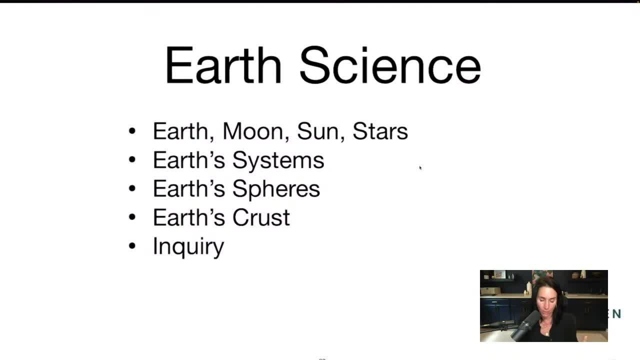 stuff. but if you know where the questions are coming from, it will really help you. So for earth science, we have earth, moon, sun and stars, Earth systems. so you know the hydrosphere how it works: water evaporates, goes up into the clouds. 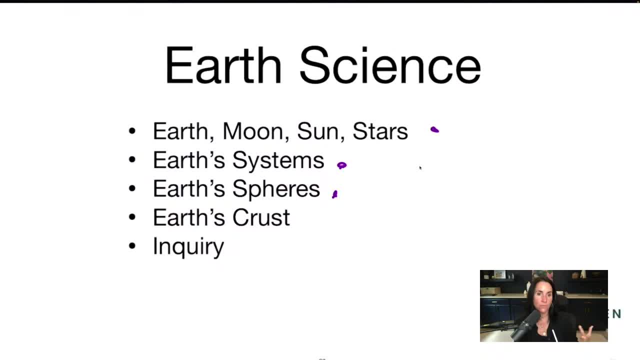 things like that. You're going to need to understand that Earth spheres- biosphere, cryosphere, lithosphere- all of that- The earth's crust, that's the lithosphere and what happens below it. And remember if you get a question on the exam about how to increase. 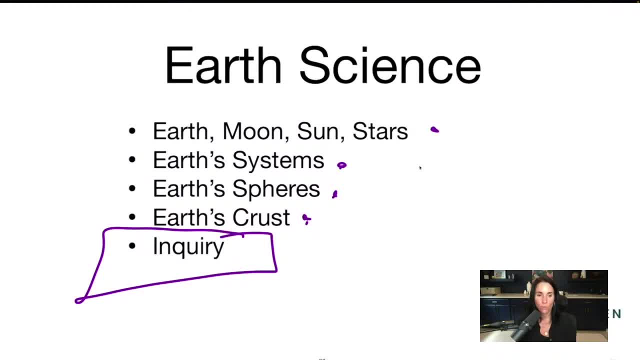 you know, student engagement or anything like that. inquiry, inquiry, inquiry-based learning, getting their hands dirty, looking at a rock, touching a rock, rather than just reading about a rock. okay, That's going to be really important here. Let's have a look at a question you might. 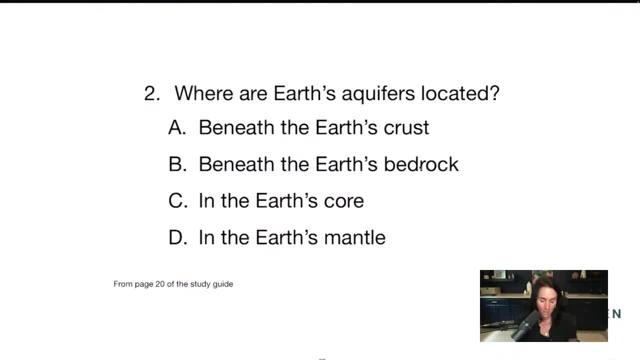 see on the earth's aquifer, on earth's surface. So let's have a look at a question you might see on the earth's surface. So we have here beneath the earth's crust, beneath the earth's bedrock, in the core, in the earth's mantle. So we have: where are the earth's aquifers located Now? 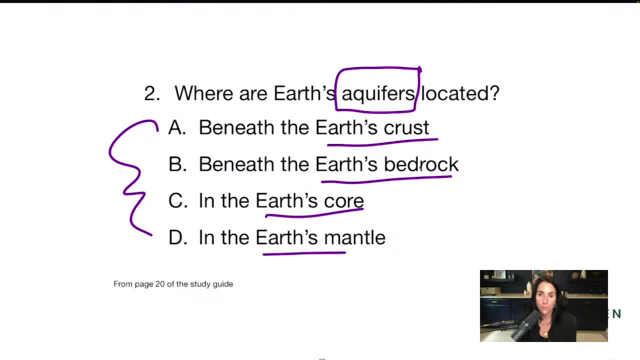 one of the things with science. we can kind of use our common sense here. Aquifers are where we get our water and it's definitely not in the earth's core. So that's out In the earth's mantle again way too deep. You're talking hundreds of thousands, not hundreds of thousands. 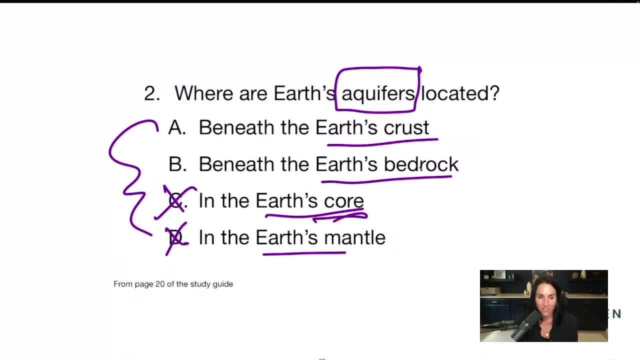 I don't know, thousands of miles deep into the earth. There's no, there's no way to extract water from there. It's not hundreds of thousands That would be. we would have a very large planet if it were hundreds of thousands of miles. but it's going. 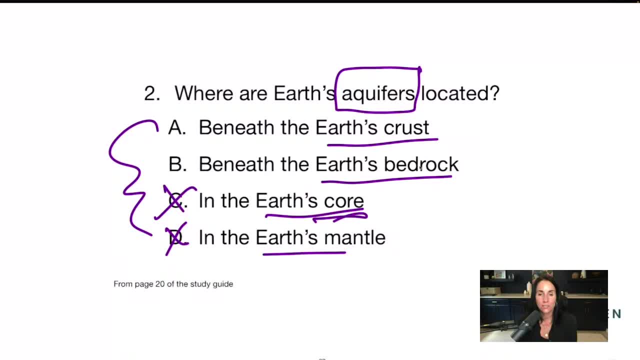 to be several miles into the earth, and it's too. it's too deep. right Now we have this bedrock and crust. Well, think of bedrock. Bedrock is really hard, It's going to be hard to extract. 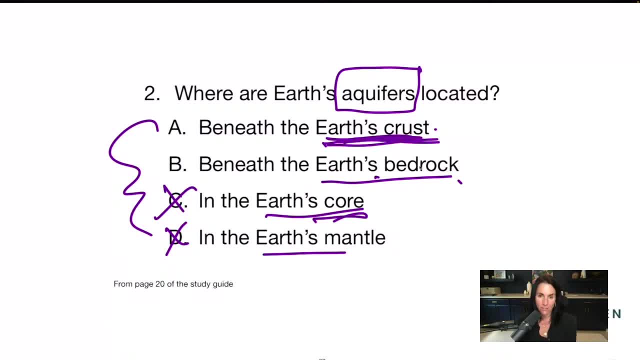 water from the bedrock. It's just below the earth's crust, at the saturation point. That's where we're going to get the water from our aquifers. So even if you narrowed it down 50 to 50, you'd have a good chance. but the core and the mantle- these are way too deep into the. 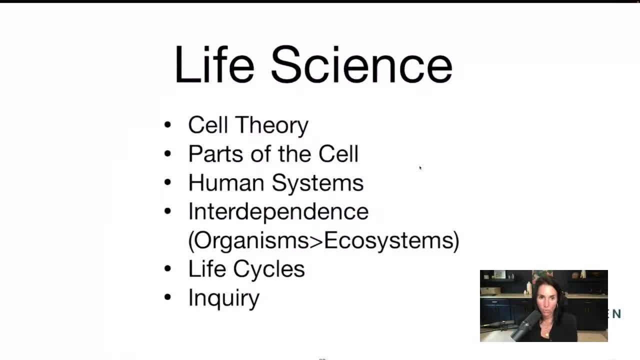 into the earth Now life science, and it's good to know these questions, like where these questions are coming from. You're going to get stuff on cell theory, parts of the cell, human systems, interdependence, organisms and ecosystems, life cycles and again. 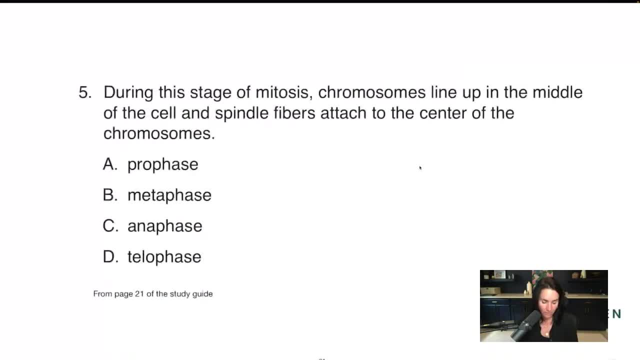 inquiry is huge on the science, So let's have a look at what that looks like So I can see from the answer choices. I'm talking about cell division, prophase, metaphase, anaphase, telephase, And I might be like, oh my gosh, I don't, I didn't brush up on that. Well, 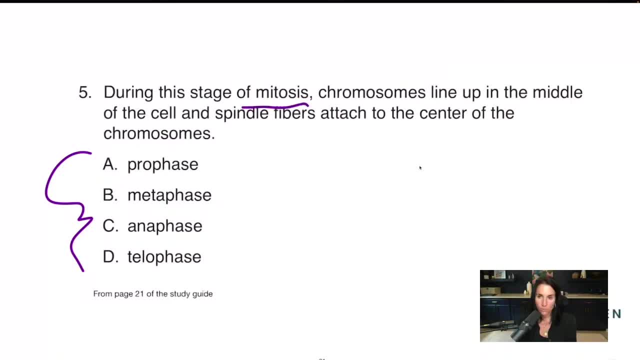 let's have a look at the question. During this stage of mitosis, chromosomes line up in the middle of the cell and spindle fibers attached to the center of the chromosomes match middle and metaphase up together. You will probably get a question like this on the exam. 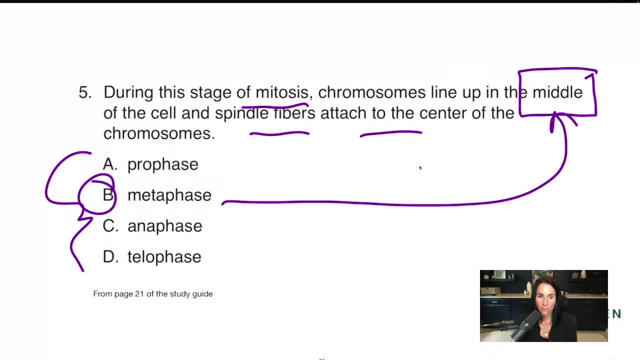 Um. I always like to use the metaphase example because meta and middle match up and it's very common to see a question about metaphase on the life science portion of any exam. So make sure you know your, your um, your stages of cell division, and you don't have to get into it too. 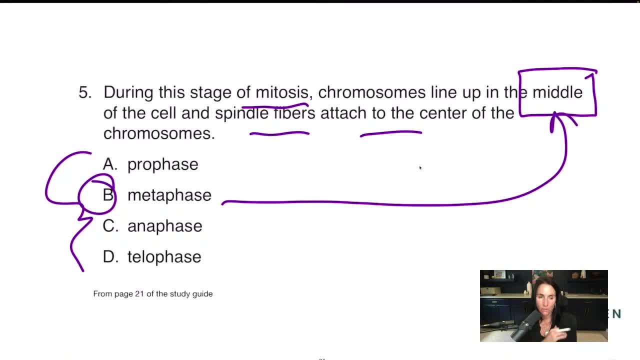 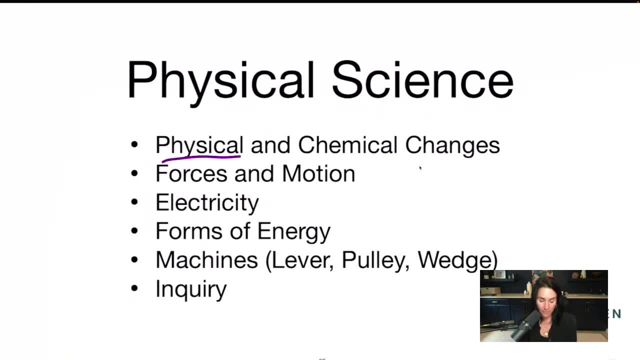 much, Just know the names and the stages of each uh point of the cell division. All right, And now let's go to physical science. So with physical science, physical and chemical changes, uh forces in motion, electricity. 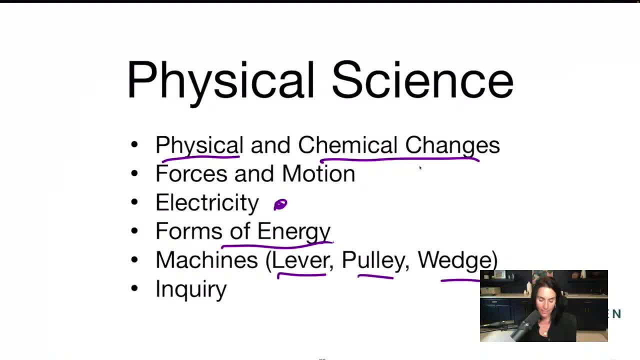 forms of energy machines: lever, pulley, wedge and, of course, again inquiry. All right. So physical changes are things like breaking, ripping, tearing. Chemical changes is when the chemical makeup actually changes, like rust. Rust is because of something that happens with 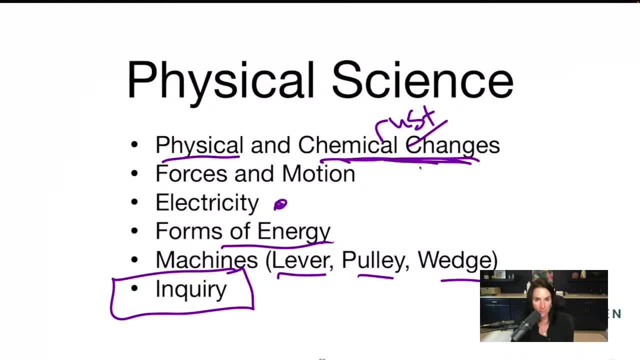 oxidization and it changes the molecular makeup of a substance And that's why it's called a chemical change. A physical change is just when something changes physically Okay, Like ice Melting ice, It's still H2O, It's just in ice form. When I melt it, it's still H2O, Okay. So make 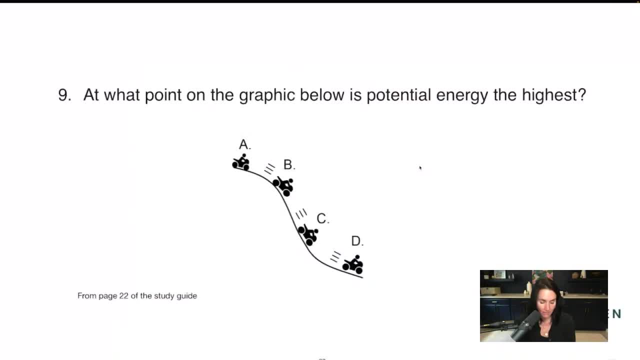 sure you know the difference with that. Forces in motion is going to be one, And in fact I have a good one here. It will help explain uh different uh energies. So I have this cute little diagram here, a guy on a motorcycle- And it says at what point is the potential energy highest? Okay, Think. 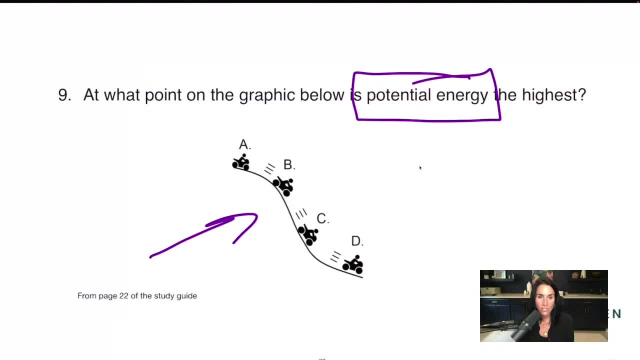 of a pendulum or this situation. Potential energy is when something has the potential to move and if we're up here in A, we are ready to go. If we're on a swing, and the swing is all the way up here and it's getting. 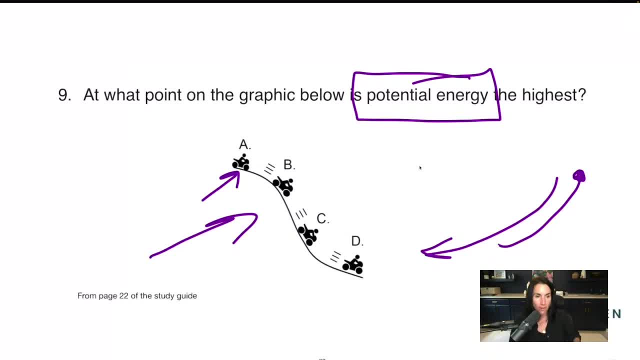 ready to go down here. that's potential energy. If I hold my pen in the air and before I drop it, that has potential energy. okay, The potential energy is highest at the top, Just like if I hold this pen up in the air and I drop it, the potential energy is highest when it's at the top. 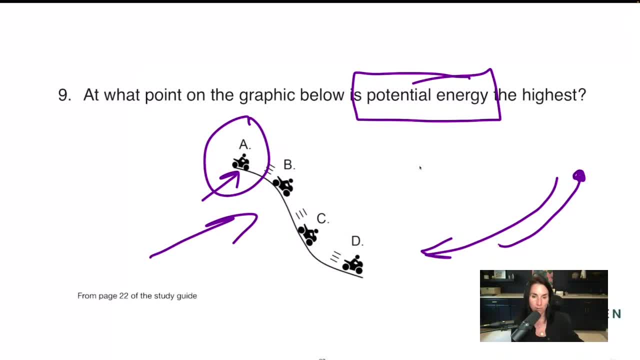 Once it hits the floor, the potential energy is virtually zero. So the highest potential energy is here, and remember this. the highest kinetic energy is here. That's when the thing is going as fast as it will go okay, And so potential and kinetic energy is on this exam, so make sure. 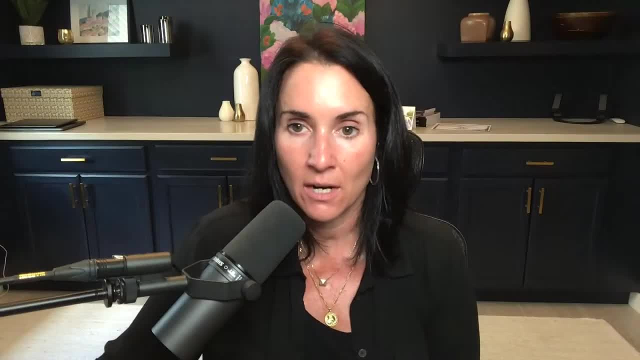 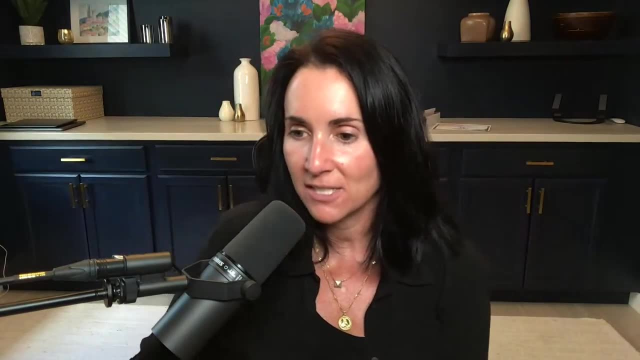 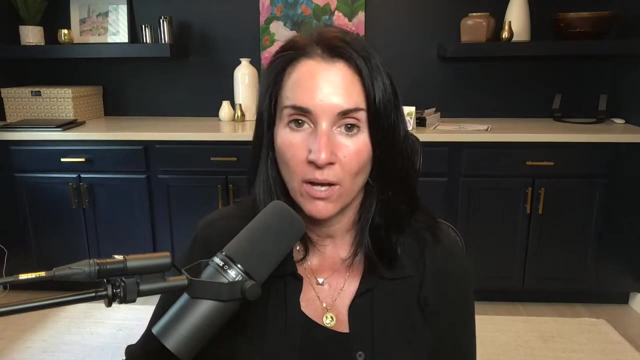 you know that, All right, so let me stop sharing there And let's go back here. Okay, so potential energy equals energy at rest. Yes, yes, yes, All right. yes, good luck, Paula, on your exam. If you do have the study guide, go ahead and review all that. 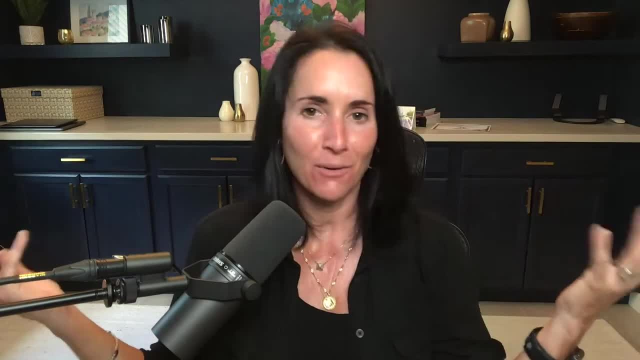 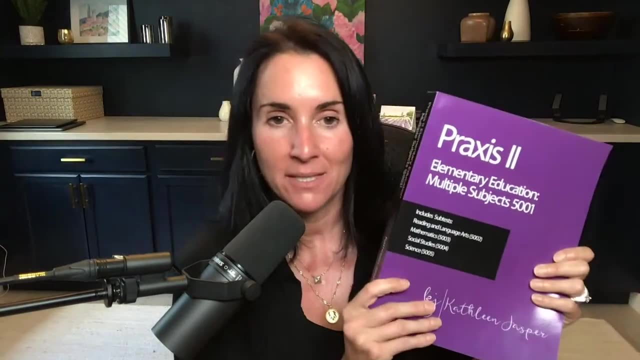 All right, this is bringing us to the end, so I do want to show you. it's not bad, only 10 minutes over. Usually I go like way too long. Okay, so really quickly. this is the book that I made the. 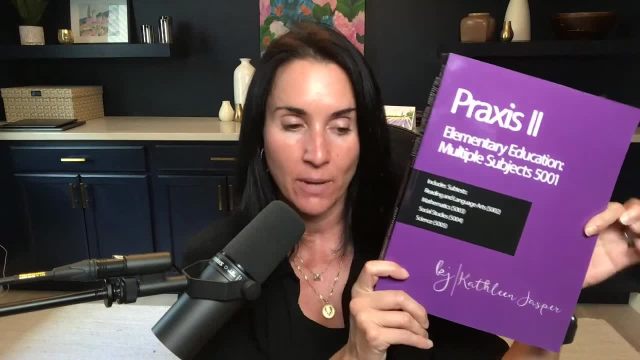 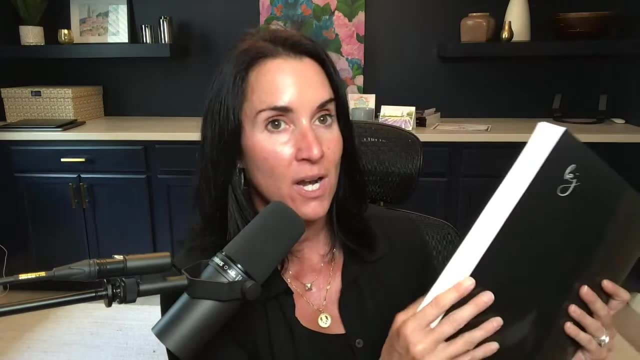 study guide for so. but I used this book, The Praxis to Elementary, and I'm going to show you how to do it. I have the same book for the 5901.. If you're waiting for the 7811,, the 5017, and the 5006,, 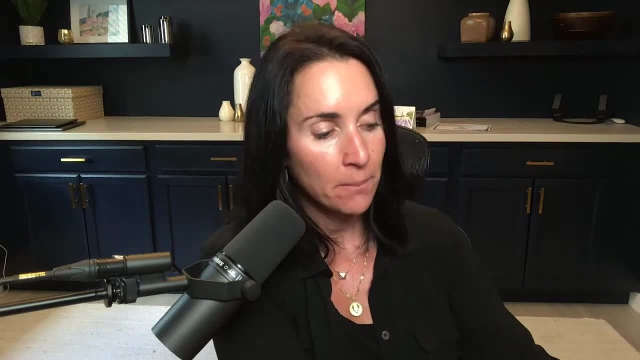 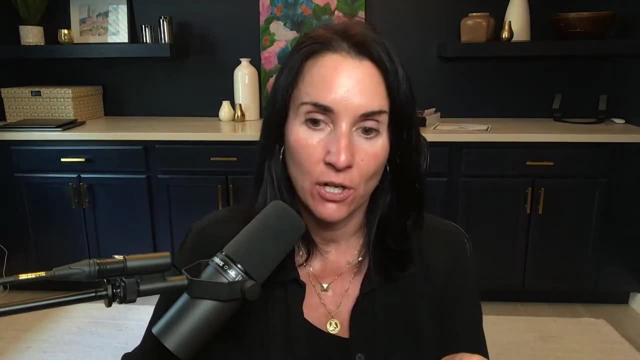 it's in the works. okay, Let me show you where you can get it. and when you get the email today from me, you're going to get an offer code to buy the book, So I'm just going to give it to you here. 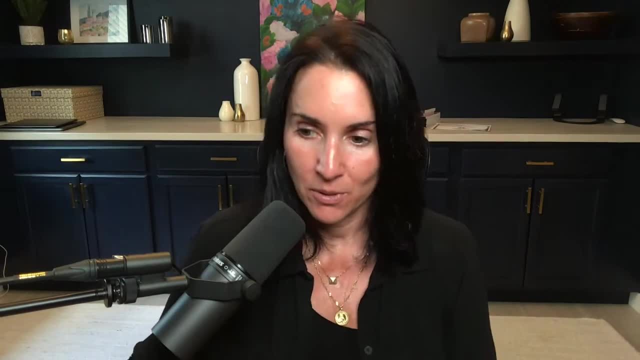 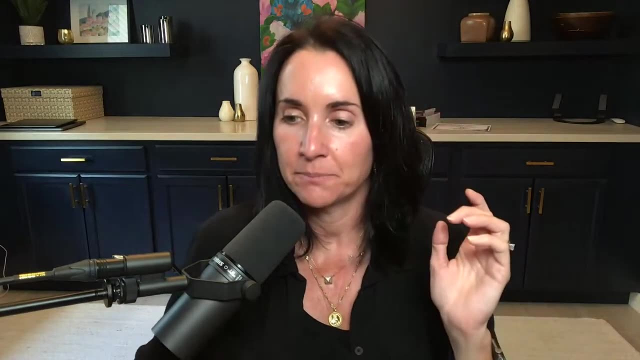 It's Praxis EE20,. all right, So I'm going to put it in the chat here- Praxis EE20, and I'll throw it in the. I'll throw it in the email you get If you're watching live on YouTube or Facebook. that's the. 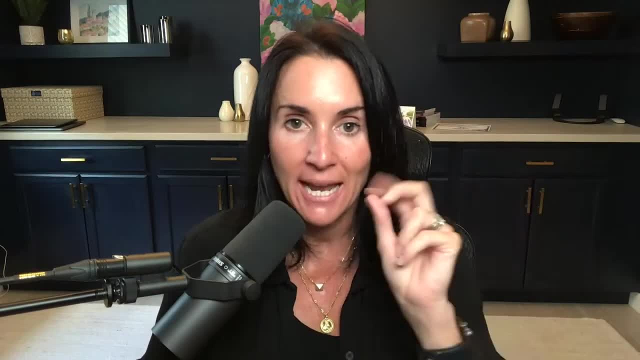 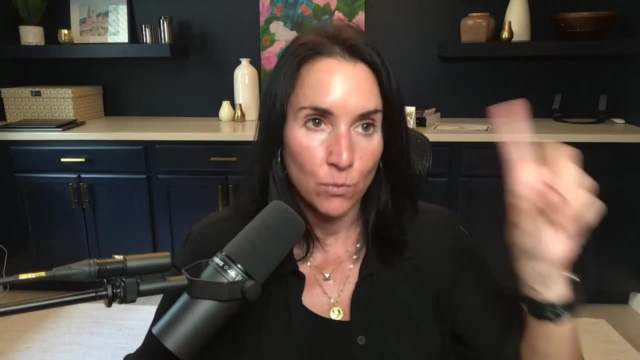 word Praxis, EE, as in elementary education, 20, and that will give you 20% off. all right, Now, really quickly, if you let me share my screen here, let's go to, okay, so I have just. 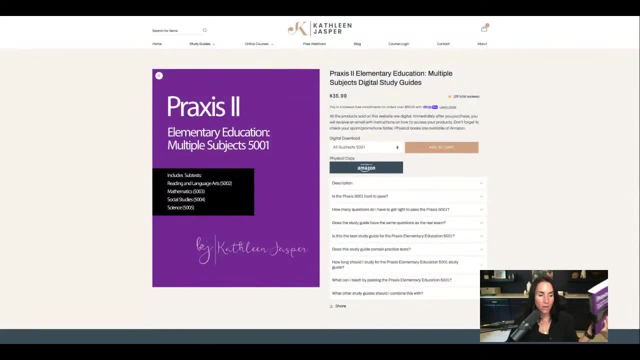 a little bit of information here. So I'm going to go to my study guide, which is great. I showed it to you. It's over 400 pages, over 600 five-star reviews. all that, but let's say you need more support. 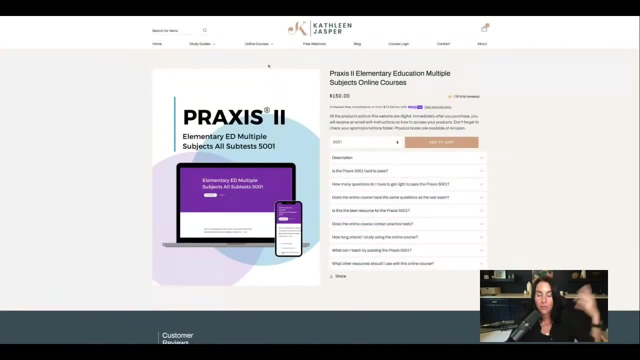 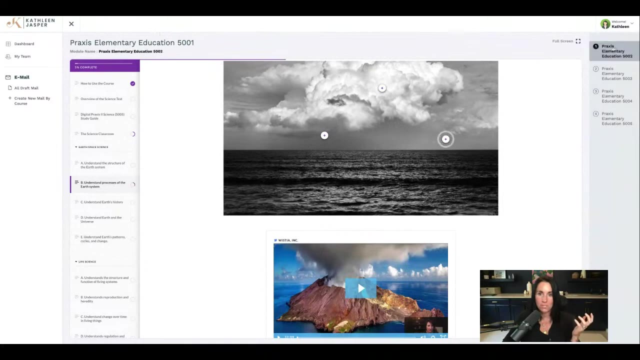 Some of you need more support in the math. Somebody talked about math anxiety. Somebody talked about needing more help in science. In these online courses there are videos and extra practice and things like that. In fact, let me go. This is what the online course looks like, So you can see. 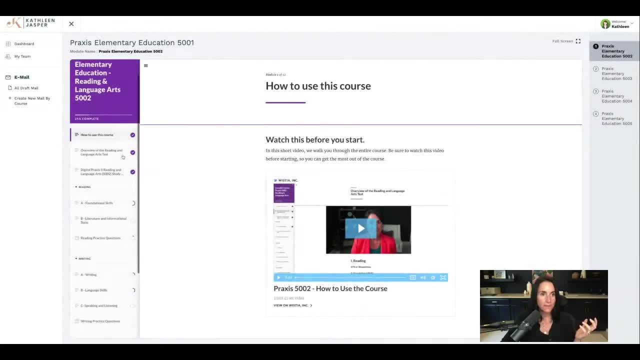 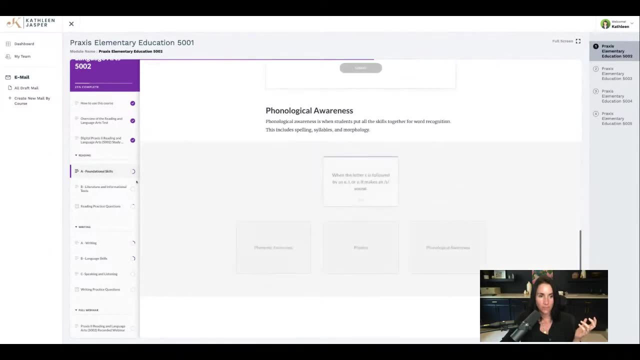 for the Praxis: 5001. You can. or 5002, foundational skills. all of this information here. all of this information, It's got flashcards, it's got videos and it has full practice tests at the end. 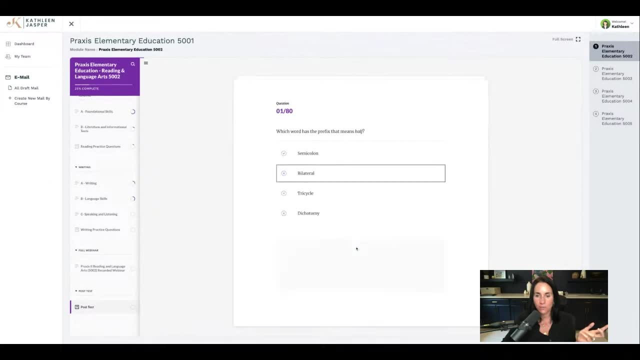 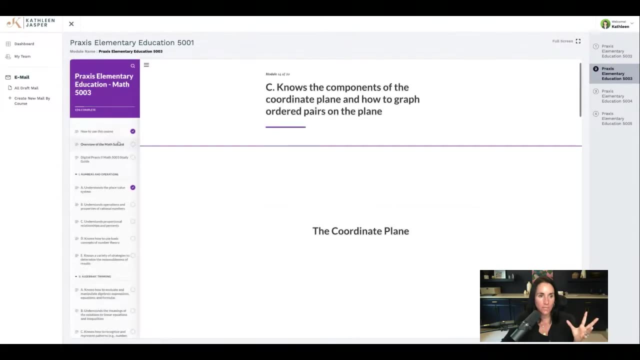 And it gives you a score And of course it's got the answer explanations to tell you why. Let's just hop on over to math really quickly So you can see so much content in the online course. Look at all these videos, I mean it just there's so much to go through in this course, So if you 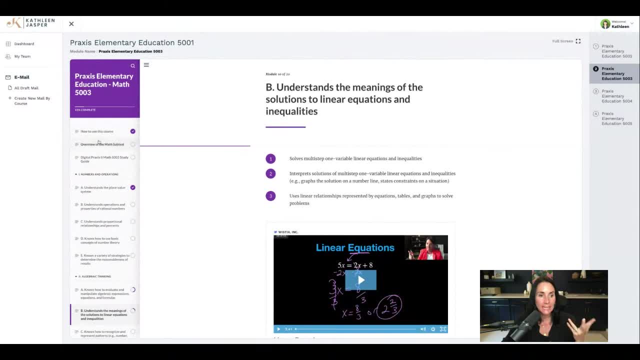 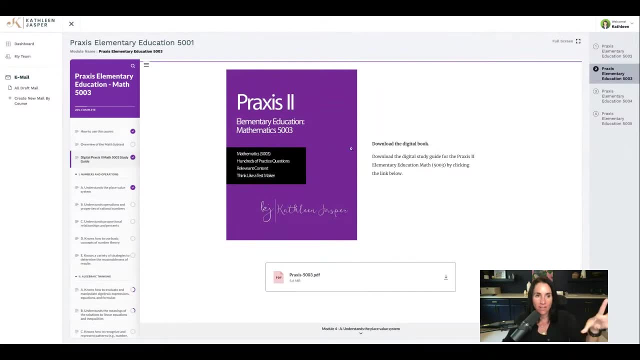 need a lot of extra help. this will help you And again, in all of this, you can get the online book, the digital book. I separated it in this course so that you download the 5002 separately, the 5003 separately, because 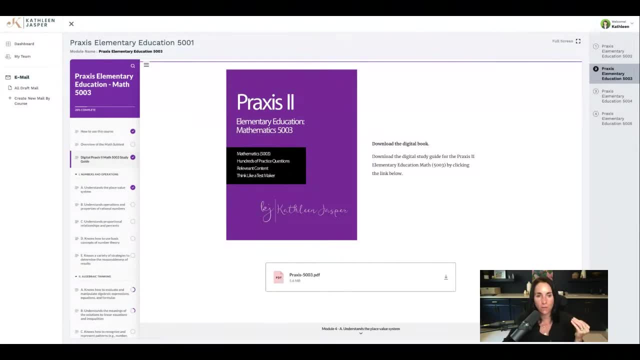 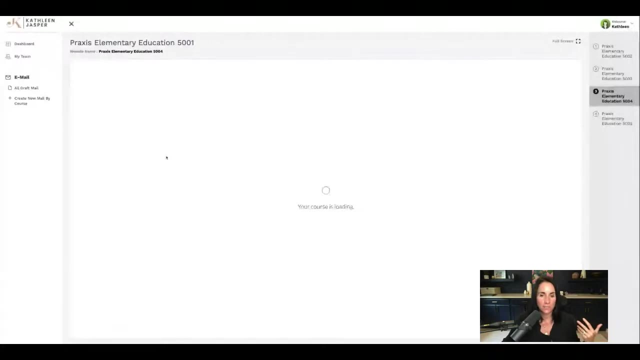 it's just easier that way. But when you buy it, it all comes at once if you buy the digital study guide. So this is going to help you a lot. And again, I have the social studies, tons of videos to explain, you know, European exploration. 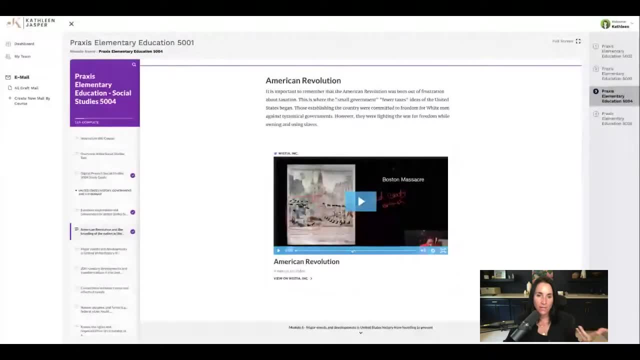 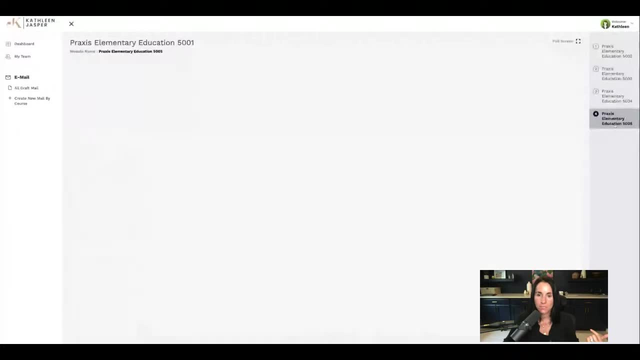 all of that stuff. So if you're interested in learning more about math, you can go to the American Revolution, And the videos are anywhere from like five to some of them are 20 minutes depending. And then, of course, I've got here for the science, all the science concepts It's got. 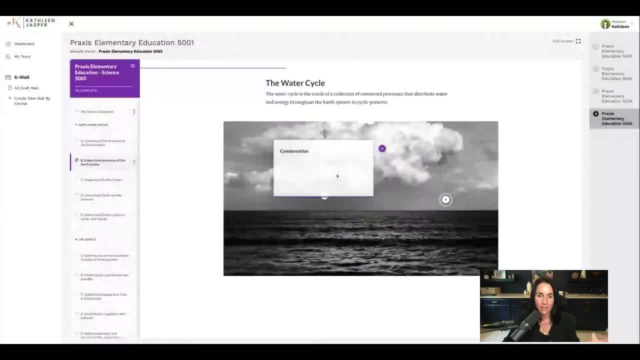 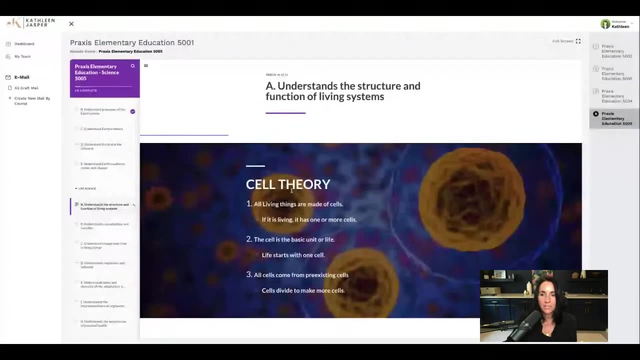 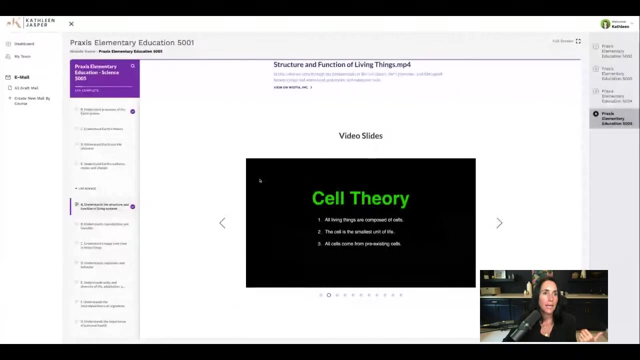 like interactive stuff you can click on people like that, earth's processes. Let's go down to life science, which is my favorite, And so you can see here cell theory and all these different diagrams I do and video slides and things like that. So there's a lot here, All right, And then 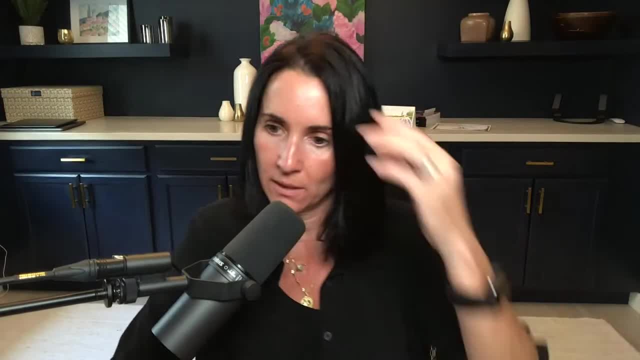 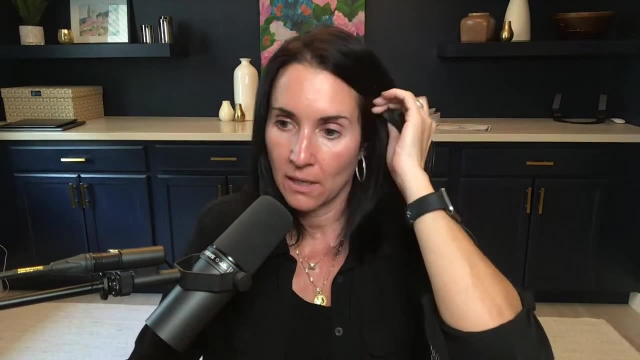 if you're interested in learning more about math, you can go to the American Revolution, And so that will help you. Okay, How effective are flashcards for each content area? Flashcards are awesome. If you want to do flashcards, that's fantastic. Can you go back to the 5002 writing? 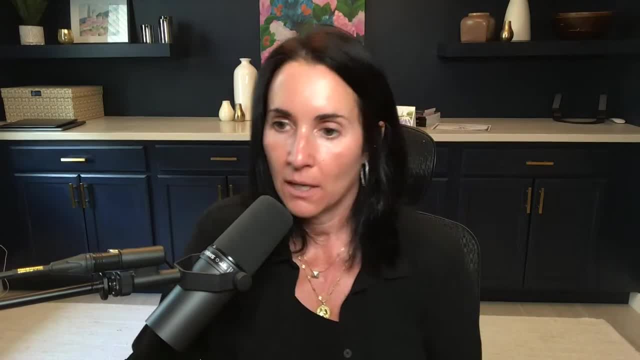 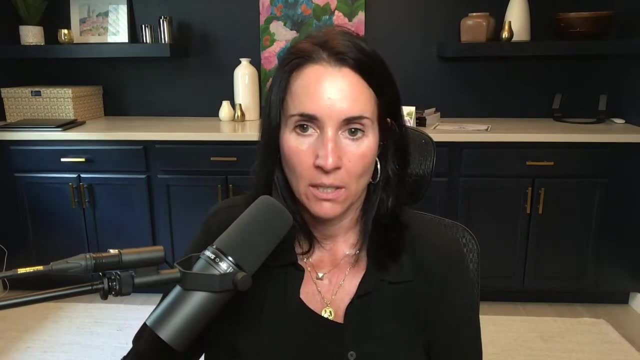 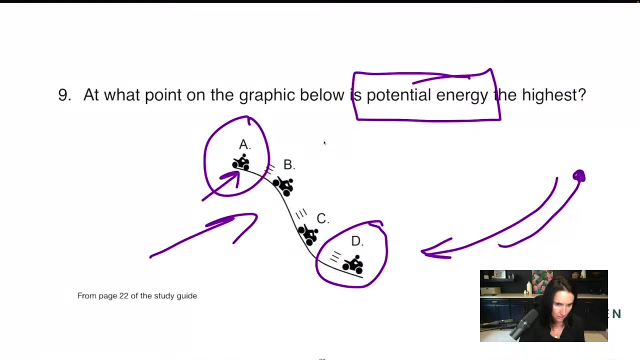 portion. Yes, I'll just hop back there really quickly. Jennifer's asking about the 5002 writing portion, So let me just hop back to my thing here And let me go to writing. Okay, Right here, Writing, speaking and listening. We talked about how the writing process and the 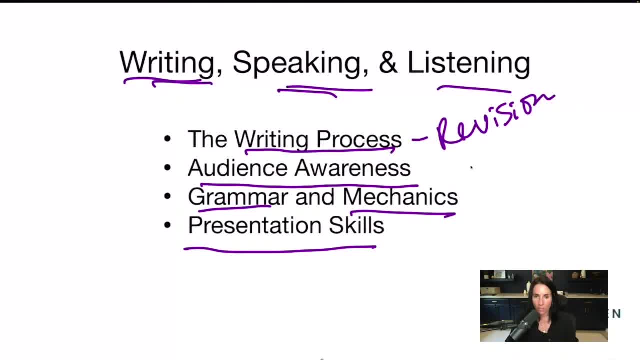 revision is most important here. You need to know the steps of the writing process. I do go over that in the book and in the online course And I have a video on it on my YouTube channel. Audience awareness- making sure students understand what they're writing to who they're writing to- is 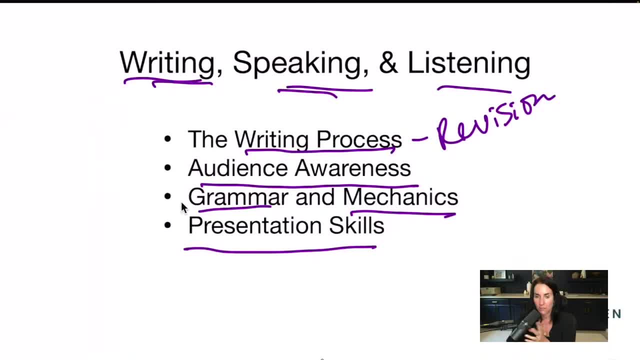 really important. There's a little piece of grammar and mechanics there- elementary ed specific- And then of course there's a little piece of grammar and mechanics there, And then of course there's a little piece of grammar and mechanics there, And then of course there's a little piece of grammar and 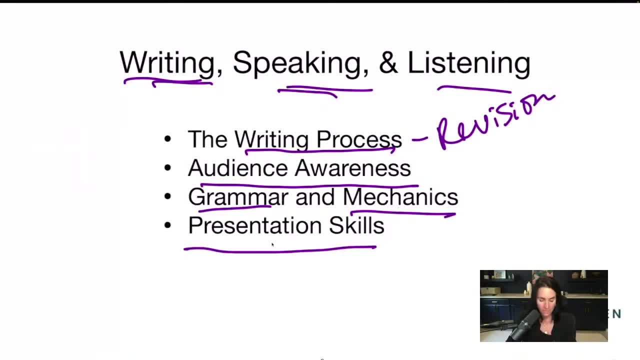 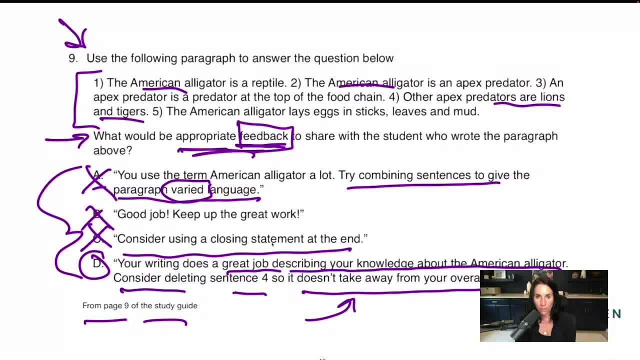 mechanics there, And then, of course, we have to teach students the writing, speaking and listening skills, And the question that I went over was this appropriate feedback question. Notice that answer D. we're giving feedback to students on their writing. This right here is a. 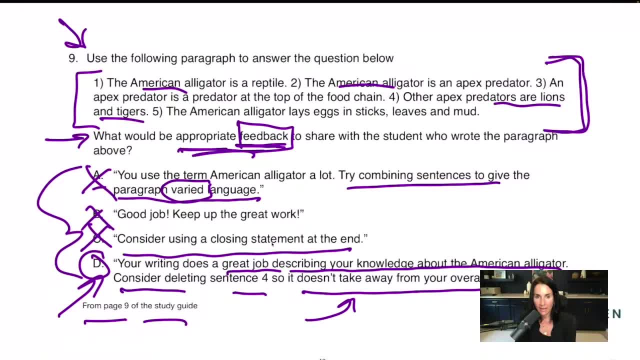 little piece of writing that the student did. And when you give feedback, you need to make sure that you have specific and meaningful feedback, meaning you talk about why something is good and why something is not good. This good job- keep up the good work- is not a good enough feedback. 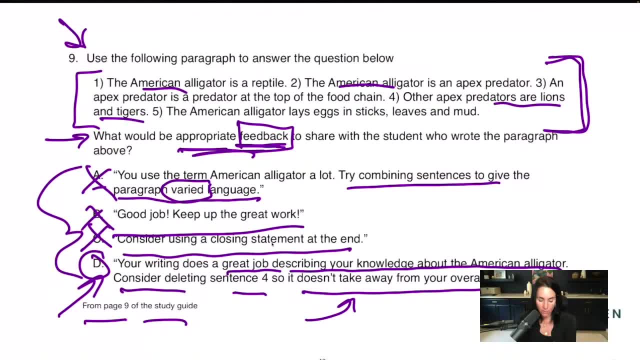 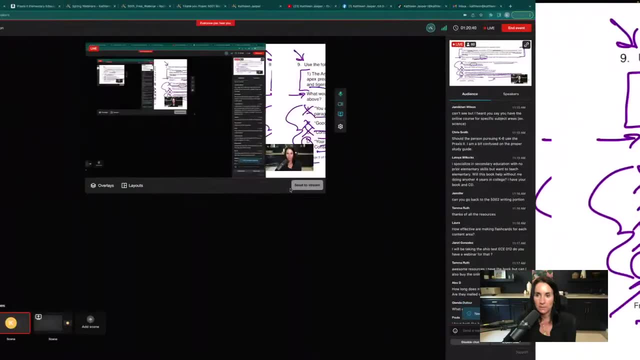 So what you want to do is: D talks about it, gives a little praise- You did a great job talking about the American alligator, So it's specific. And then we have a critique: consider doing this, And that is also specific. So that's really important for the writing. All right, Now again, I'm only 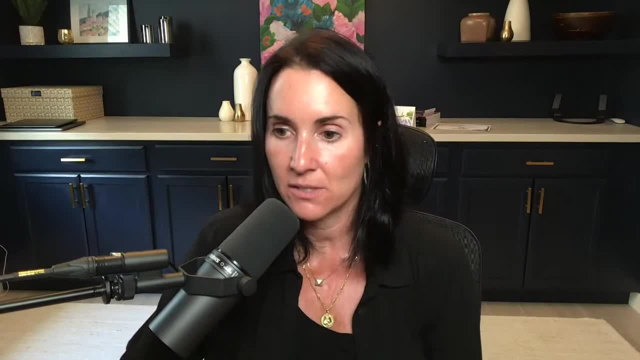 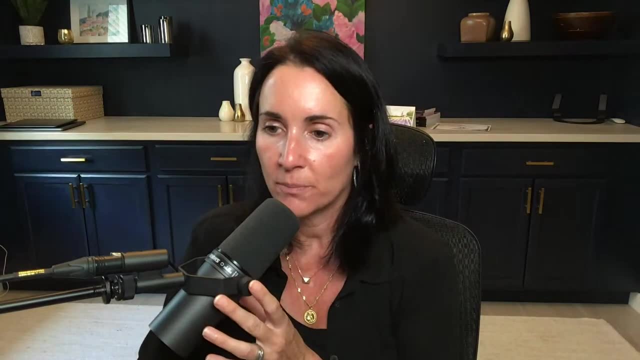 scratching the surface here, you guys. It's a, it's a, it's a huge exam, So there's going to be a lot more there. uh, for the five Oh two and the five Oh three portions, Will there be fill in the blank questions? I don't think there are fill in the blank questions. 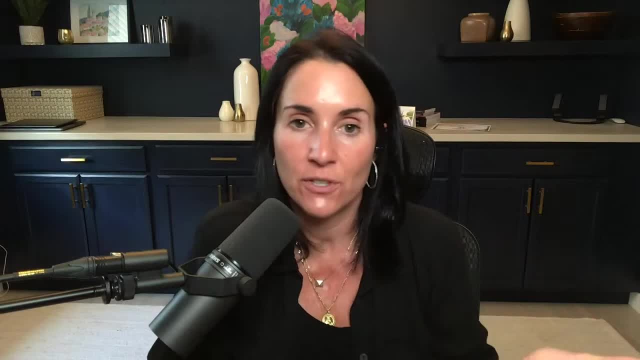 but again you could get it. I don't know. I mean they could do a fill in the blank question. Try not to focus too much on that. You don't know what questions you're going to get, So you've got. 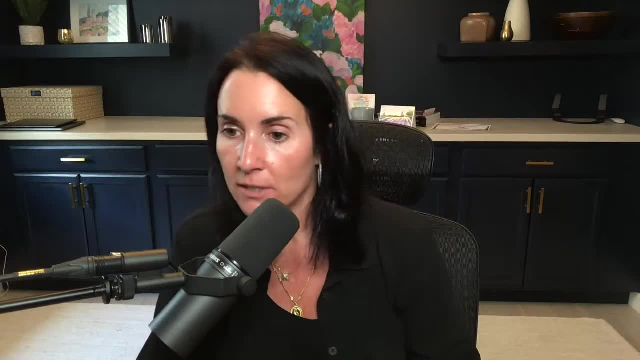 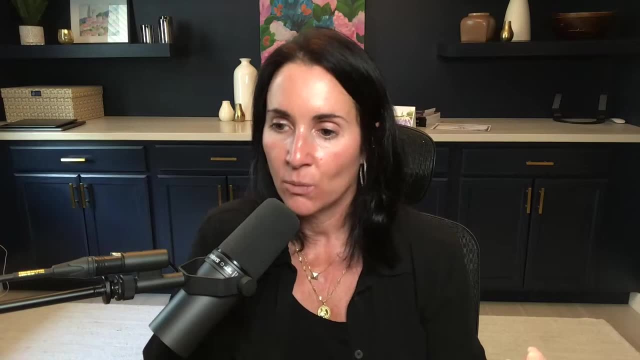 to understand that information really good. Uh, Jimmy Khan Wilson, life science is my favorite too. Thank you for all the help and resources. Very informative, Awesome. Will this study guide assist with the case six exam? Listen, I don't do uh, FTC. 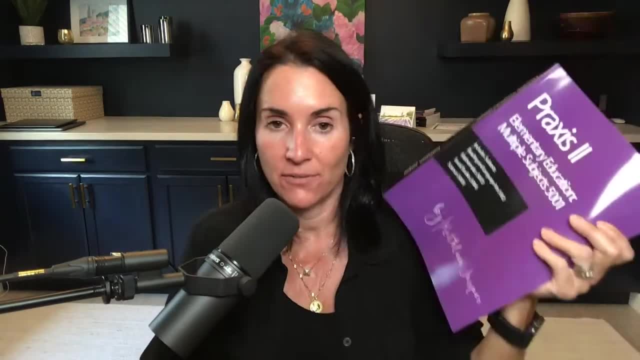 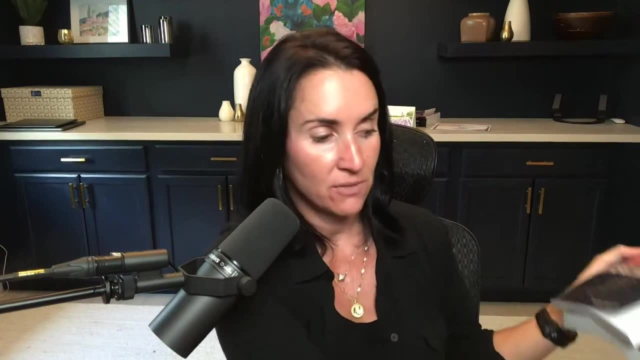 This is for the praxis Okay, But it will help you with lots of different elementary ed exams. Thank you for all your help. What else can you recommend for the foundations of reading? The thing that I recommend for the foundations of reading is this praxis: my praxis um teaching. 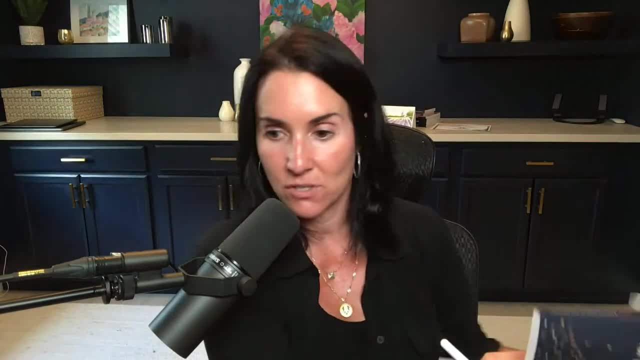 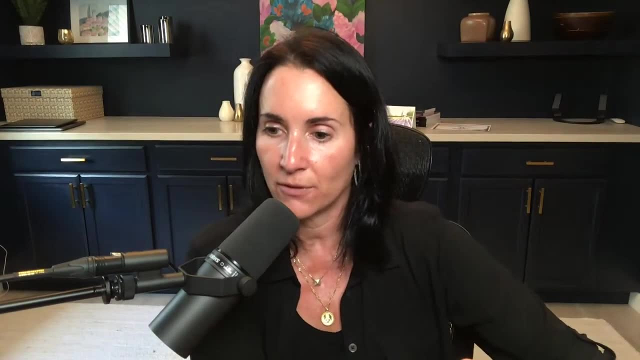 reading book. You can get that on my website. It covers all the same stuff. Latrice, for the online course. What are the costs for those, please, And do you offer a discount? Yes, The discount code I just put in the chat. It's praxis. 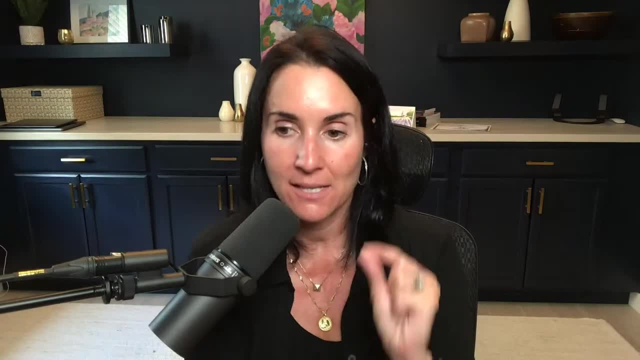 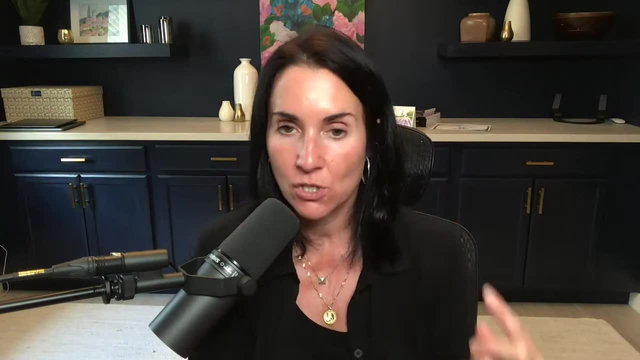 So praxis, the name of your test, EE as an elementary education, 20.. And I'm going to send that out in an email in about an hour, So you'll be able to do that. So just go to the um website. 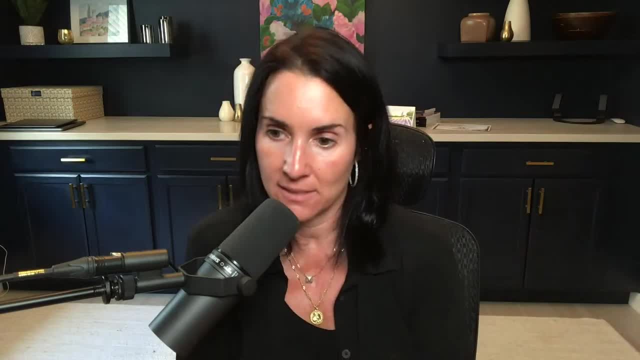 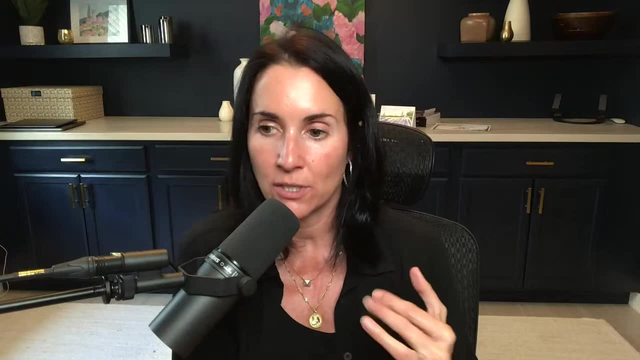 You got to go all the way to checkout and you can enter that discount code. How long does it take for the scores to come in? Are they online or mailed? Alex D, good question, All right, So you're you. most of the time, you get an immediate score for each section. You'll see it pop up on. 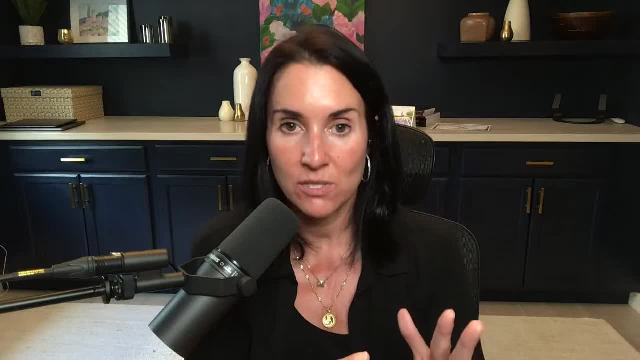 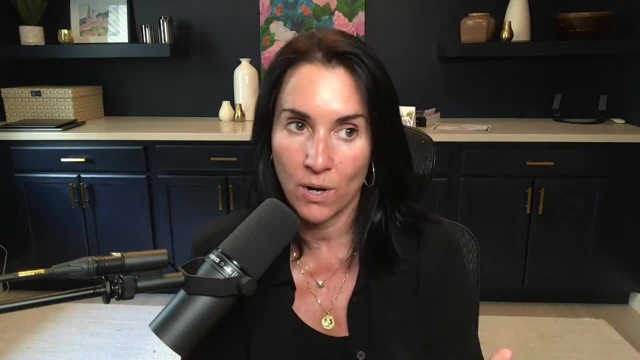 the screen. Be careful. Sometimes you miss it. So you'll see a score pop up on the screen Now- not always. if they're, you know, in the test working on some items, things like that- they won't give you a score right away And then a few weeks later you'll get it in an email. Now, 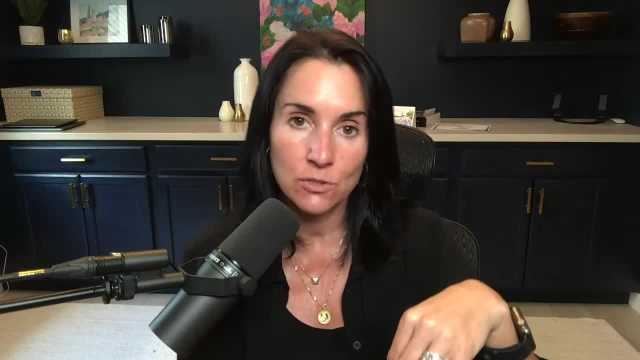 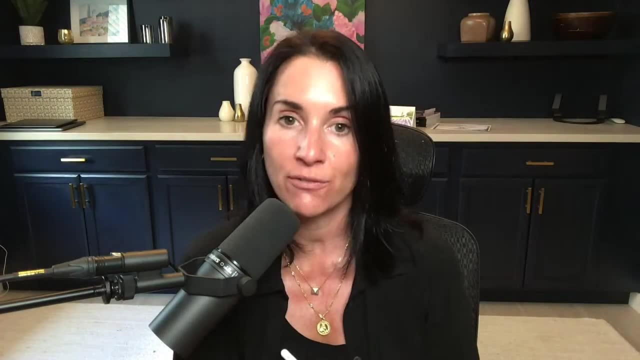 people will say: does your um online score match your official score? Typically, if you have a passing score on the screen when you're done, that is going to translate to your official score. It's very rare that your official score does not match your unofficial score. 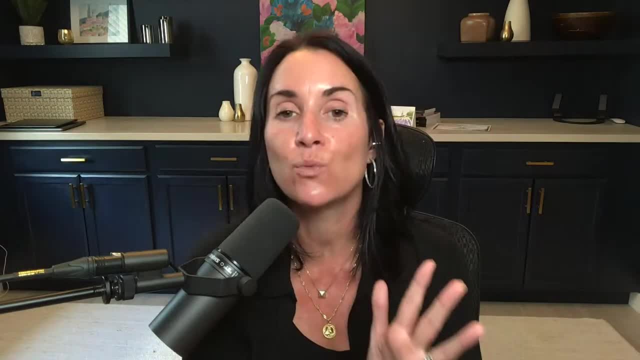 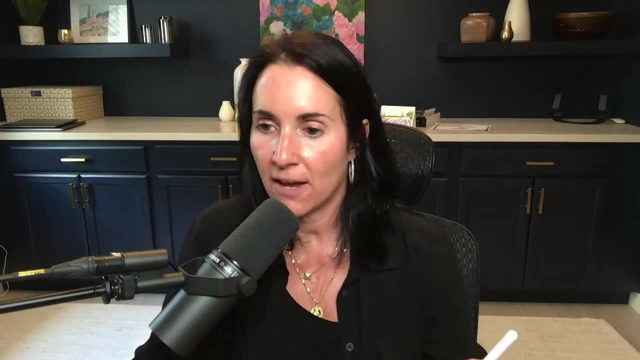 The unofficial score is the one that pops on the screen. but it could. but it's rare. All right, Um Praxis EE20.. Yes, that is the offer code. Do you have anything for the 5543?? Oh yeah. 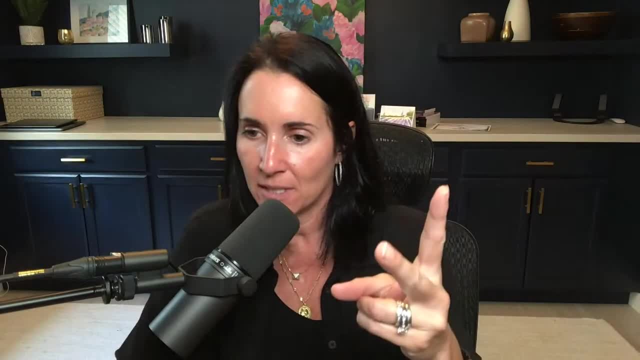 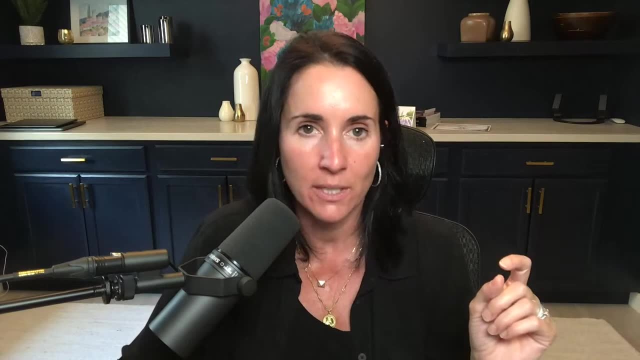 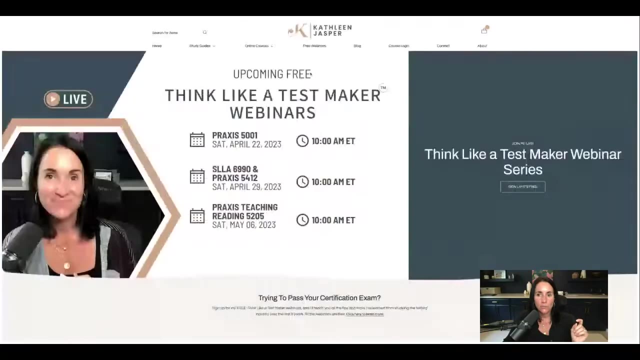 guys, let's have a look at my products here, Okay, Cause somebody is asking about the PLT K6, um all of that. So let me just do a quick little share on my products really quickly, Cause some of you are looking for more stuff. All right, So on this homepage you can see. 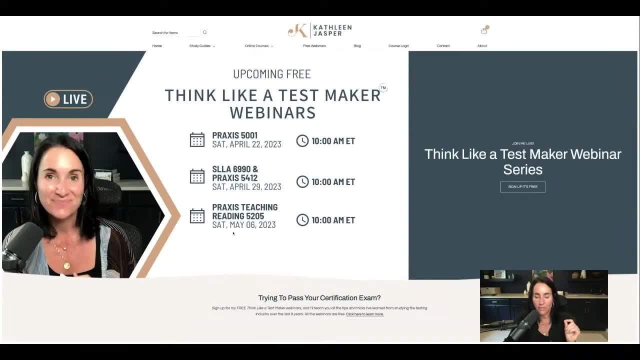 I've got my new webinars coming up, So if you need the Praxis teaching reading or the um, the Pearson 190 or any teaching reading exam, the Texas um uh teaching reading exam you're going to want to come to this May 6th. We're doing all just teaching reading And if 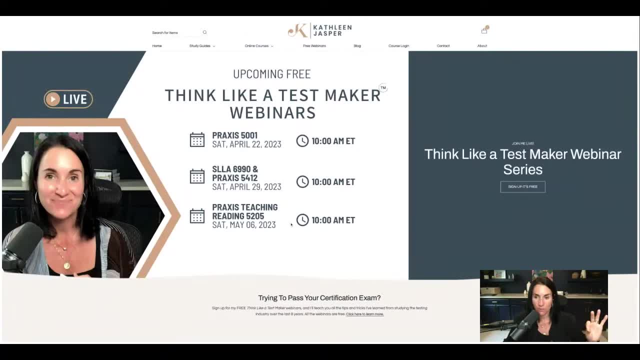 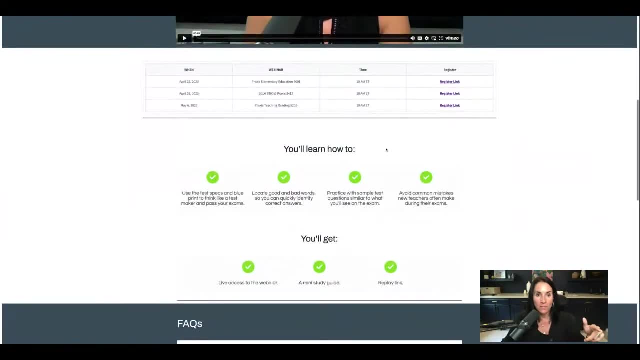 you're struggling on the 5002,. this May 6th webinar is going to be great. You just click here and it'll take you to the page with all the different webinars on it. Okay, Now for all my different study guides. 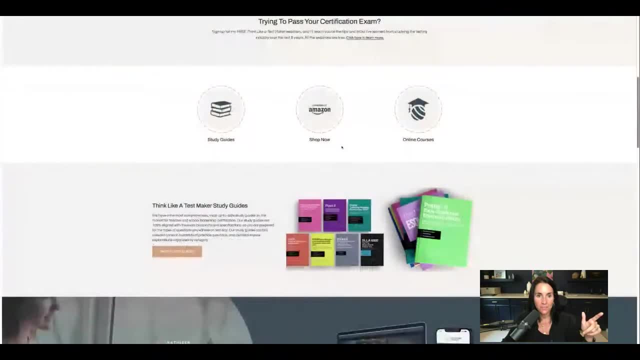 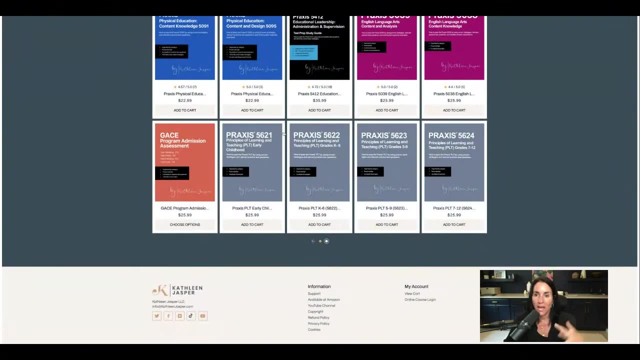 let me just go to my study guide page. Hang on, please hold study guides, Look at all of them, And I've got more. Now some of you are asking about the PLT. I know that test so well. I wrote an. 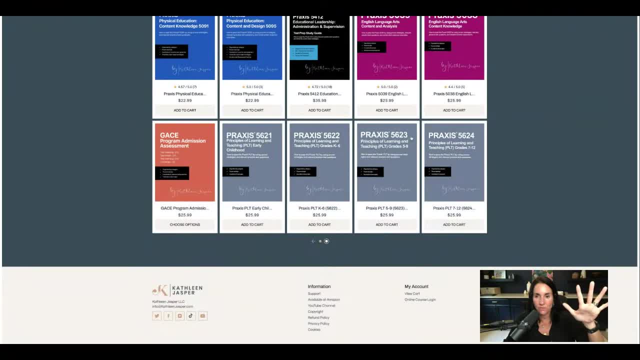 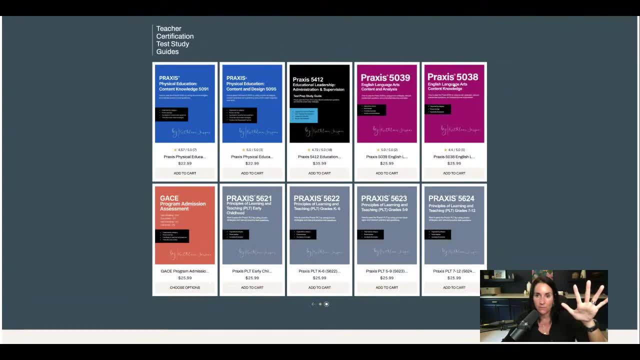 amazing guide for it. I have the 5622.. I have the 5621,, 5623, and 5624,. all grade levels, All right For high school. I have the ELA. This is the 5039 and the 5038.. 5039 has writing. 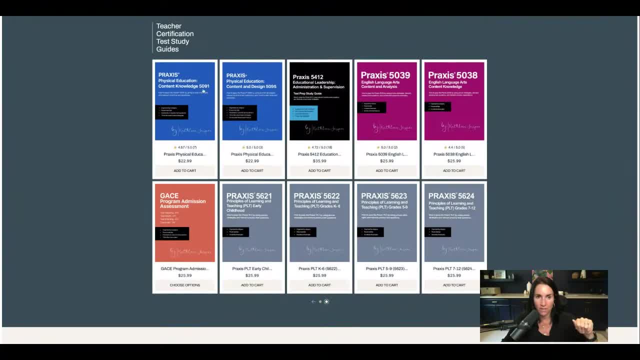 5038 does not. I've got physical education 5091, 5095.. 5095 has the writing. Same test. Don't buy two, It's the same test. I've got GACE. This is basically the same thing as the Praxis Core. I've 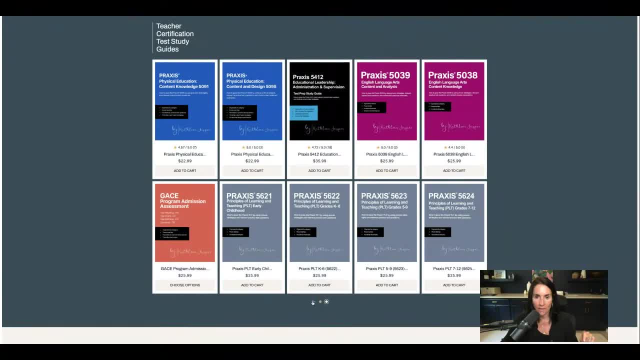 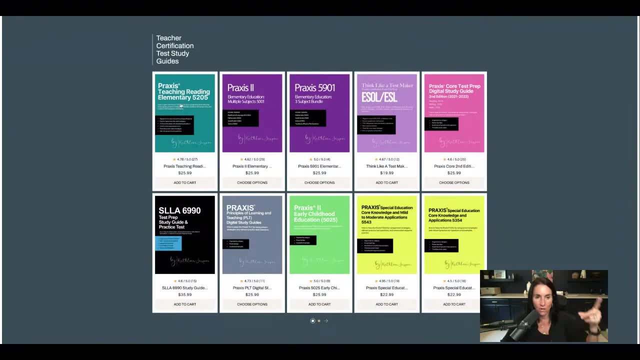 got leadership, Praxis 5402.. You may not be ready for that. And then these are our biggest sellers. We have the teaching reading elementary. This one's huge. You can use this for the star any teaching reading exam. Then 190, Praxis teaching reading. This is going to help you out. 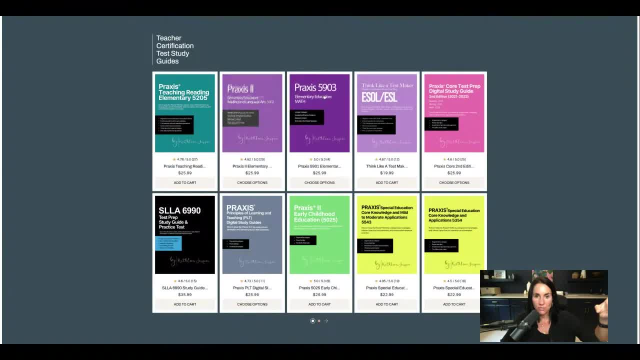 a lot. This is what we just used today: the elementary ed. These two are the same, These books, except this 5901. here it does not have the English language arts and reading People who take the 5901 have to take this. So you get the reading there. I've got ESOL that will help you with any. 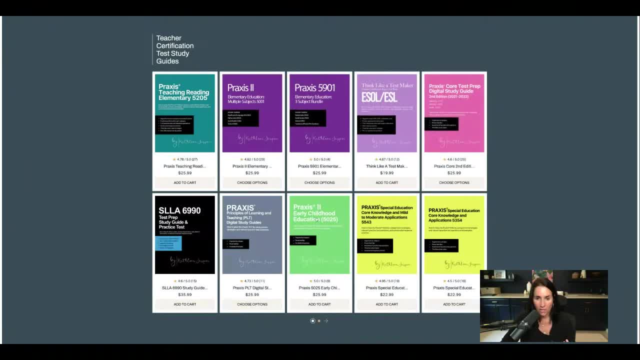 ESOL exam. I've got the core. Many of you have to take, that Early childhood. I've got a study guide and an online course for that, And the SLLA, when you're ready for leadership. And then I have the. 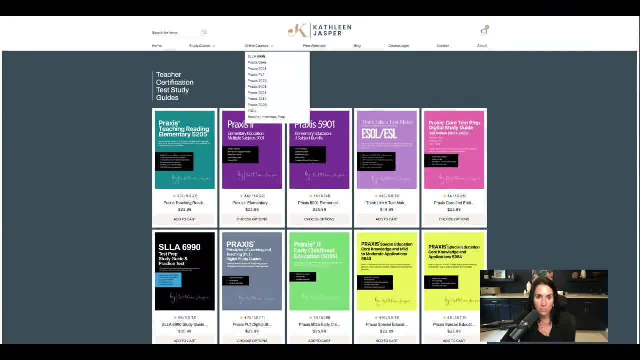 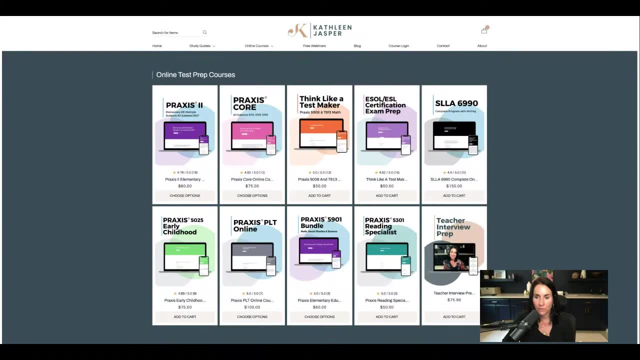 program, special education. Now also, if you go to online courses, let me go back to home so I can get you all the online courses. I have online courses for tons of it And I just did a new interview, teacher interview prep. That one is an online course and it comes with some templates and 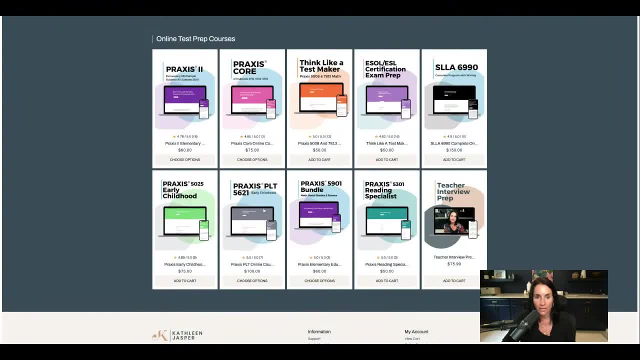 things like that, And so these are all my online courses. I have early childhood, I have all the different PLTs, I have bundles, ESOL, all of this- and I'm developing more. This one is for the 7813. 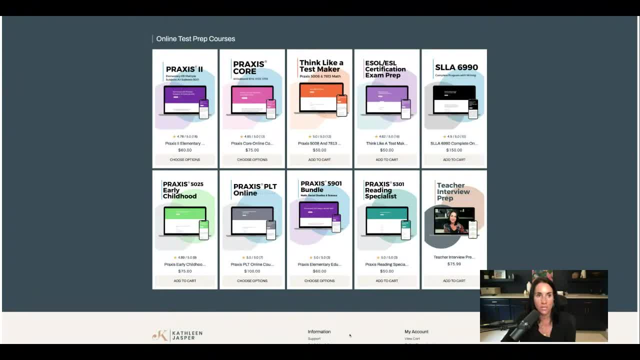 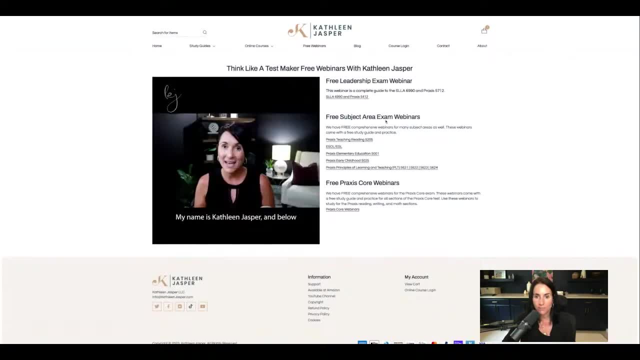 and the 5008 math. This comes with a study guide. They all come with study guides, All right, And then, finally, if you want some more free stuff, go to my free webinar, And I have all these different free webinars. I am updating that. So today I did the elementary. 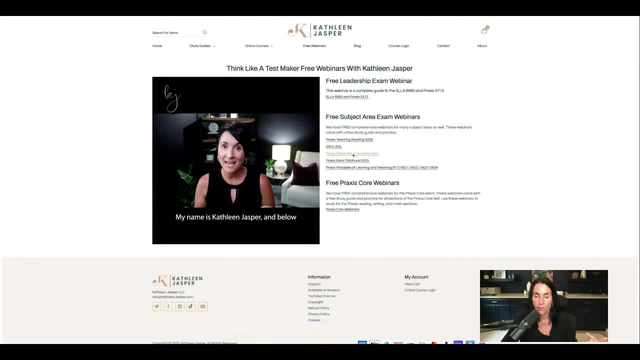 education. This is an old one, So if you want to do another one, you can do that one, And then this is the new one that will replace it. I'm doing SLLA and Praxis 5412 next week, next weekend. 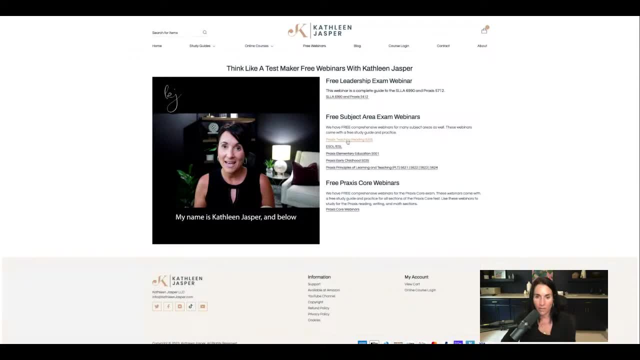 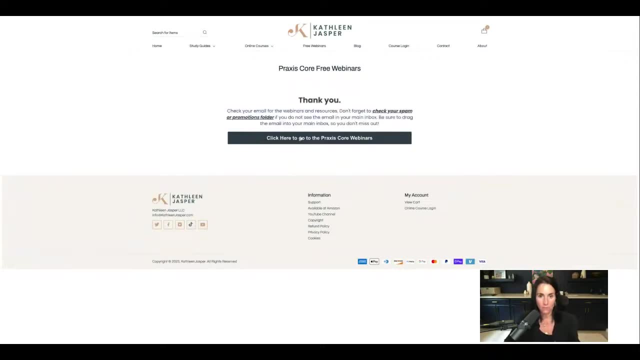 And then I'm doing a new teaching reading on May 6th. Okay, But I have these Praxis core webinars. Check this out. Check out how much stuff you get. Let me just go Here. you click here, You get a study plan, You get Praxis core. Look at all these videos. 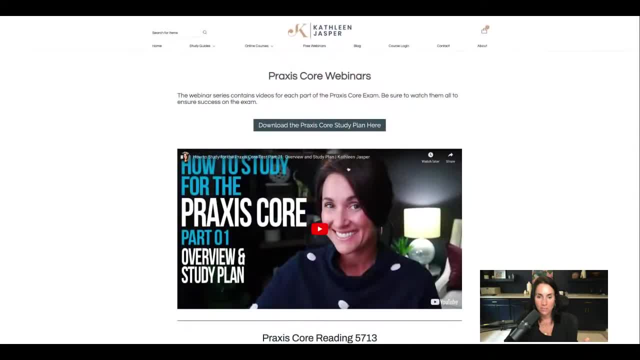 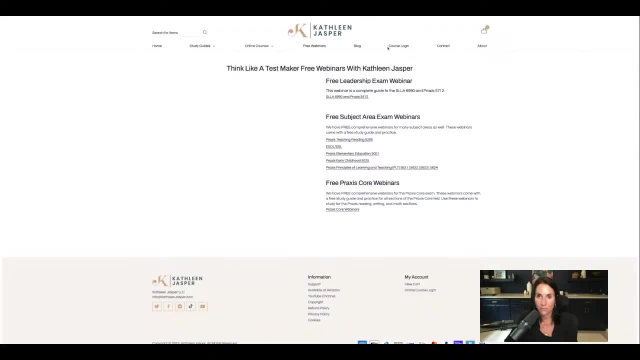 So, when you sign up for these webinars, you're going to get a study plan, You're going to get resources- These are study guides and all of that- And so the free stuff is really good. So make sure you check out the free stuff and, of course, the online courses- And we have a bunch. 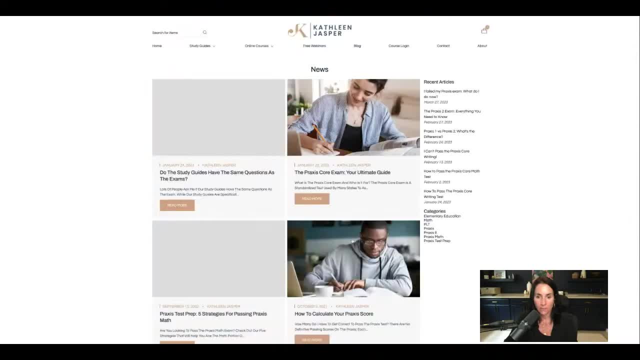 of new blogs out. This one's a really good one. how to calculate your Praxis score: This one will help calculate. some of you have questions on that, So I just have a bunch of resources there Now. Any questions on that? What? 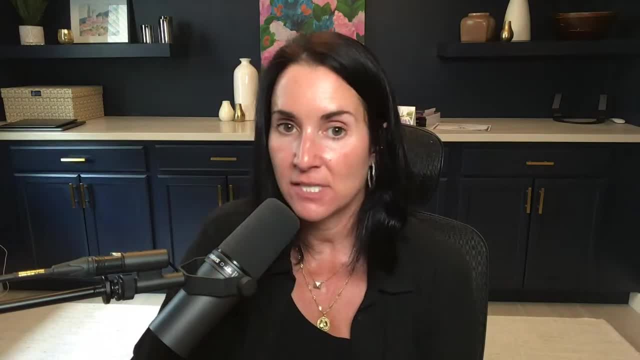 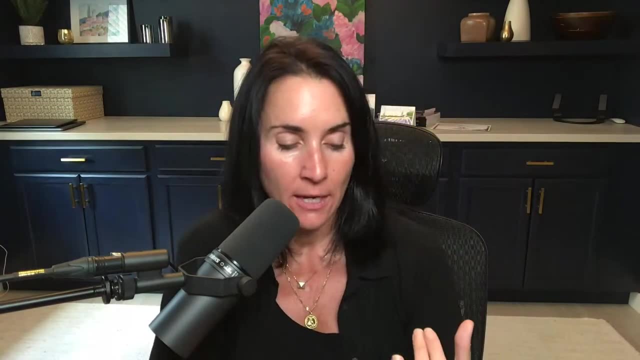 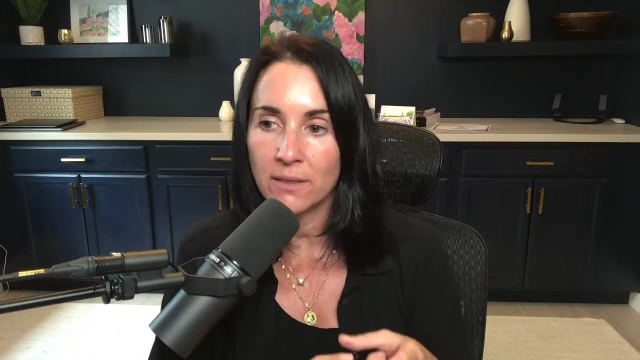 is the basic difference between the 5001 and the 5018?? The 5001 is all content driven, So like for the math and for the science and for the social social studies. it's just knowing those concepts with the 5018. It's teaching them. So you're going. 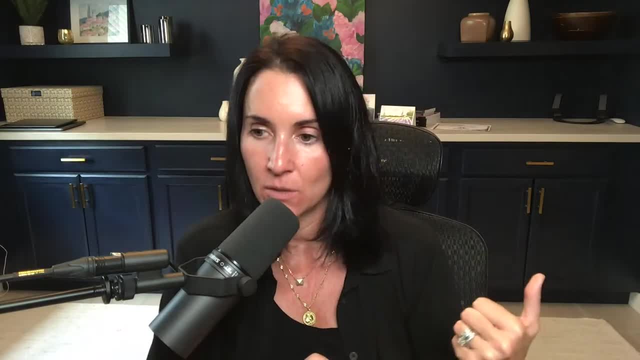 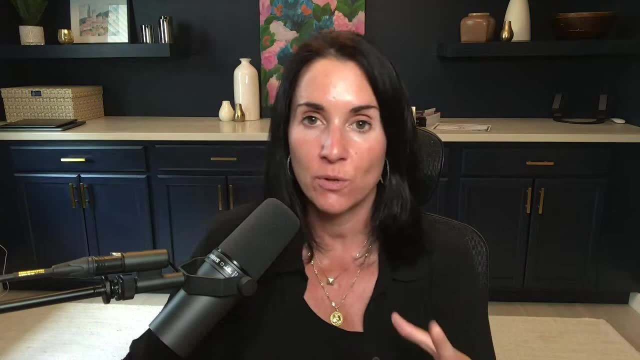 to have teaching scenarios rather than just straight up content. Will you have an online course for students with disabilities? Yes, I'm working for working on a course to go with my book, But if you need it now, let me show you. I have a. 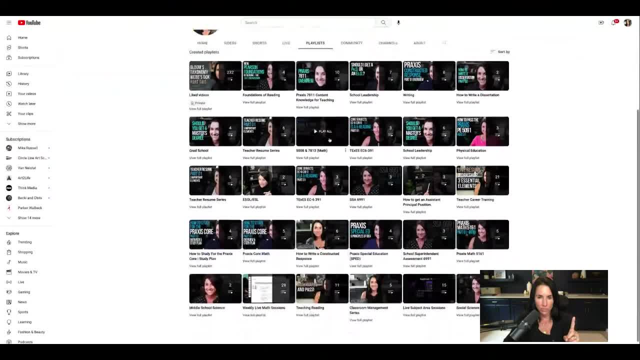 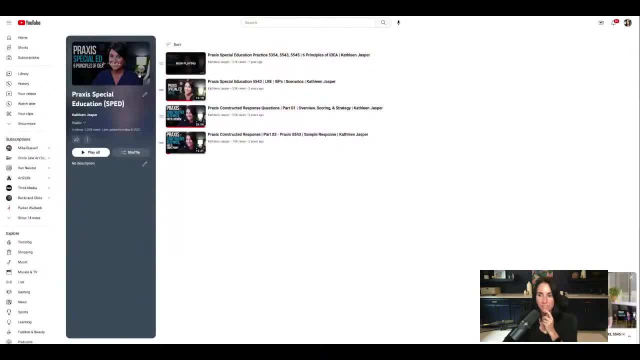 whole playlist for special ed on my YouTube channel right here. Let me go here. You can see that I have all of these videos here for practice special education. So on my YouTube channel you're going to see a lot of that, So make sure you be. 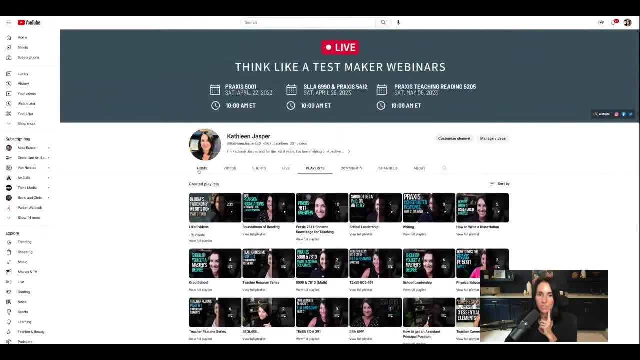 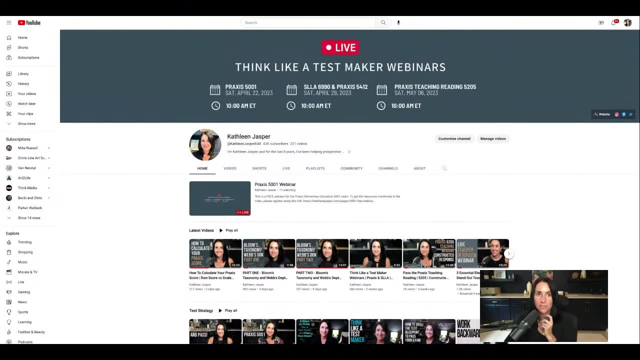 quiet. Kathleen Jasper, There we go. I would definitely check out my YouTube channel, subscribe and all of that. That will help you out there. Also, I have Tiktok. I'm doing a lot of stuff on Tiktok where I'm doing shorter videos like this one's on: 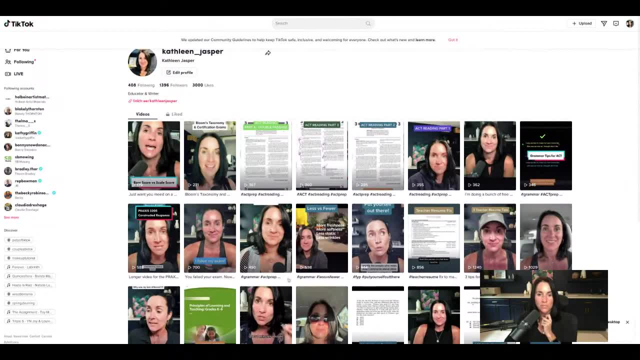 blooms. I do some ACT Grammar tips. I'm trying some different stuff, shorter versions here, And then, of course, my Facebook page here And this will all help you. you know joining the Facebook page If you go into groups. I have a group for teacher certification. 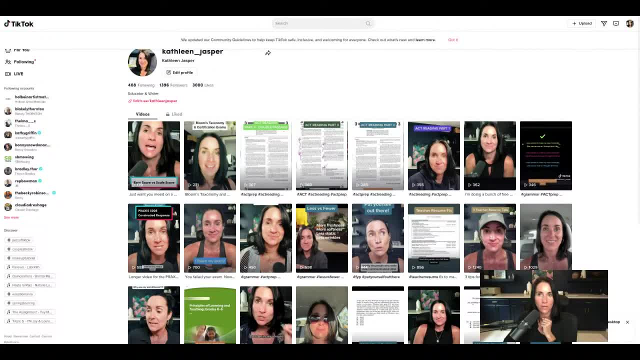 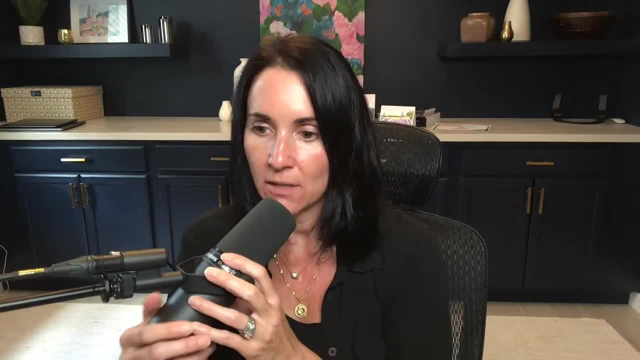 exams, leadership and, to go with my new book, teach, a survival guide for new educators. So definitely check that out. All right, So we're coming to the end. Will you have a webinar for the 5543 practice? Yes, I'm going to do one right now. I'm 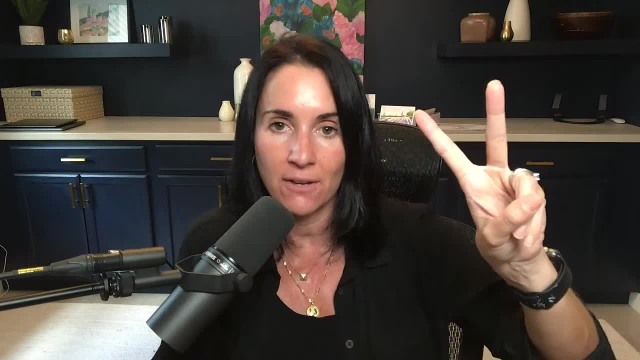 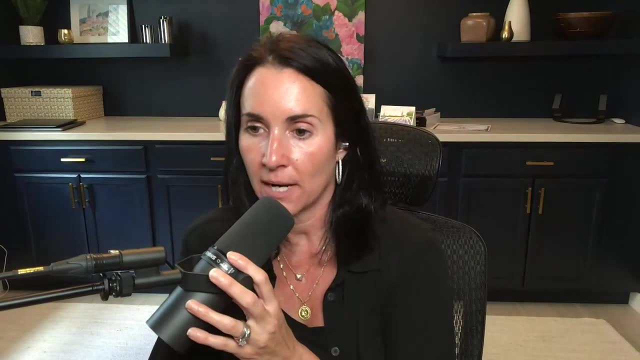 focusing on these three: the 5001, the SLLA and the 5412.. And then the following week will be the 5205, the teaching reading. But yes, I will definitely check that out, Chris Smith praxis. 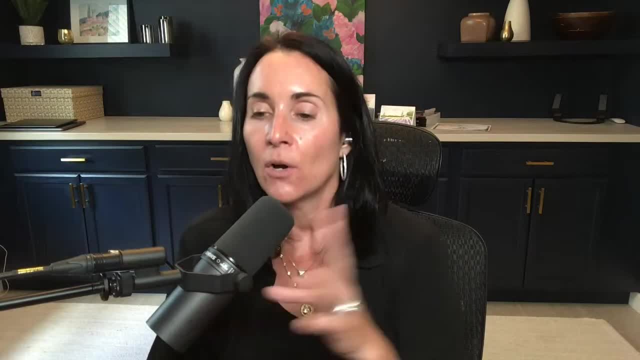 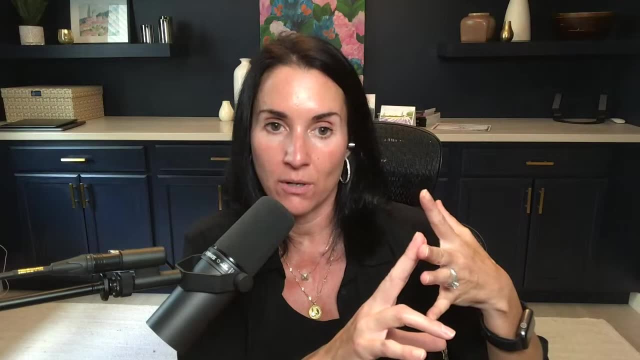 5001 and 5002.. Will it cover all sections? Okay, this is how it works. The 5001 is the full test. that has the 02,, the 03,, the 04 and the 05.. The 5002 is just English language arts. So if 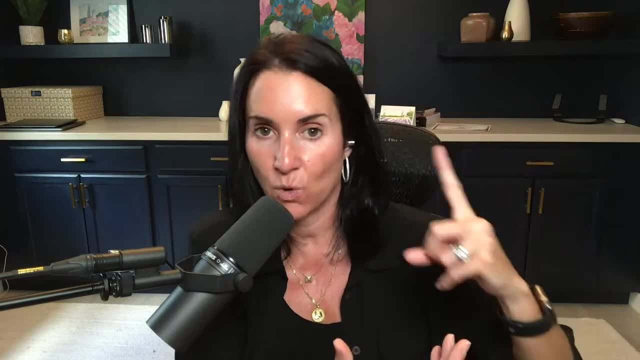 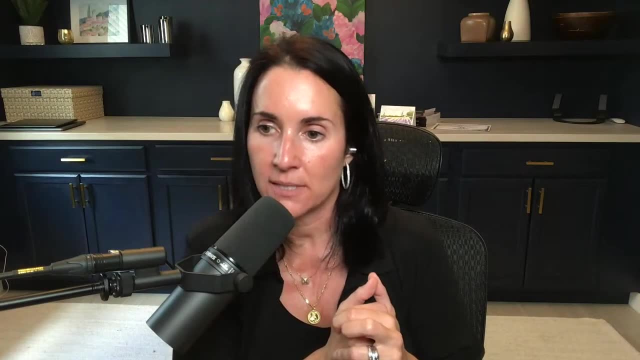 you need all of them. you got to buy the whole thing. If you're just need to pass one, then you can buy individual subtests. Okay, teaching mentally challenged children- anything for this class. I've been subbing a lot For teaching students with. 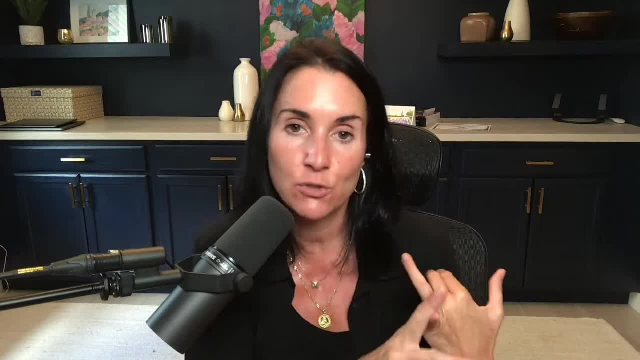 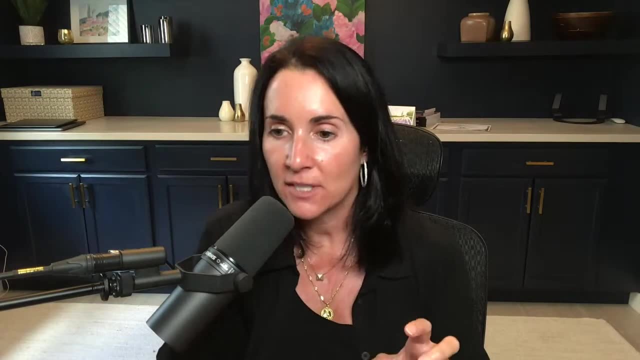 disabilities. you can definitely check out my special education playlist on YouTube and the resources on my website, Dr Jasper. thank you so much. Thank you so much, Cecilia. I already have a webinar for the 5025.. Go under free webinars on my. 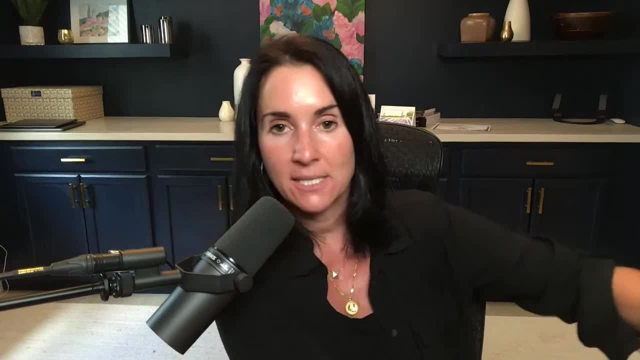 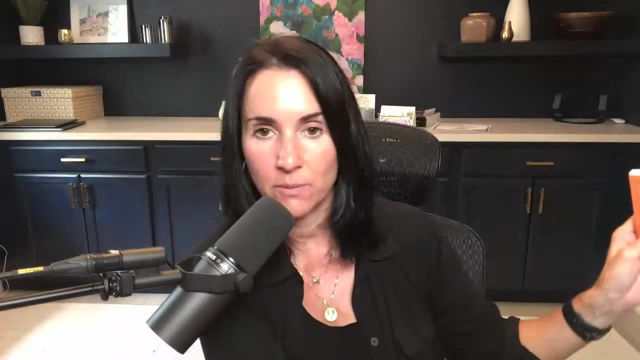 website. It's there. What about the science of teaching reading? Yes, this book will help you with the STR. Okay, it'll help you with any teaching reading exam. Lots of people pass using that book. I specialize in secondary education with no prior elementary skills, but want to. 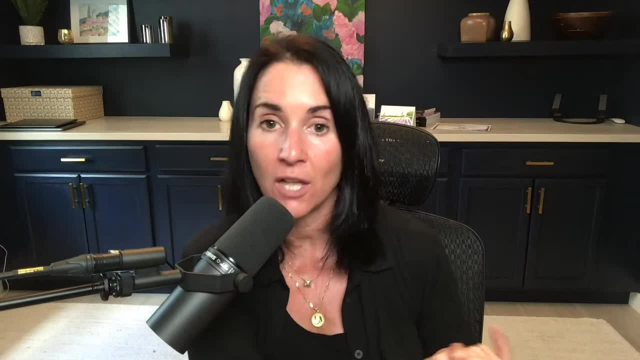 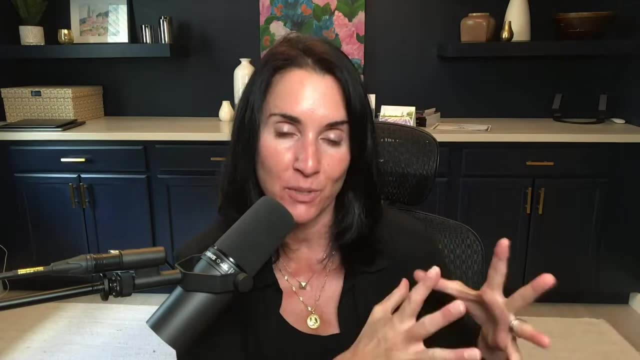 teach elementary. Will this book help without me doing another four years in college? The book will definitely help, But you know it's hard to put it all in one book. But the book will definitely help. a lot of people use the books to kind of teach.